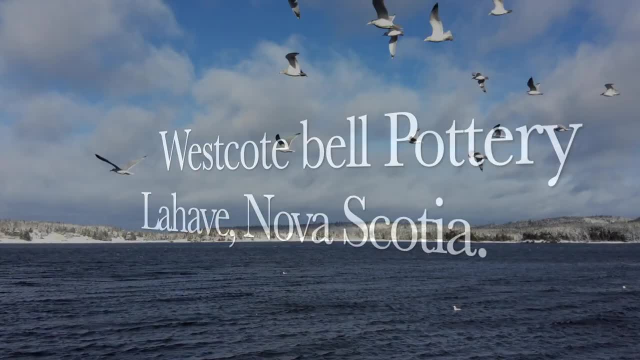 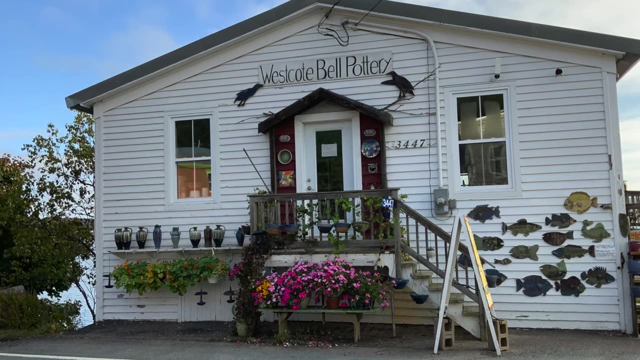 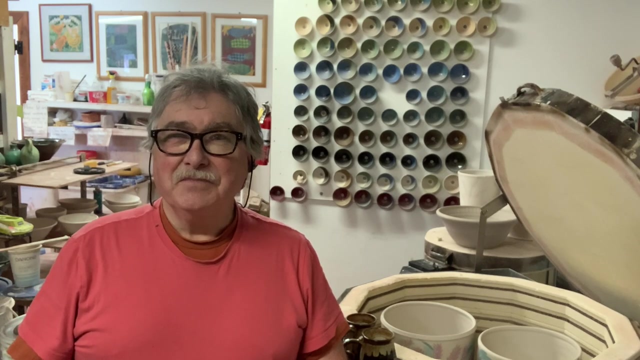 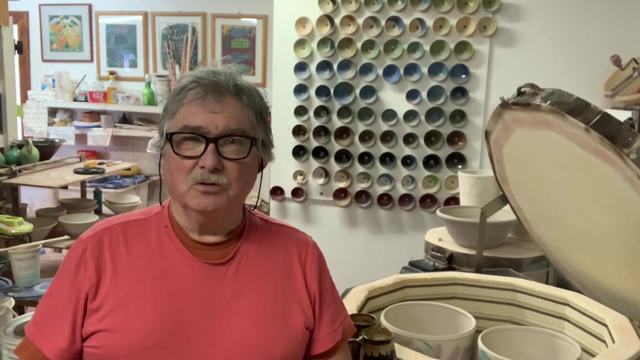 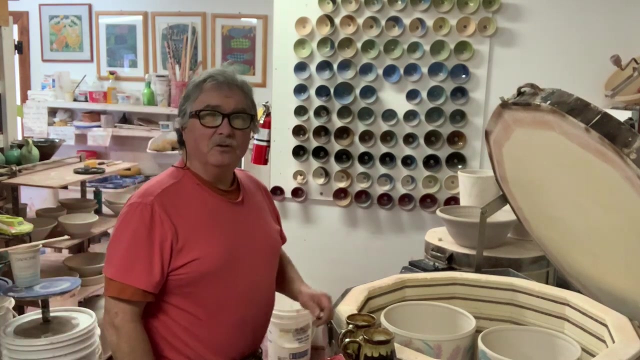 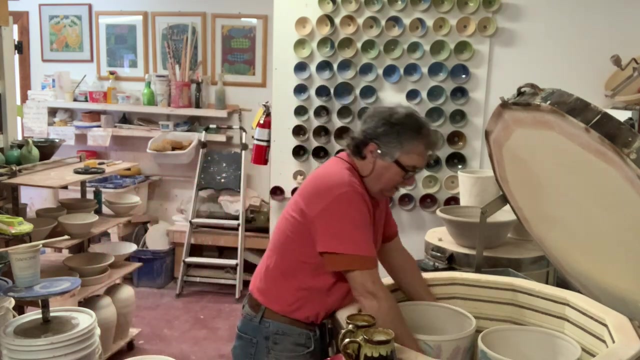 Hi, born in Nova Scotia at West Goatbell Pottery. Two kilns are going to be unpacked now and maybe a third, but I think I'll decide what to do about the length of the video later. A quick tease: I decided to paint really elaborately some of those flower mugs that I had in a previous video a few weeks back, and so I spent some time really painting. 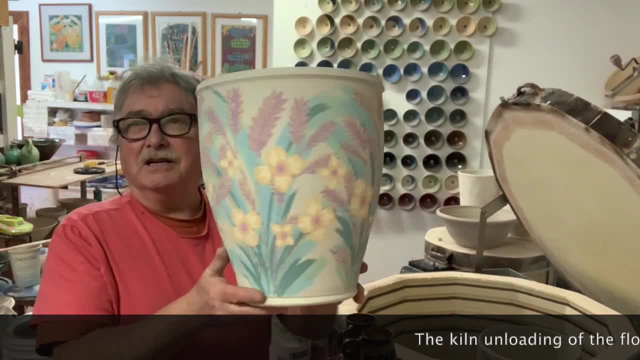 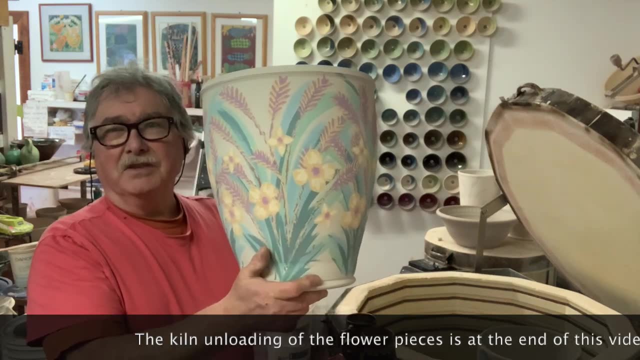 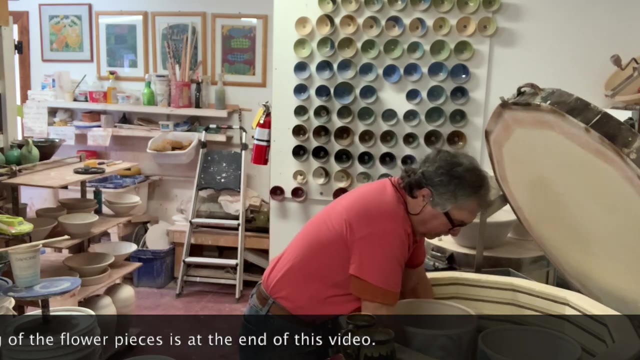 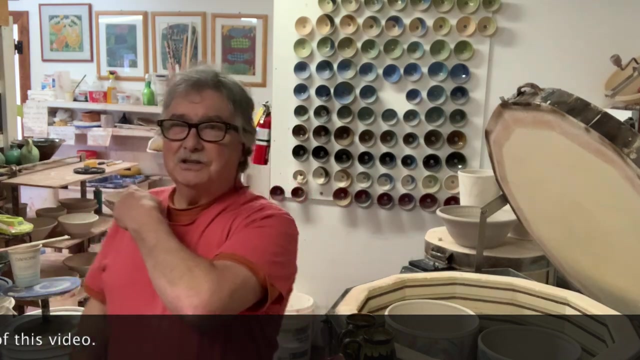 So here you go. this one is going through the kiln. it's a bisque firing. it's going in now, but this is an underglaze painting using those brushes that I showed you. So I'll have a whole bunch of these out of the kiln and I'll do a kiln unloading when I do it, because I've got lamps, large bowls, a whole bunch of things on that shelf back there and it'll be a really nice kiln unloading. 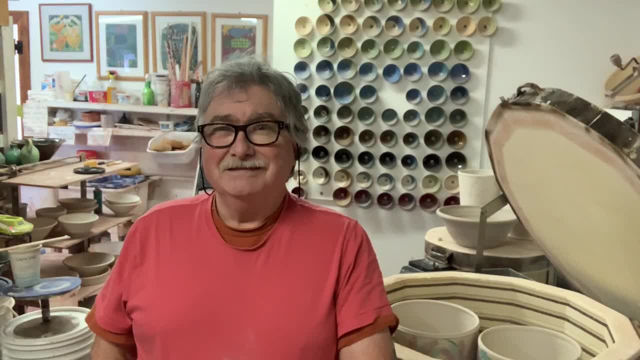 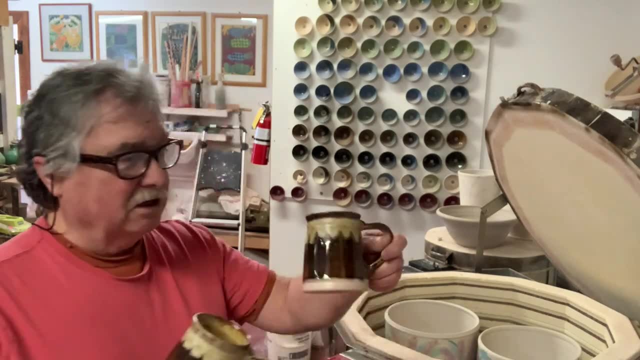 So basically, just hold tight, it'll be coming soon. Alright, so somebody wanted a mug with Tenriku gold. I can't find the email, so if somebody wants to re-email me about these mugs- they wanted a Tenriku gold mug- 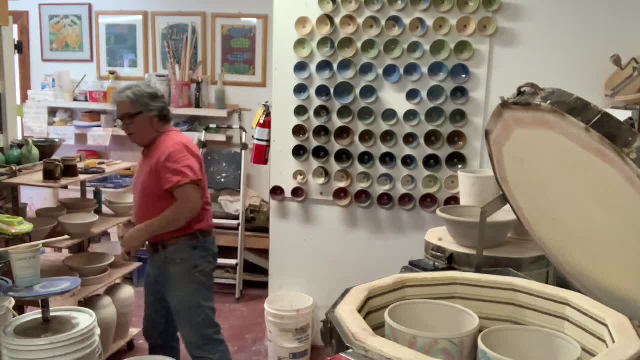 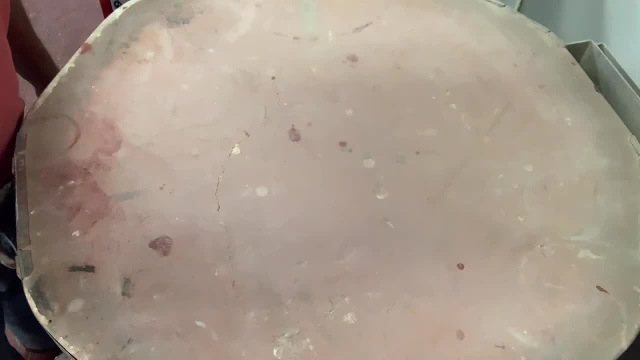 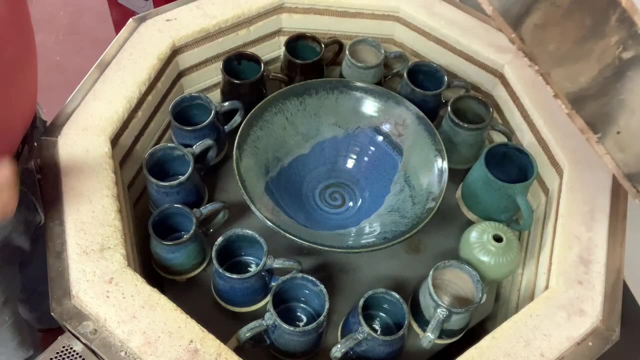 So, okay, let's tilt you down so you can see what's happening. These glazes are all from Mastering Cone 6 Glaze Book, and it's warm today, so I might be able to go outside and mix some more of my oatmeal, and when I do, I'm going to try two or three different recipes of oatmeal. 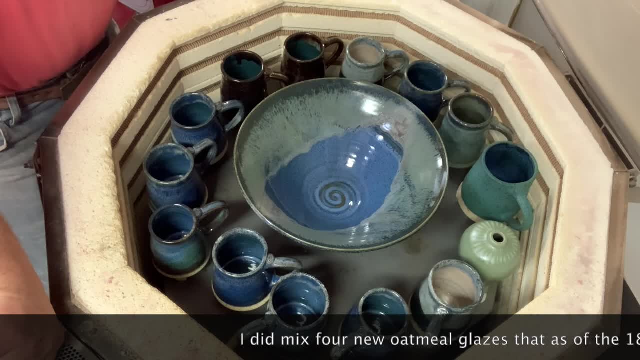 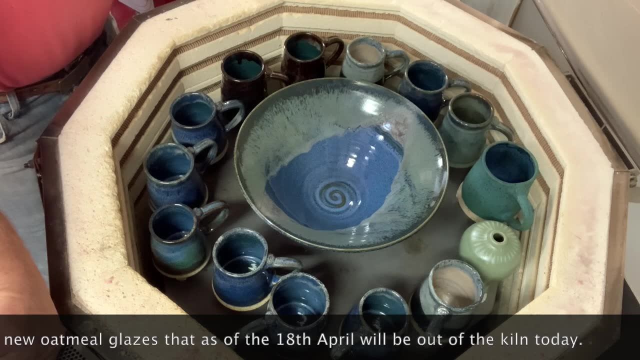 Because maybe I don't have the best one, but so I'm going to try doing that, especially since I have David Leach 2 recipe which I had in high school in the 1970s and it was a beautiful semi-matte white glaze. and I have to think if I add ilmenite and some iron ochre to that, it'll be a beautiful oatmeal. 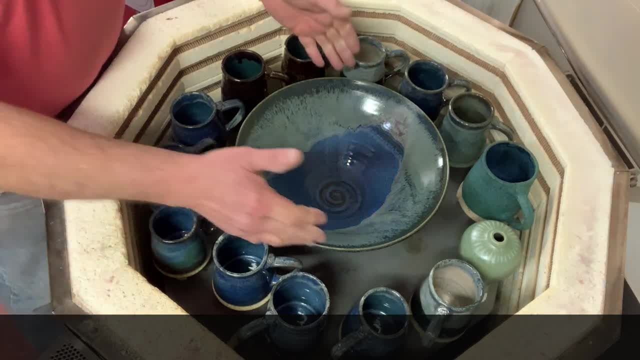 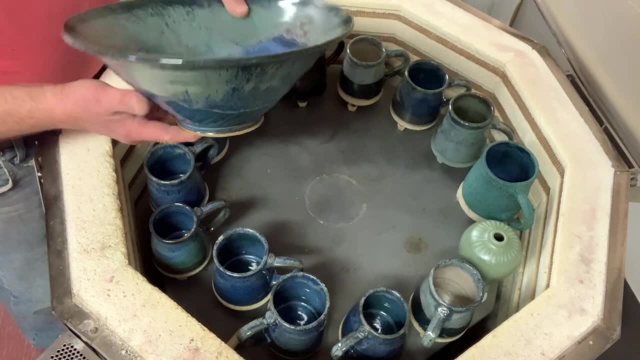 But it was Cone 8, so we'll see what it does at Cone 6.. Okay, so speckled clay, number 455.. From, uh, Pottery Supply House. I'll give you a look at that as well. 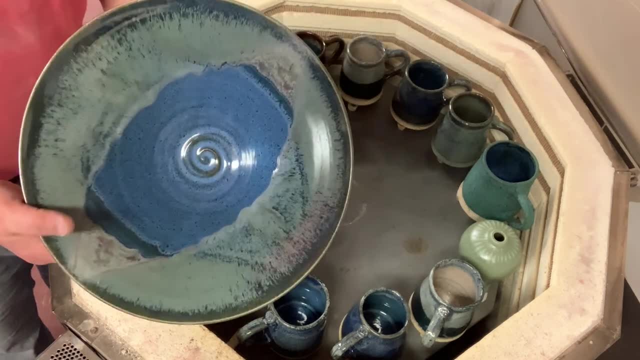 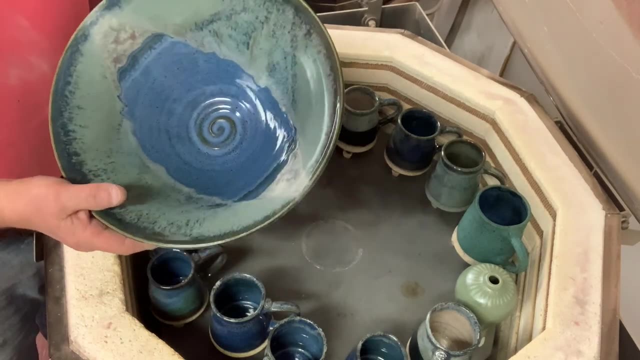 Speckled clay on the bottom there. So that's a nice ball. Let's see if I can tilt this a bit up so you can see a bit more, because when I angle them sometimes they go off the camera. But that's a really nice ball. 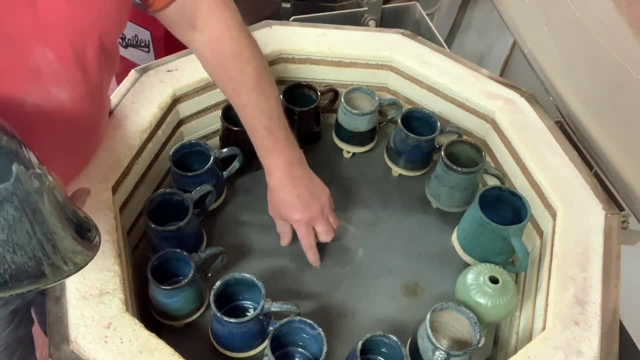 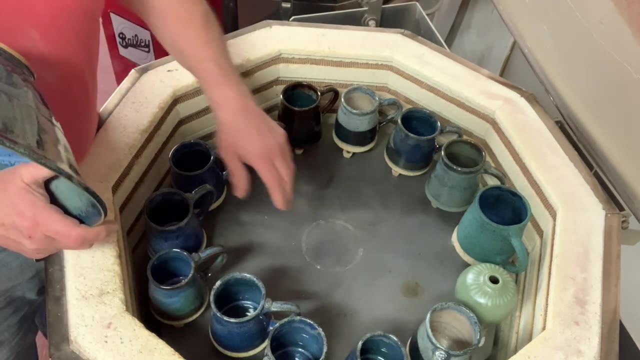 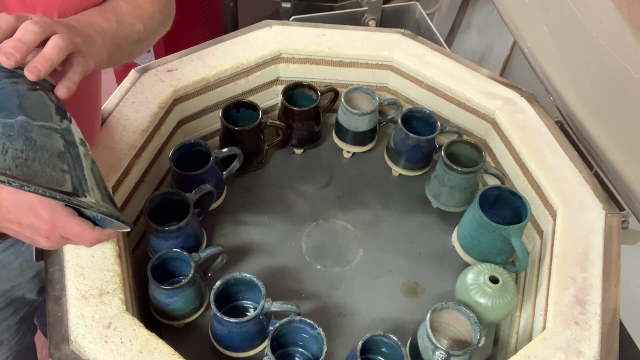 Speckled clay does not stick to the new shelves- although there's a little bit on there, And I talked to Jim Bailey and he recommends that you backwash these shelves If you're actually doing anything, Um, with porcelain-style clays- that means B-Mix 5, and any of those smooth white clays. um, what do we have in here? 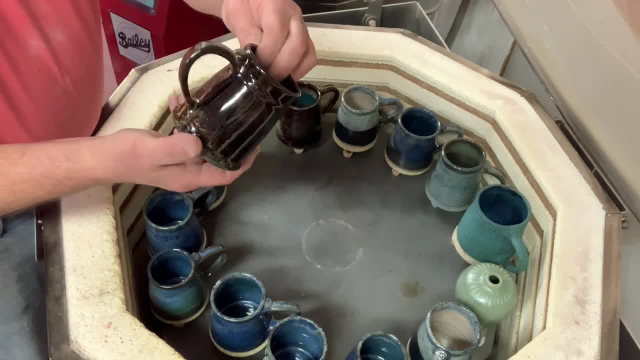 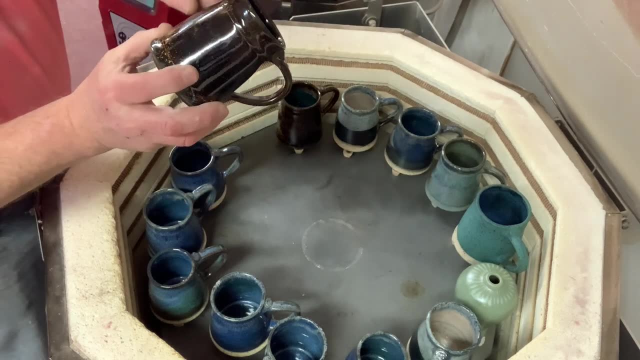 This one is a Tenmuku Gold, but it, the oatmeal, seems to have really mixed into that one um. so that's interesting. It didn't show up. they're usually just a bit on the top, but I'm not sure. maybe I didn't do that to that one. 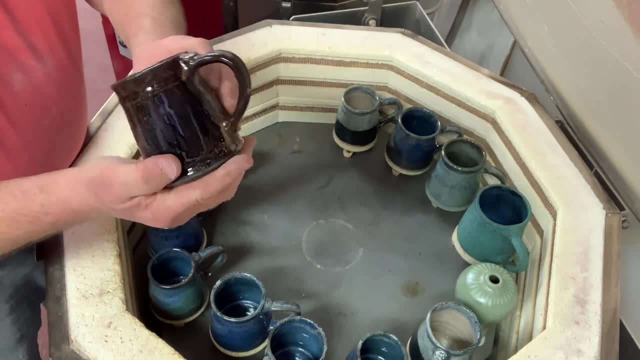 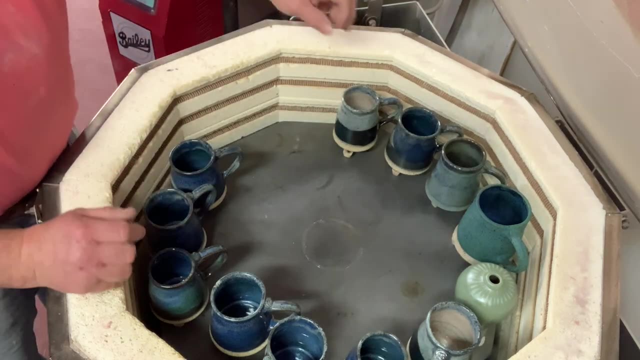 It's got blue on the bottom, Blue on the bottom, Blue on the bottom, Blue on the inside And then the oatmeal. I did fire this one back up to a little hotter so I might drop down to uh between cone 5 and 6 for the next firing. 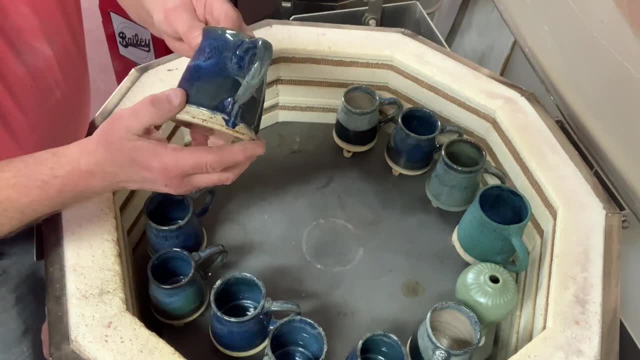 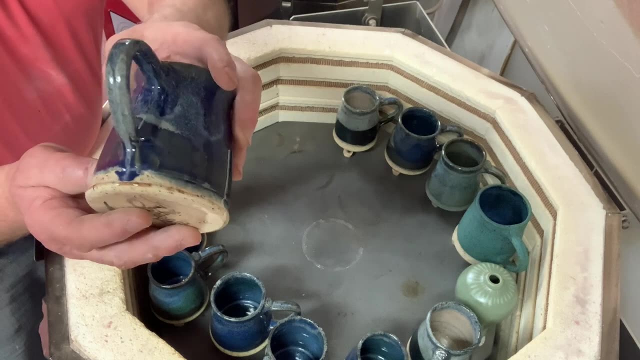 Everything looks good, um, but they run more obviously when you get a little hotter. So, oh, look at that, it always runs a little bit down the handle, But it didn't come off the bottom, so that's nice. 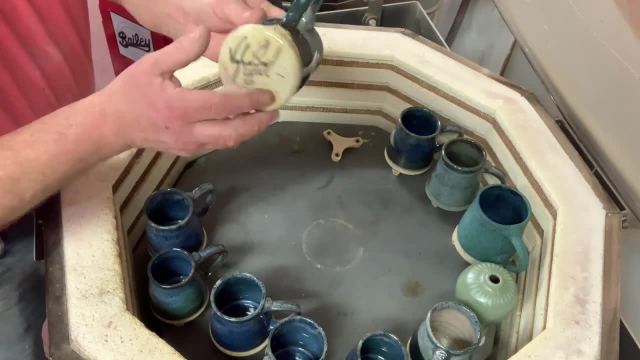 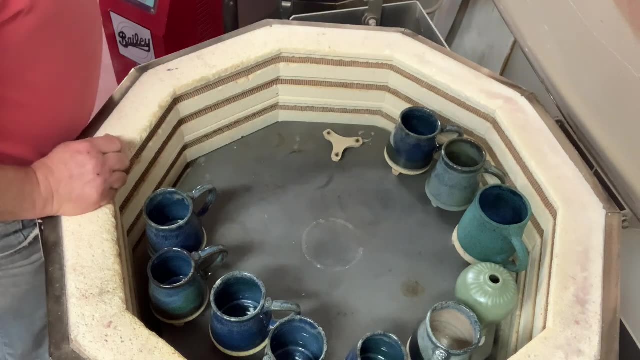 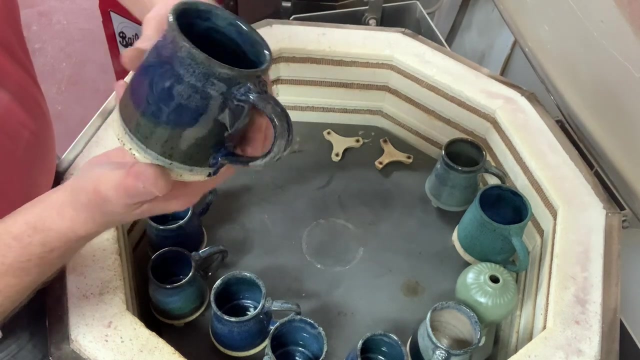 So hopefully the grinding issues are over. In that last kiln unloading I did re-fire all the pieces that were run running onto the bottom and they all flattened out. So that's a good use of stilts. This is all bright blue, dark blue and oatmeal on these pieces. 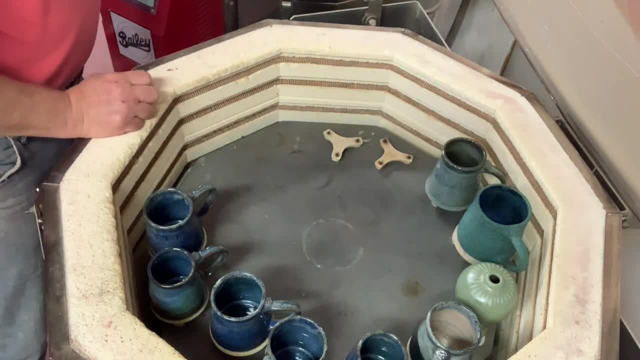 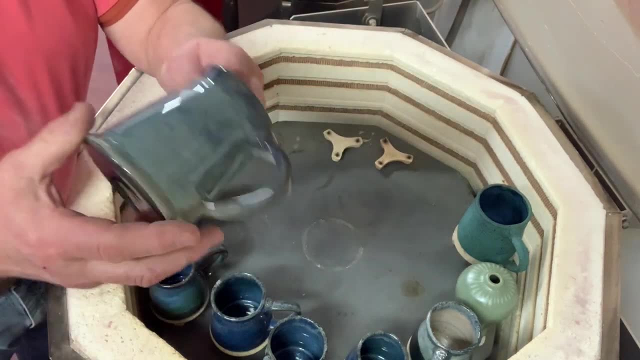 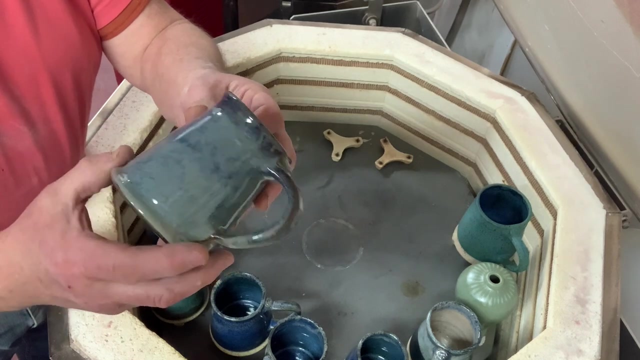 They'll run again, But not off the bottom. And here's the one that always runs. What did it do? Well, I got better with it, So I decided to dip a little less thickly on these, And I've maintained that kind of color, because it really has a nice flecking. 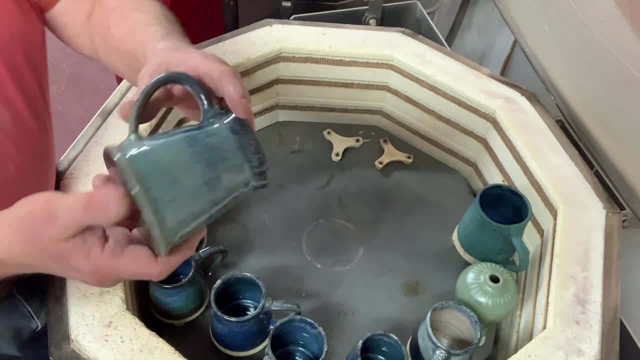 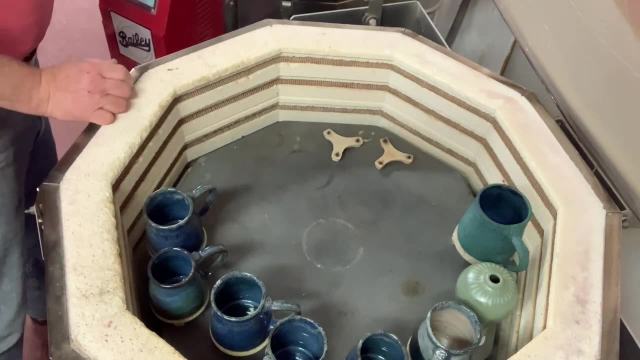 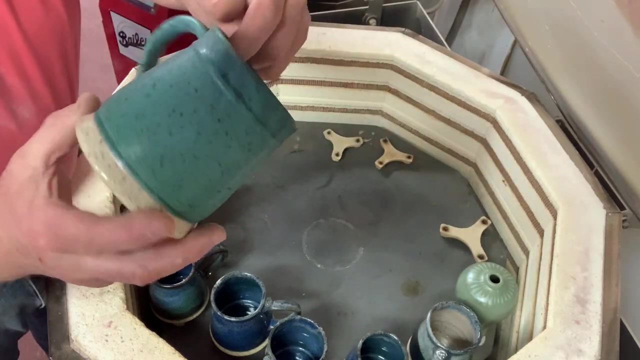 Um, so basically, um, that's where it always runs and sticks to the kiln shelf or the stilt, and this time it didn't. So it's just about tiling with this glaze, And this is the turquoise matte, which has done really well too. 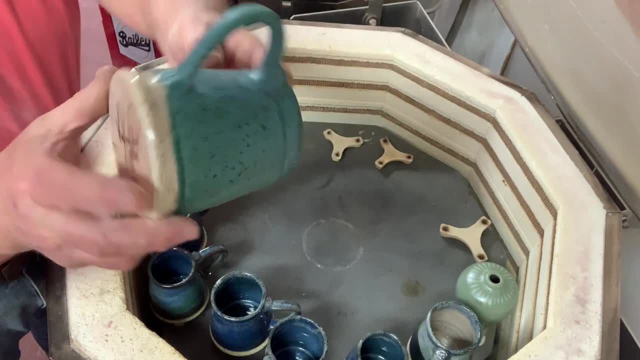 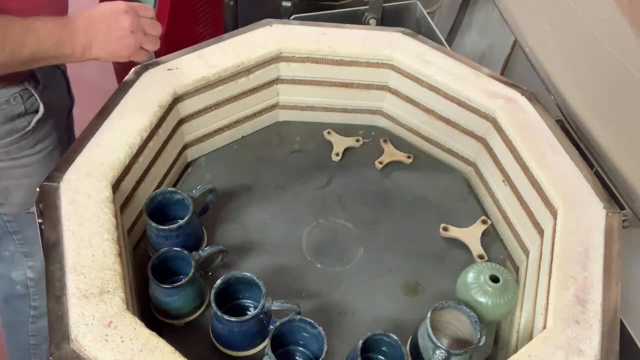 Oatmeal on the bottom, blue on the inside. No crack on this one. It's the seafoam that's been cracking for me. Um, and this one ran onto the shelf, so I'll have to grind that one. That's the green again. 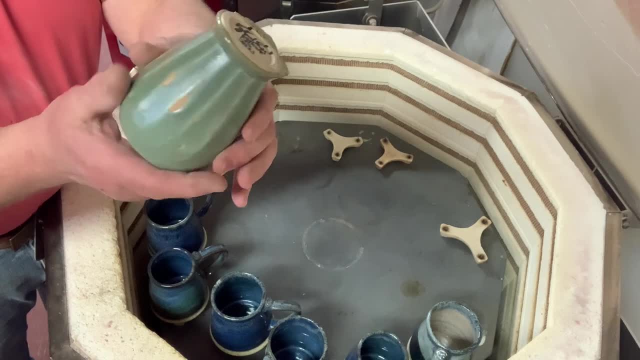 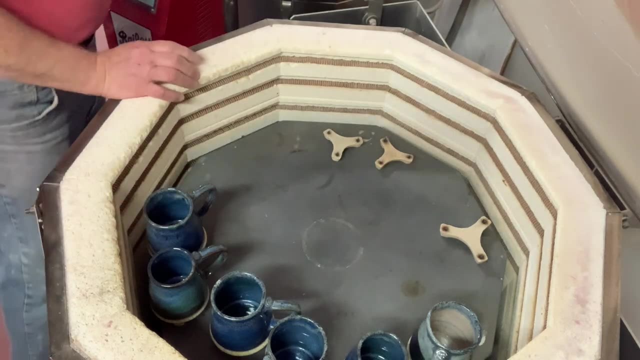 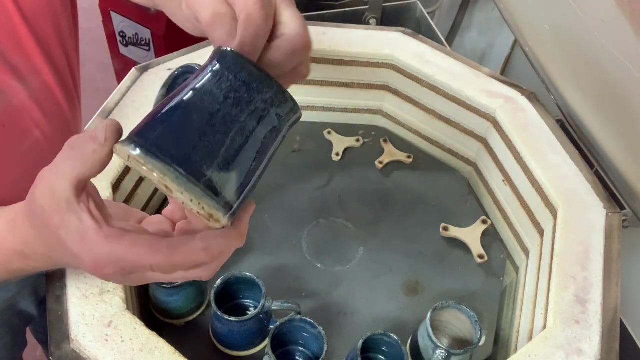 That's the one we are having issues with it running Um, so that one needs to be fired a little lower in temperature. But I can grind that one down easily. But the stilt-fired pieces? There's the dark blue with oatmeal over the top. 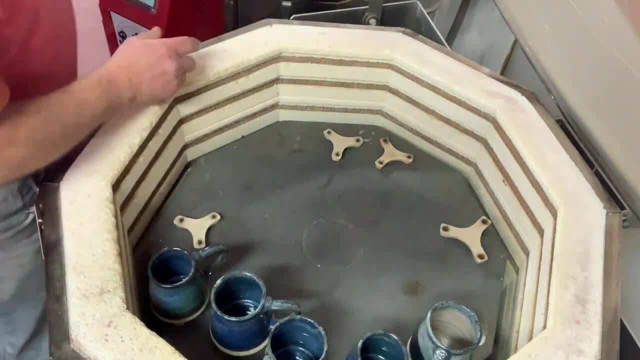 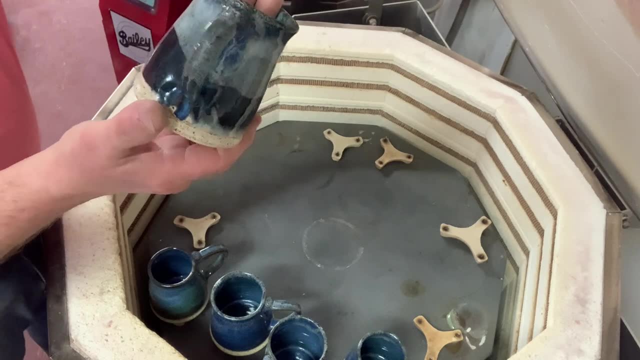 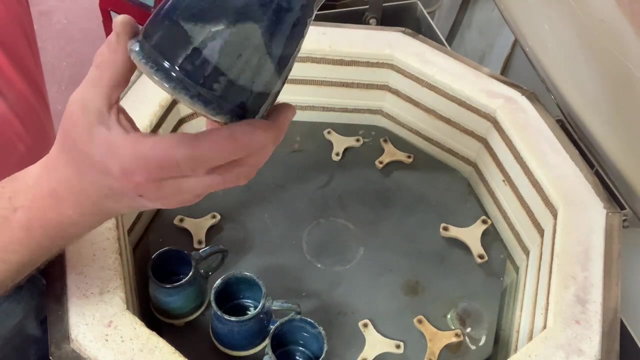 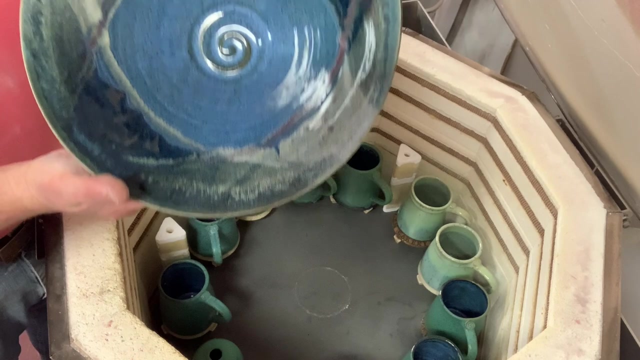 And then I dip my bright blue over that Dark blue again. I think seem to remember I packed this kiln mostly with the same pieces on each level And perfect, No running. So another one of those big blue bowls And it's in the speckle clay as well. 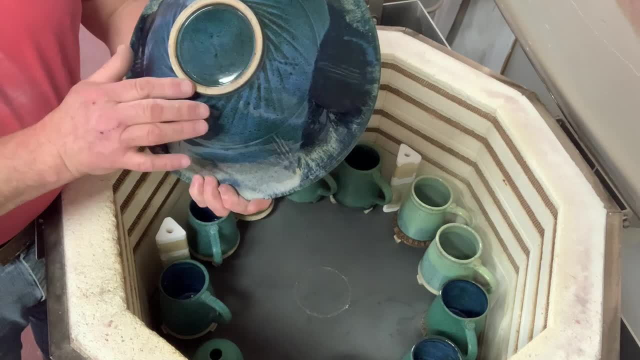 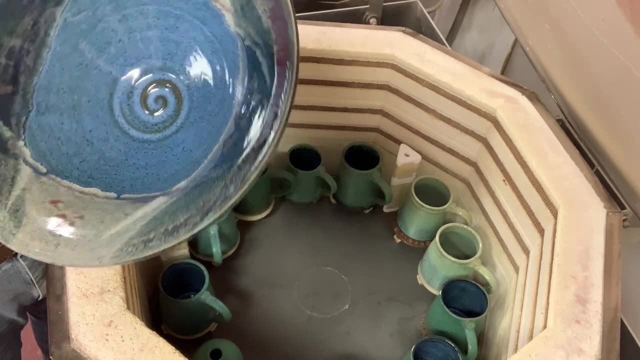 And there's a little ring on the bottom so it does need sanding a little bit on the bottom. So I think I'm going to bat-wash all these shelves- And that's what Jim Bailey told me to do, Because they don't warp at all. 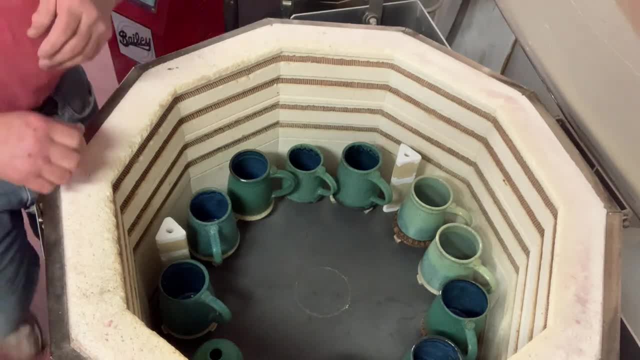 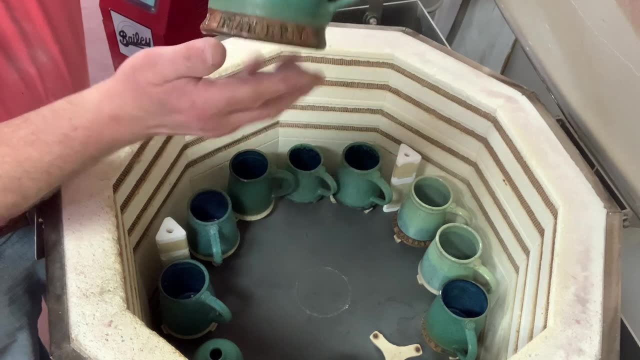 So you can bat-wash one side and you don't have to flip the shelves over. Okay, These look really nice. This is dark blue on the bottom. They're the ones I make for the bakery next door. We have a bakery next door that's called the Le Havre Bakery, if you check it out online. 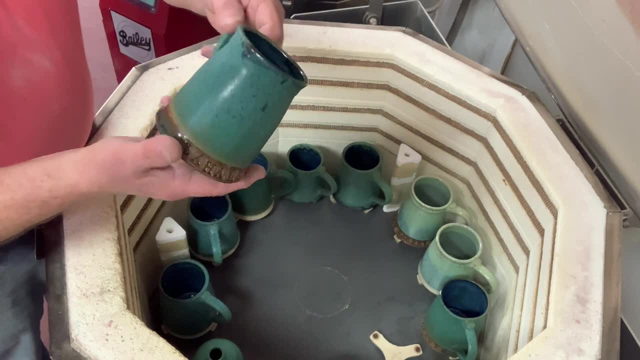 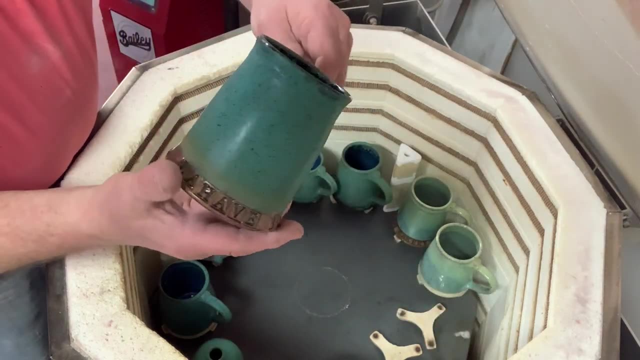 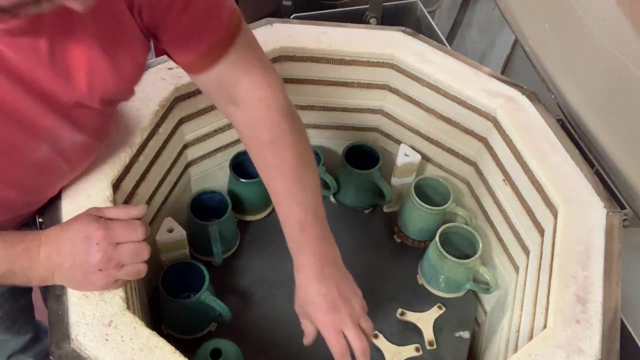 And on Facebook, I think we have a page too. That turned out very nice. So they're all Turfoys Matte, Turfoys matte, And it has a sheen to it, so it's slightly shiny And that is. 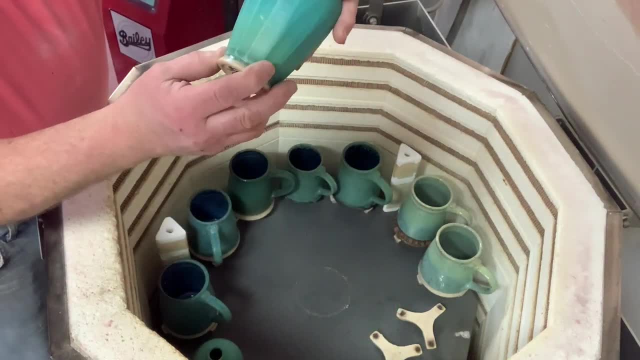 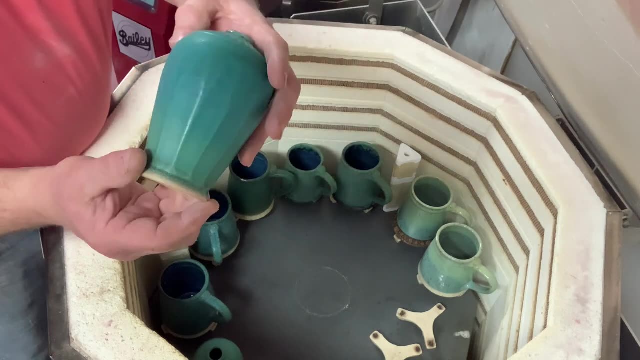 This one is seafoam And it didn't crack Interesting So, But it's very pretty. I'll tilt you down a little bit more so you can see a bit more, So I don't go off the screen each time. 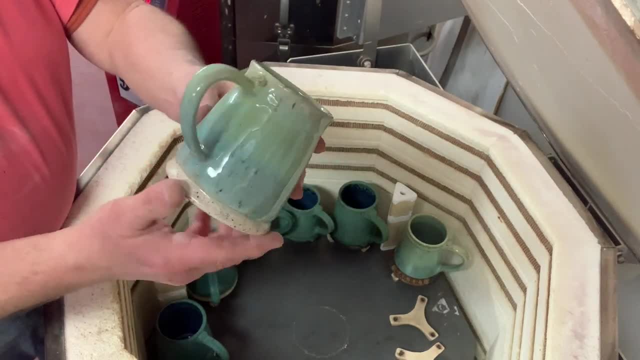 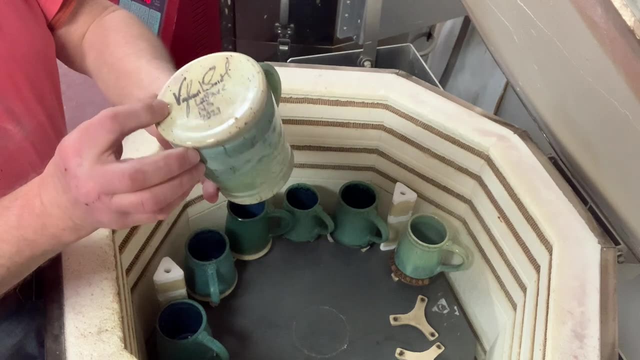 This is the blue green copper red. You'll find that one on the internet somewhere. Just type in blue green copper red in Pinterest Or glazyorg, whatever it's called, And you'll probably find that one. 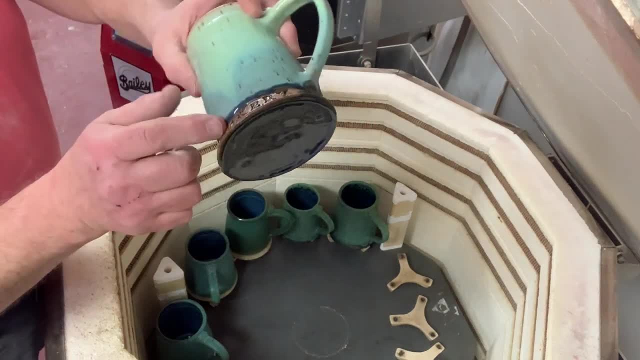 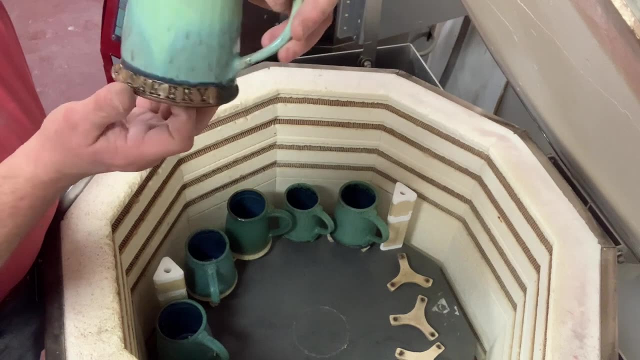 And this speckled clay looks really nice. I dip blue over the bottom of these where the writing is for the bakery, And then the turquoise and the oatmeal above. You can turn it into anything. Yep, the turquoise matte has worked nice on these. 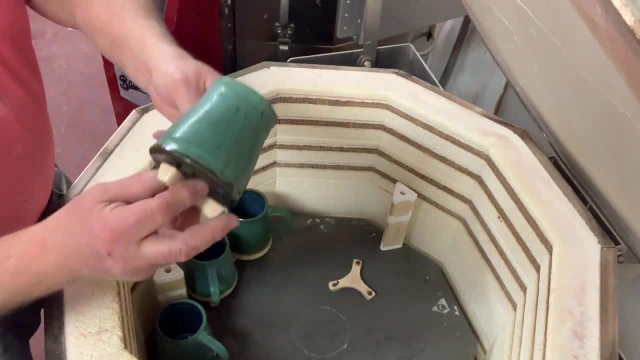 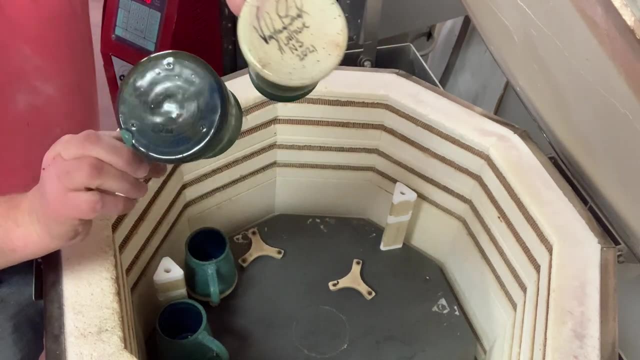 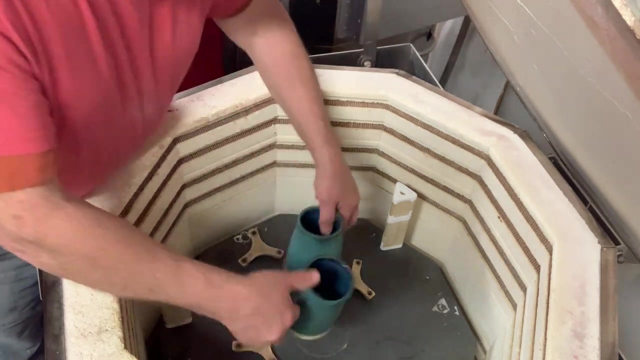 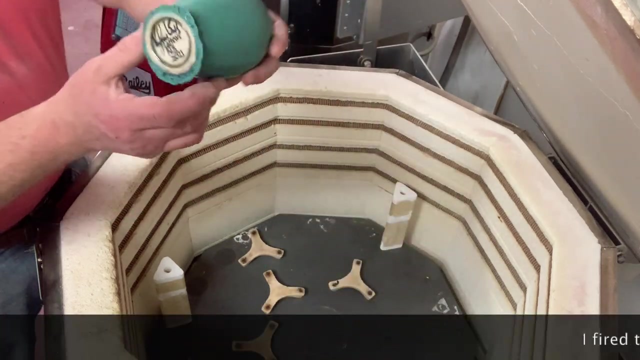 I'll skip through these quickly, because they're all with the turquoise matte glaze Blue on the inside. Yeah, the stilts come right off the bottom easily, So the bottoms are glazed. Another: Ah, the seafoam ran a little bit too. 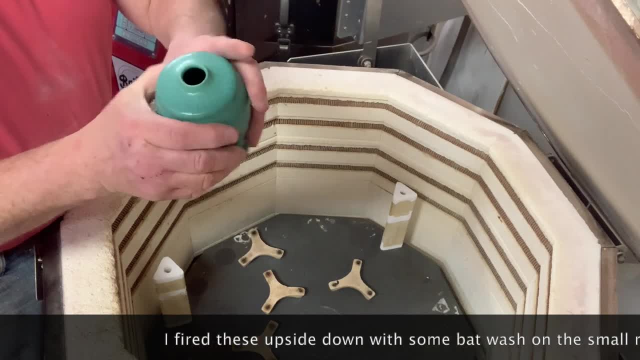 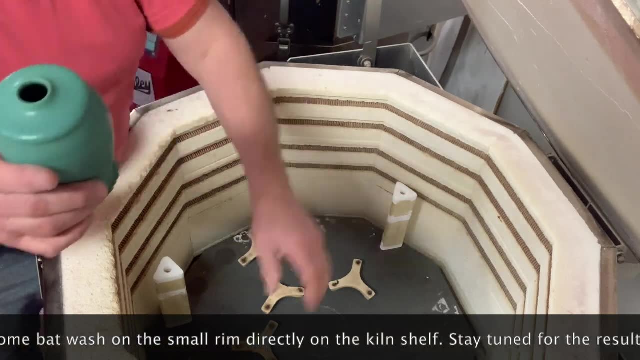 So there's another one that's, But no cracks. That's interesting. These are small, tiny. Use it as a bud vase if you want, But I make them as a lotion pump dispenser. So I've got some grinding to do on those two. 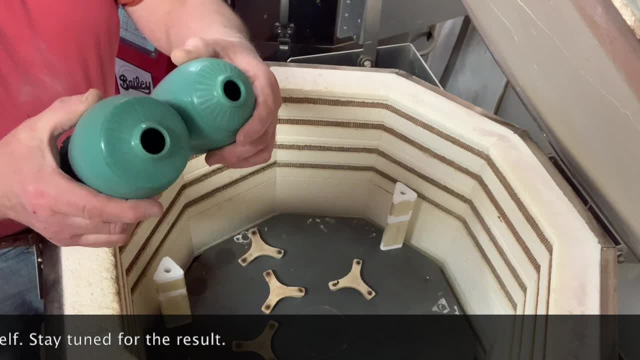 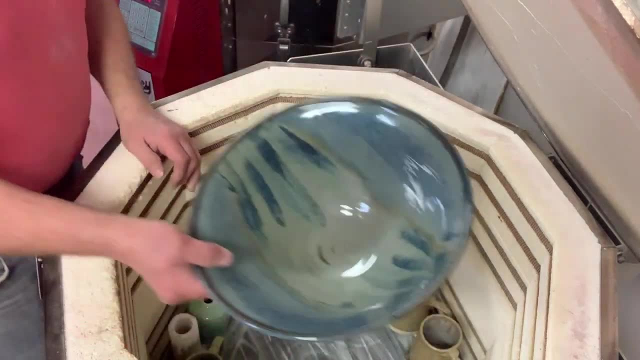 So that means that glazed seafoam. I'll make a note on my chart that it shouldn't be glazed thick near the bottom because it runs A bunch of glazes. There you go. And this shelf has already been bat washed, But it's also needing a second coat because it's already soaking into the 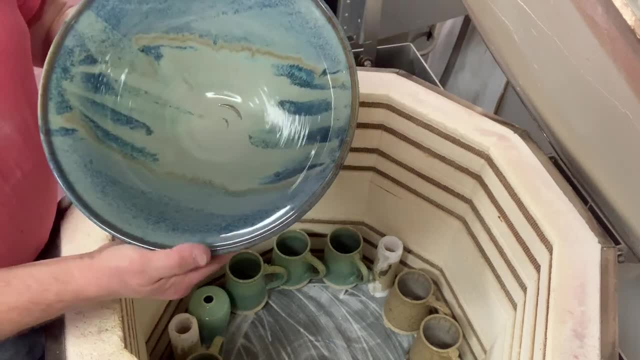 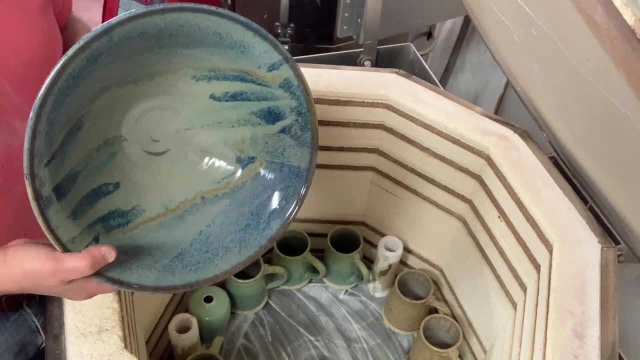 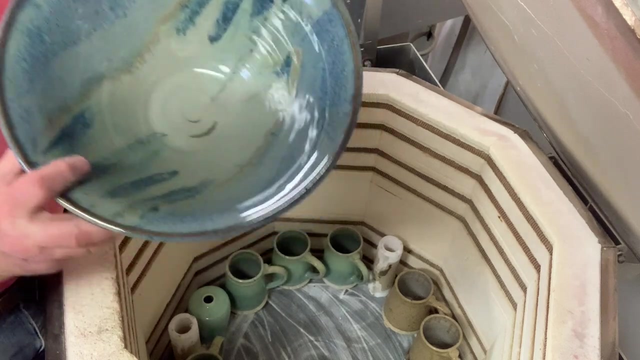 The shelf itself. Look at that one. I did brush work on this one, So it's just brushed with. It's glazed with base coat of variegated blue And then an oatmeal over the two sides, And then brushing other glazes just across randomly with a big Japanese paintbrush. 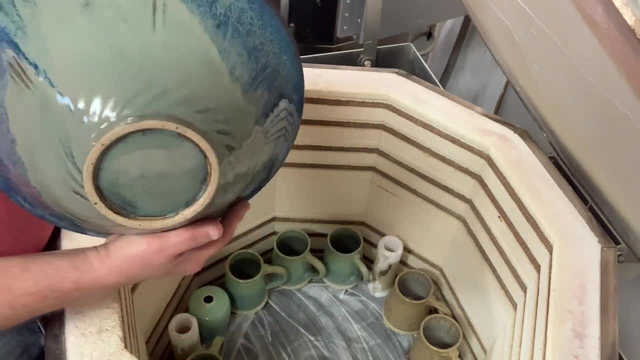 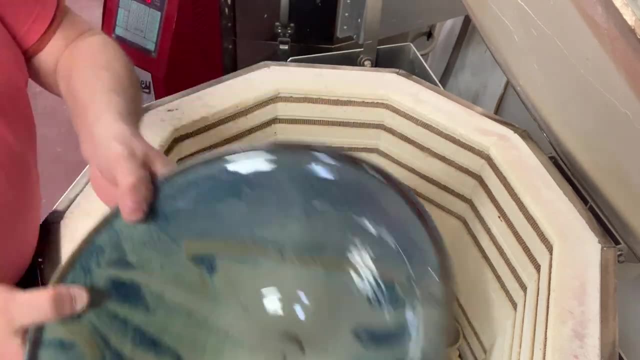 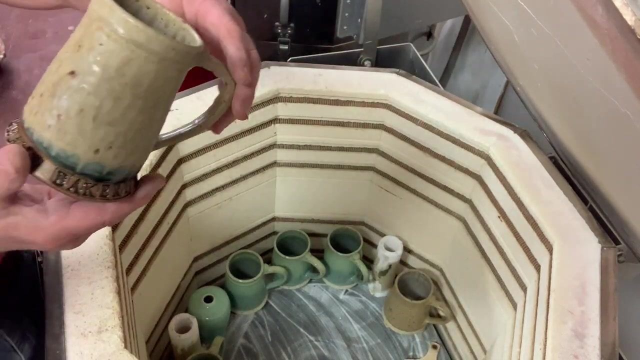 And it's good. on the bottom, Almost ran down That one's almost touching the shelf, But that's a nice big ball There. Now I have an experimental glaze Which It's doing. okay, It's the fake ash glaze. 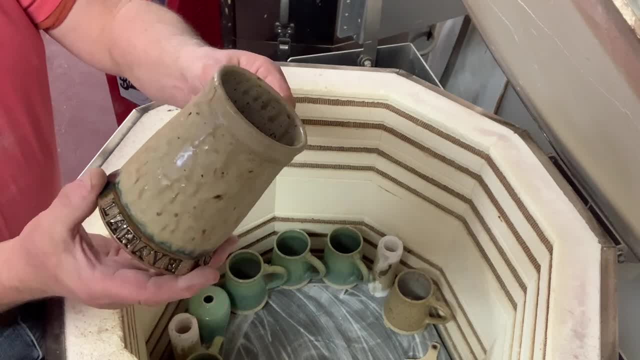 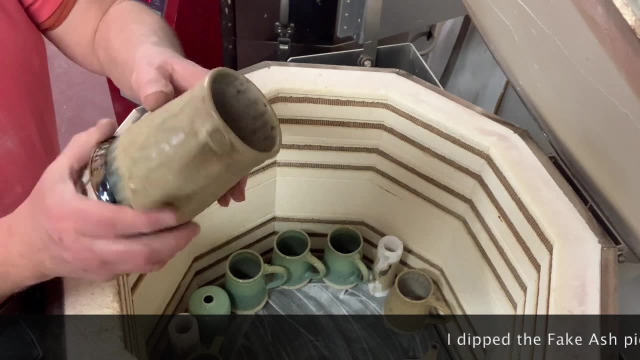 And I would say that looks a little overfired. I did oatmeal on the inside But I would say that one's a little overfired. So this kiln may have overfired a little bit, I don't know. 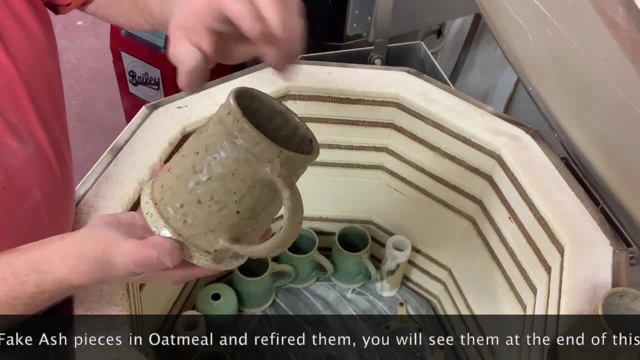 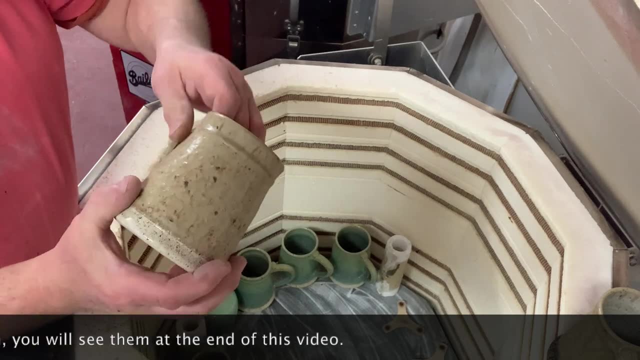 I'll have to check it with a cone next time, Because that glaze is supposed to go to cone six, But it's bubbling a little bit. It's not sharp, But it's actually bubbling a little bit. Turquoise again. 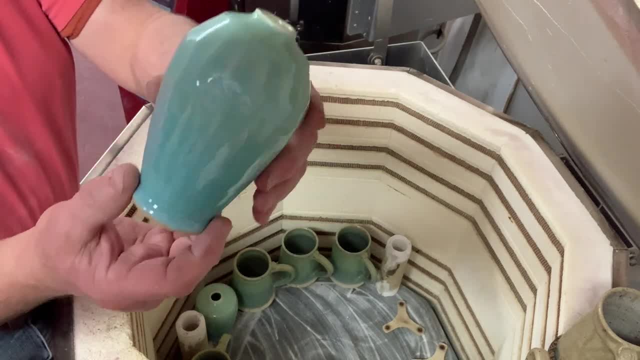 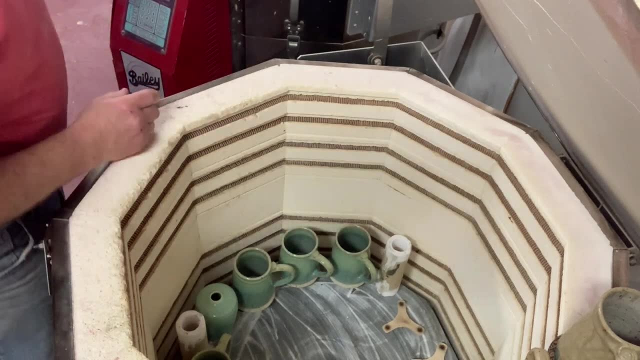 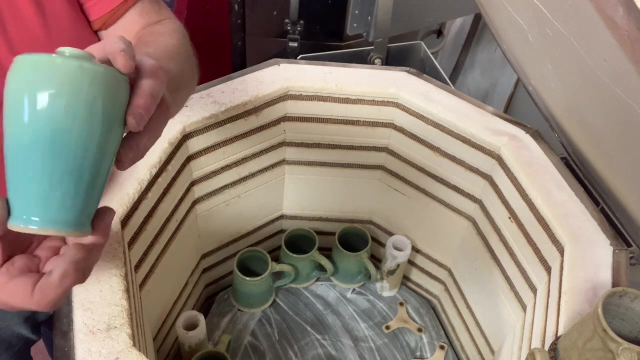 With oatmeal over the top And a lot of fluting in that one Just to kind of You can see better over just about this side. Yep, Perfect on that one too. Blue, green, copper, red, Pinterest, Or look it up on. 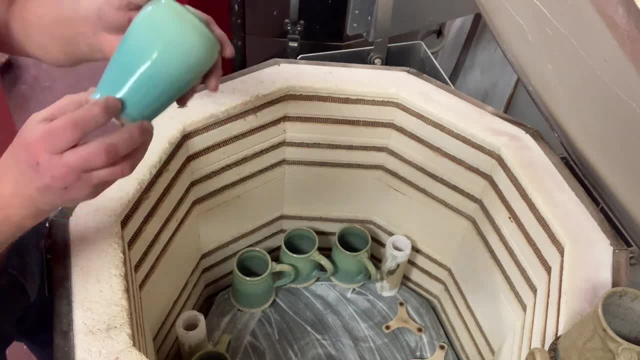 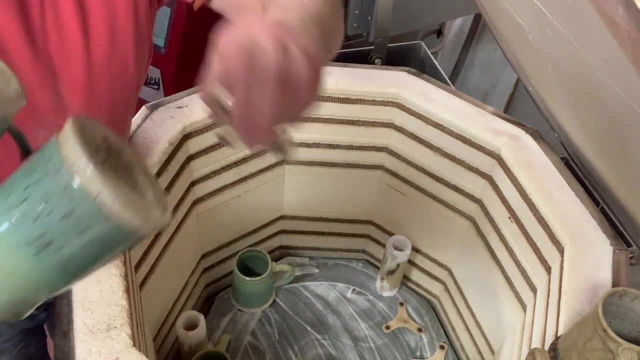 Where do I think The other site I go to is glazyorg, But blue green, copper red. There were some of these on the top shelf. This is the same blue green, copper red over oatmeal clay. 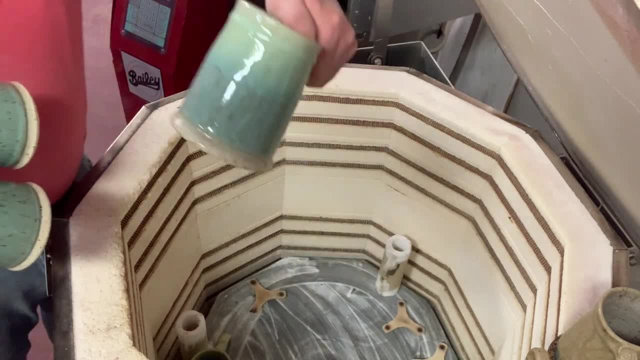 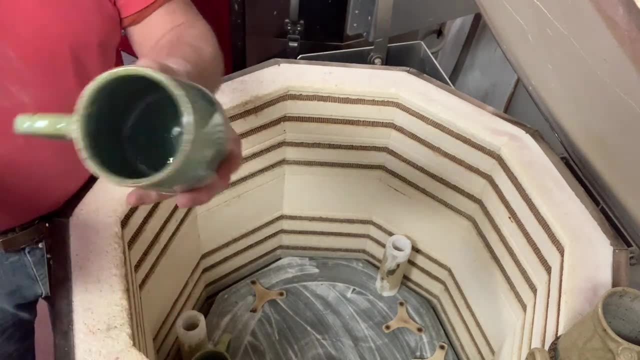 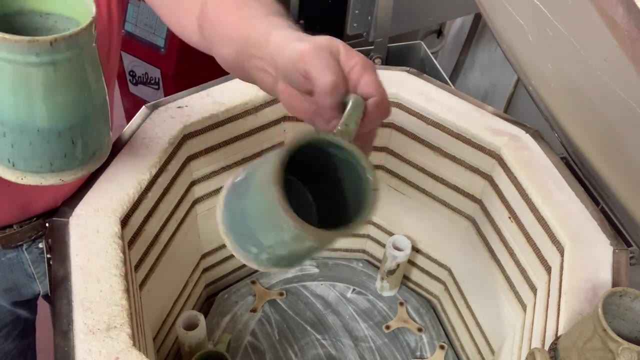 Same again. This is perfect. These are the. It's from Toronto Pottery Supply House, Number 455.. I love throwing it. It stands up well when you're pulling up. It's smooth, But it has a little tooth to it. 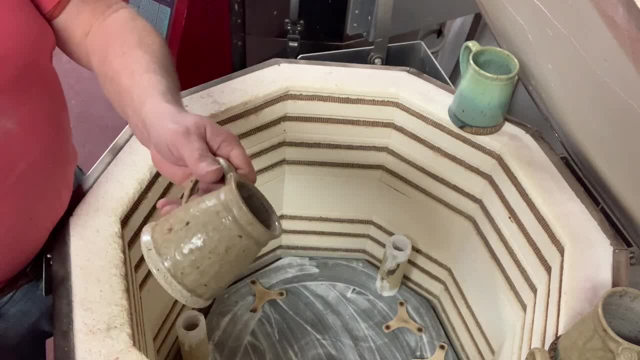 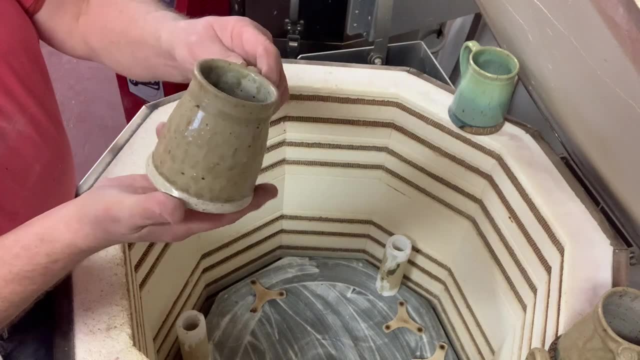 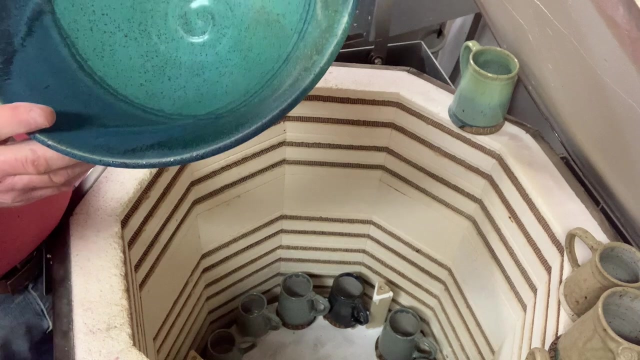 Another ash glazed piece. I only did a few of these because I was wondering What it would do, And it definitely has the appearance of maybe over firing for that glaze. And here we go. This is a large matte- green, Matte, turquoise- sorry, 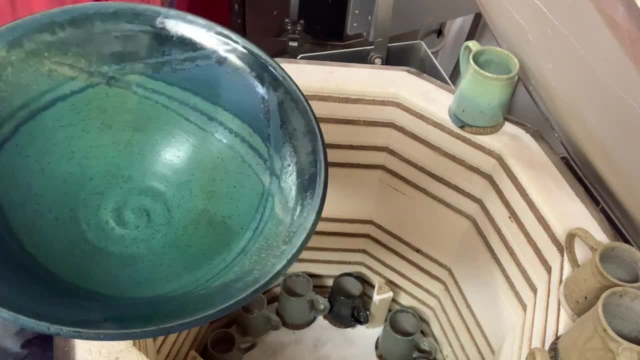 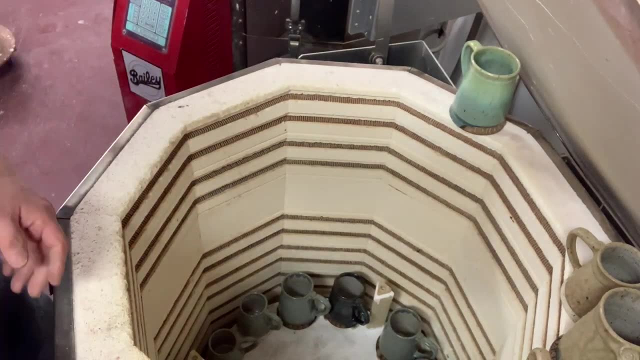 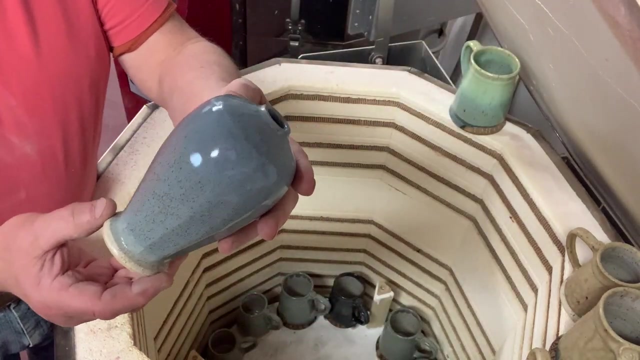 With a blue swipe and an oatmeal swipe And a little slip trailing. You'll see those lines. I do that with slip trailers with glaze in them- And this is an experimental glaze that I have no idea how to ever get this again. 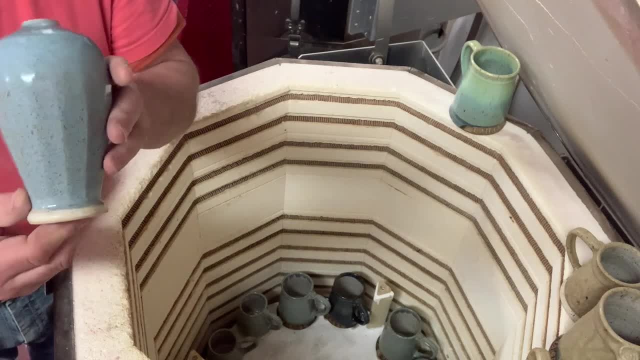 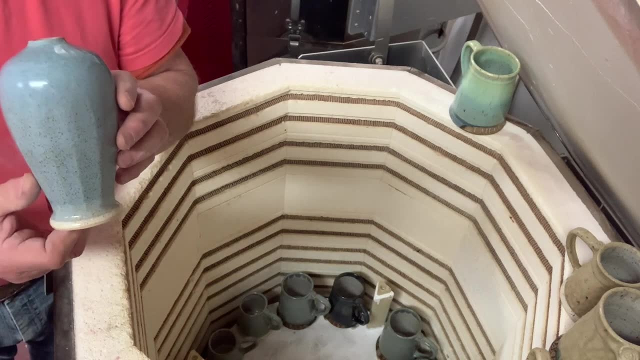 Because I did it with all my glaze slops And basically added some cobalt to it And this is what it turns out like, So it's pretty nice. It's baby blue. Yeah, I'm happy with that, Because that's. 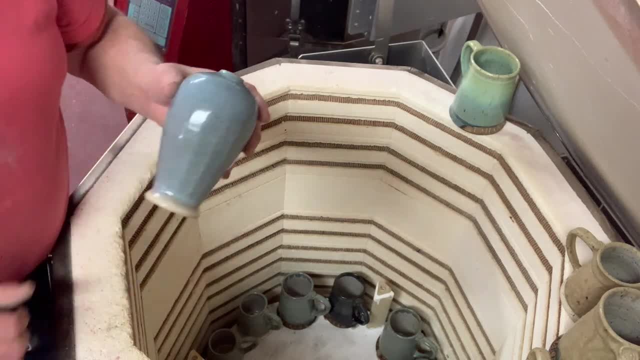 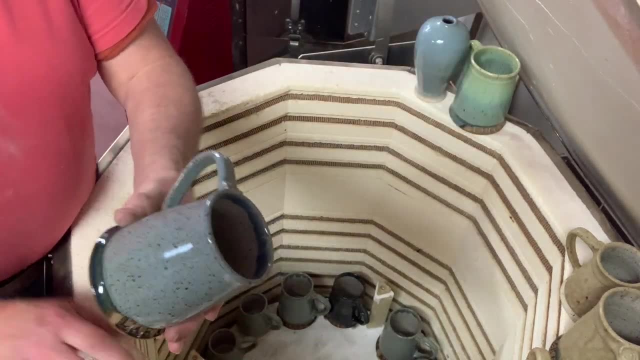 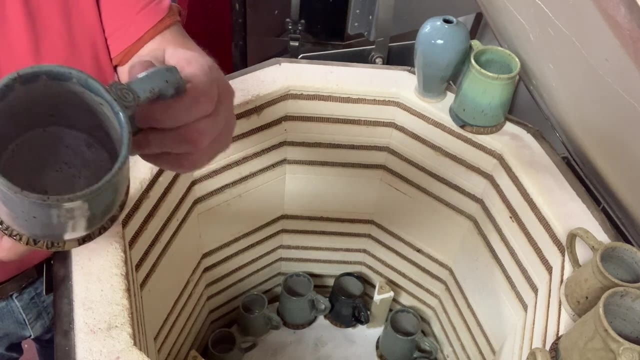 I have three and a half bucket, five gallon buckets of this glaze, But it's looking good And here it is on the speckled clay, So baby blue. I kind of like that. now It's nice when you can use all your scrap glaze. 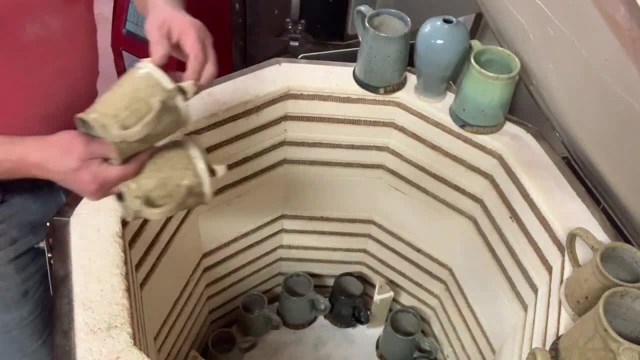 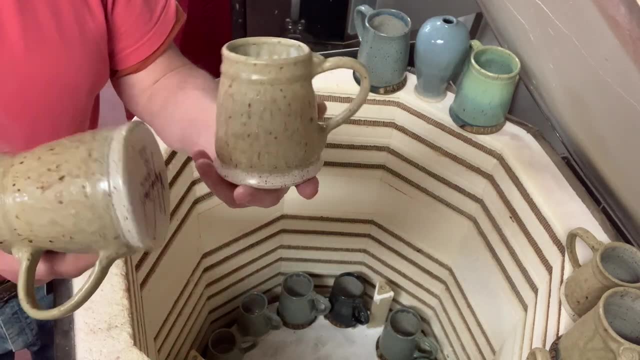 Scrap glaze is basically from all the sponge wiping pails that you use And then you've got all that debris in the bottom And I hate throwing anything out because of the toxicity of raw glaze going into the environment. Once it's fired, it's fine. 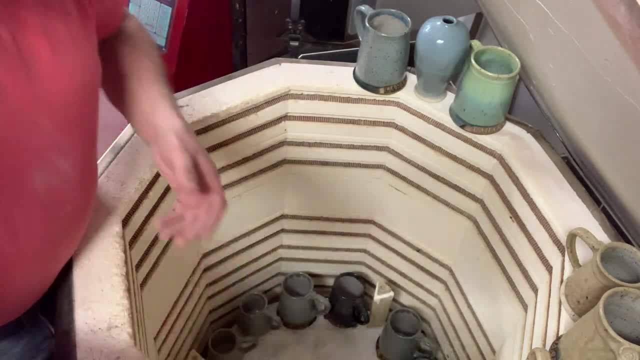 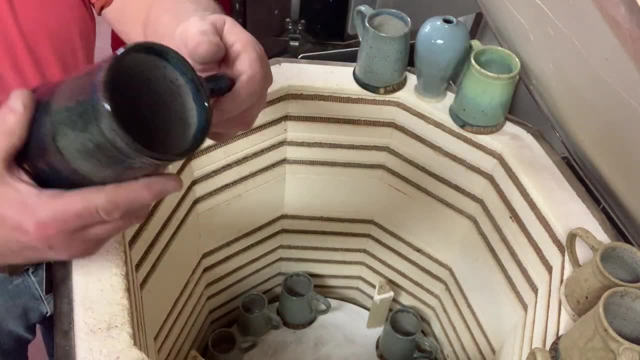 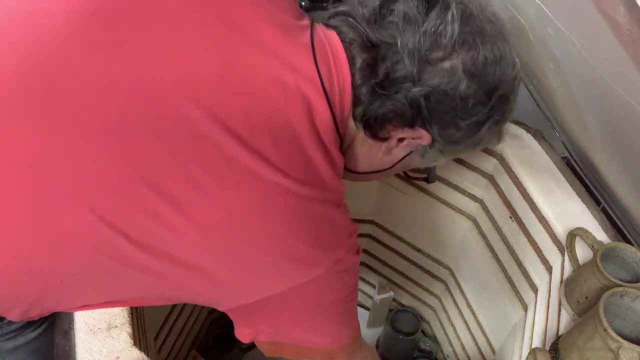 These are all going to get re-fired. I'll dip another glaze over them, Probably the oatmeal actually, So I've got to mix them. This is the dark blue, More of the baby blue. See, the stilts just fall right off. 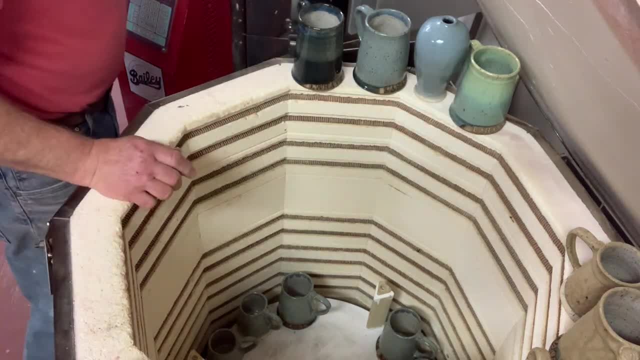 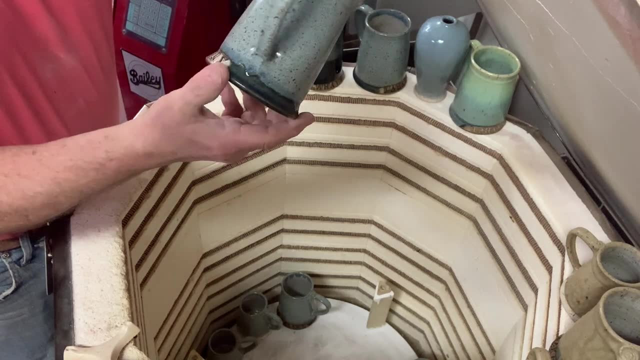 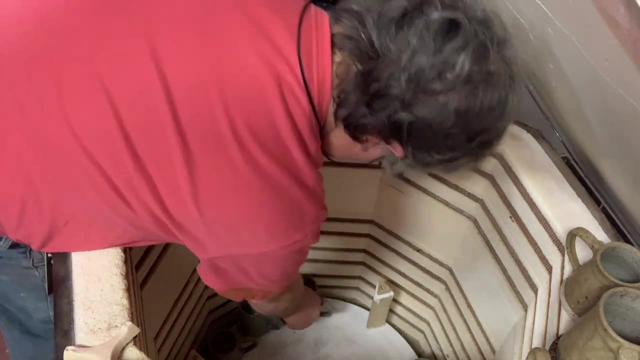 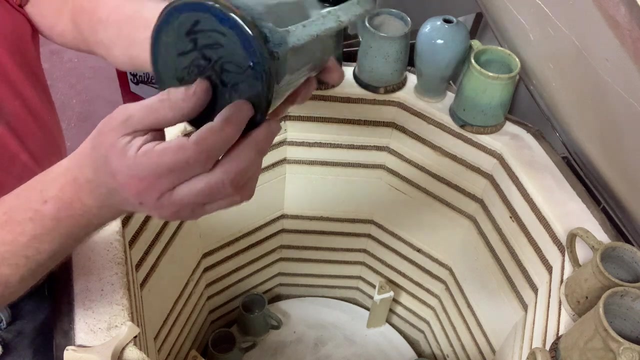 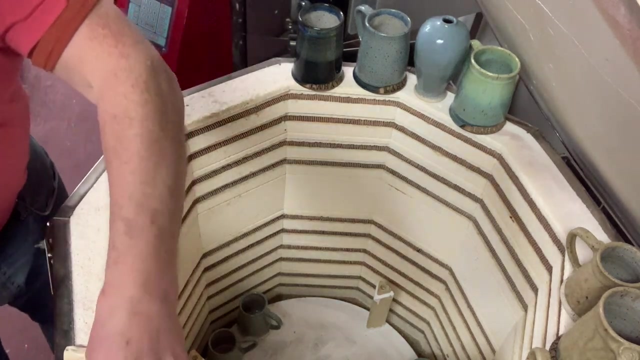 I mean, they basically are easy to take off As long as you don't glaze the bottoms thick. Yeah, that's a nice speckled clay combination. I left a stilt pin So to get that figure out where to just put that down. 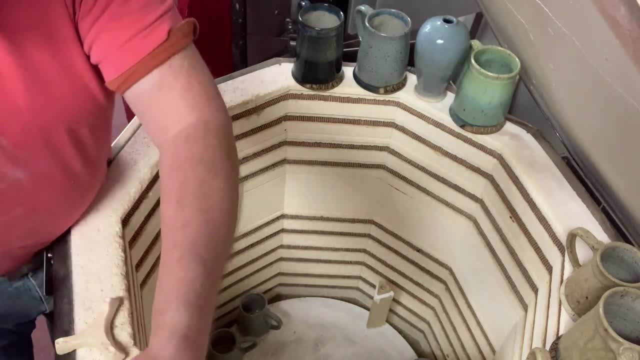 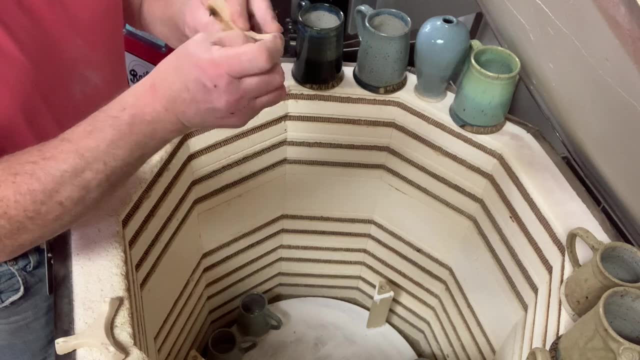 Oh well, we will come back to that afterwards. There it is, The pins will come out, But then you can put them right back in, Find out which way round it was. Use a pair of pliers, in case it's sharp. 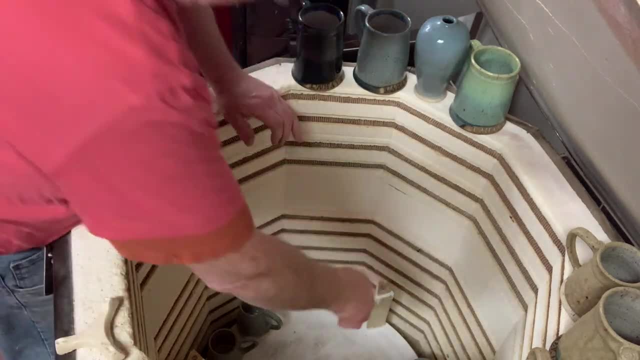 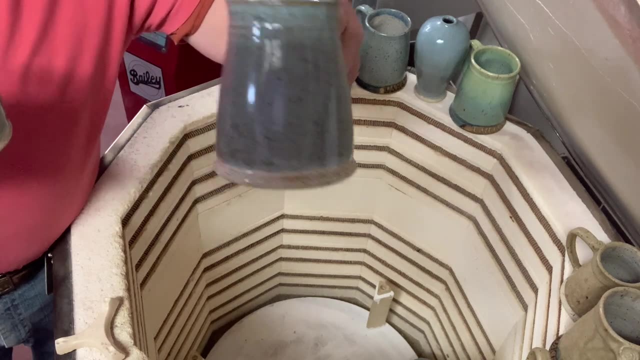 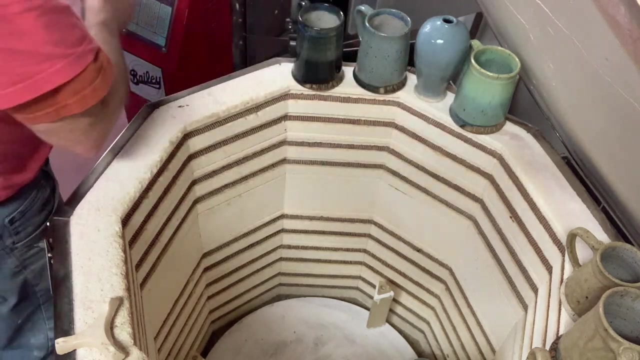 But you can put the pins back in- And two baby blue little mugs. These are like smaller than my usual mugs. These are like smaller than my usual mugs, Alright. And lastly, another lotion pump, Baby blue. 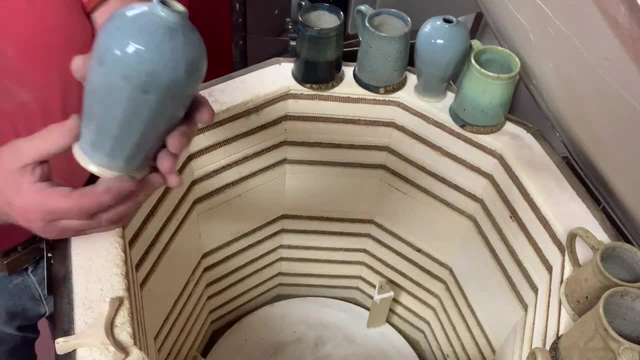 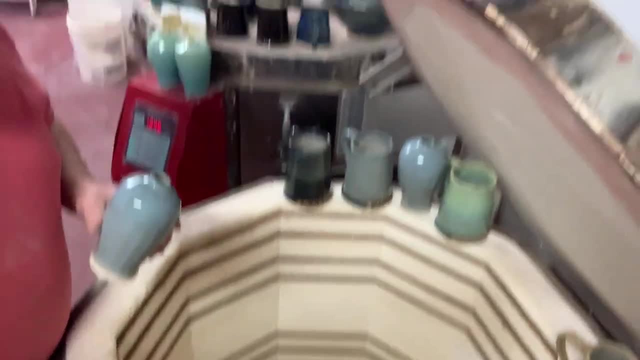 Okay, so The fake ash glaze is on Pinterest, I think as well, Or glazeyorg, So beware of that one. I'm testing it at the moment And it needs to be fired at a slightly lower temperature. 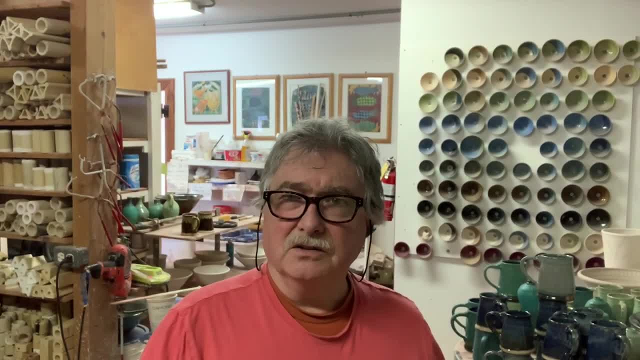 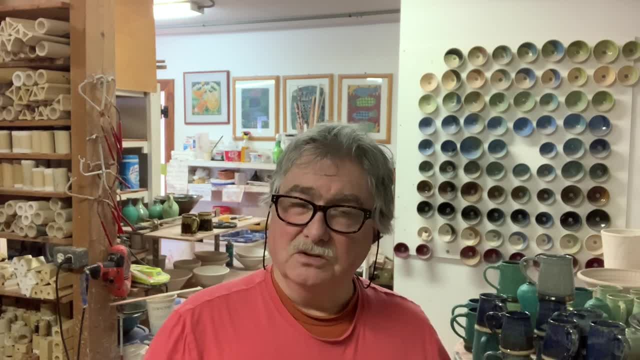 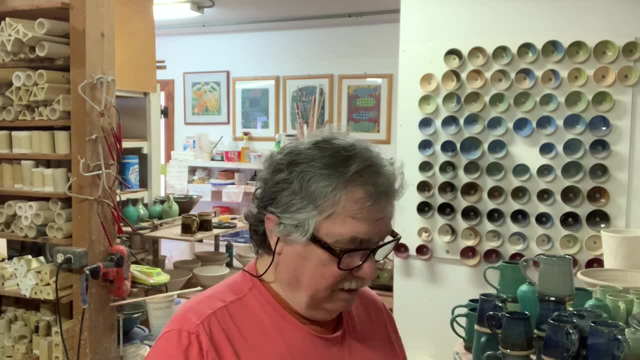 And then I'm going to put it in the oven, Or I'm going to add some silica to it, Or I'm going to add some silica to it To raise the firing temperature, Because this was not an overfiring. Everything else is perfect. 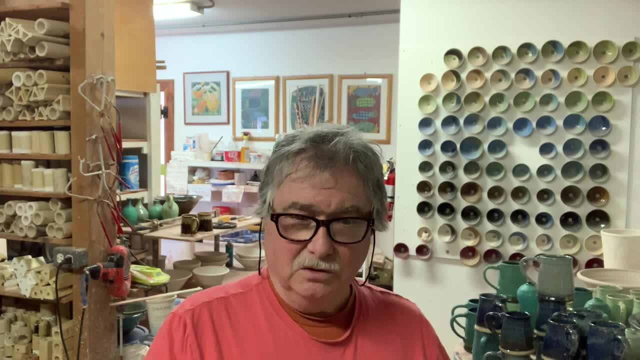 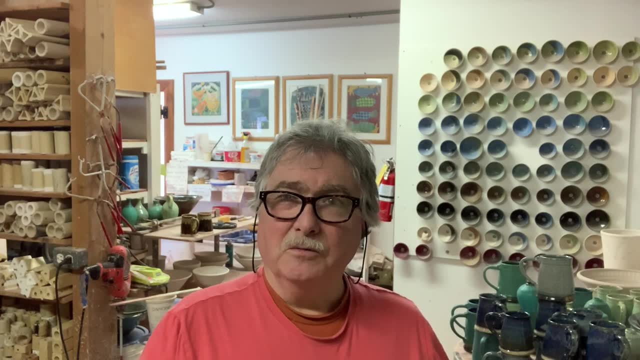 And the blue And the variegated blue would have run like crazy, And the variegated blue would have run like crazy if it had been overfired. So I wonder what's going on with that glaze. But anyway, that will go to the next kiln. 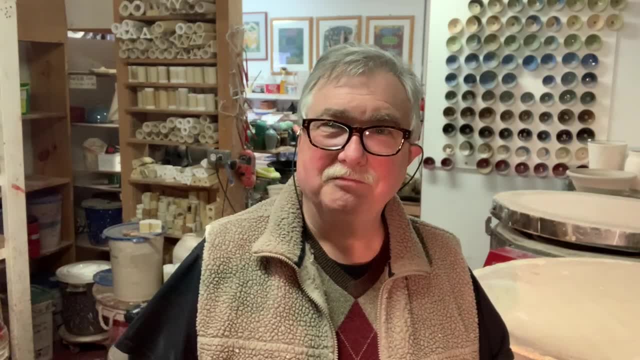 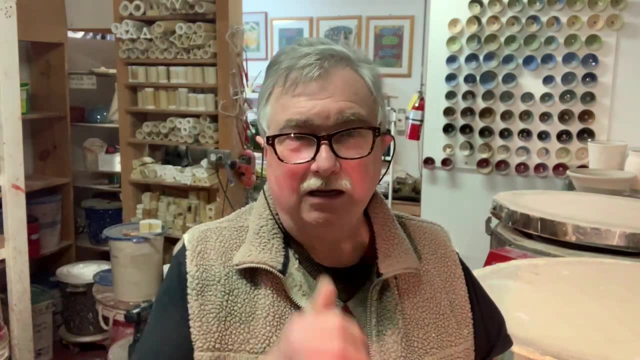 Alright, this is the second kiln. Alright, this is the second kiln. Basically glaze firing tone 06.. Basically glaze firing tone 06.. At 2225, And then 125 degrees slow cool. 125 degrees, slow cool. 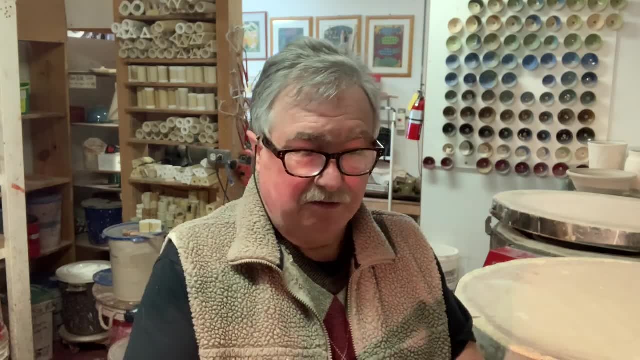 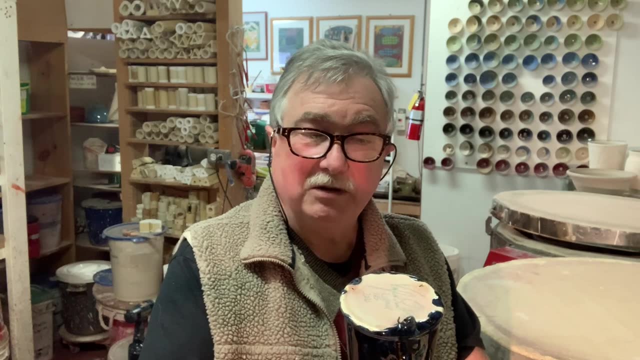 to 1750 with a 1 hour soak again. Alright, so this piece ran a little bit too, So this is confirming that I need to lower my glaze temperature a little bit so I can stop this running. And it's on stilts. 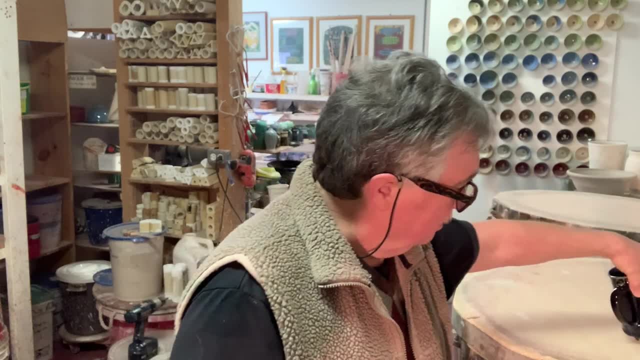 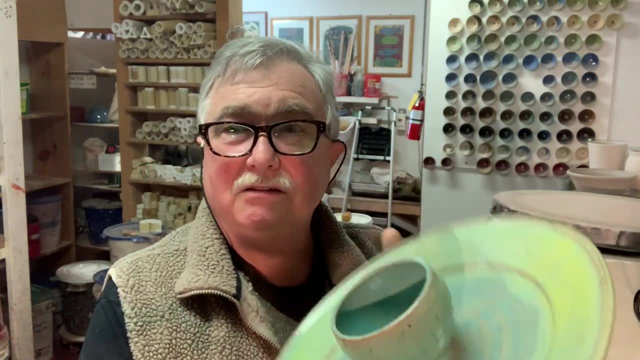 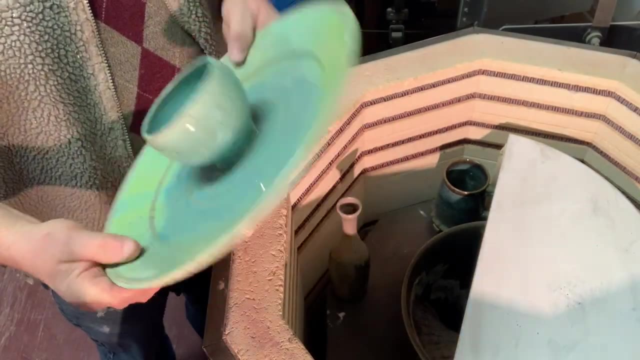 so I can grind that off easily. But that was what we found in the other kiln, With a few pieces, not all the pieces. Here is a nice- Let's get you looking at this. Here is a nice chip and dip in the blue, green, copper, red. 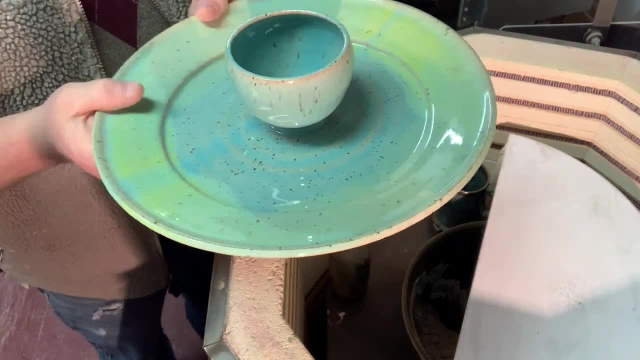 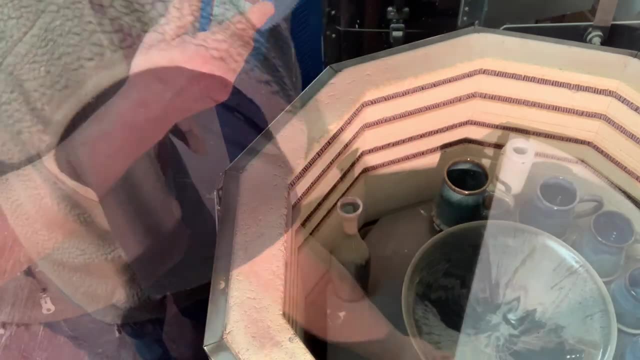 speckled clay 455 from Pottery Supply House, with some yellow oatmeal on the rim. That's what gives it a nice summery look. Wow, Now it's like what did I do here? Oh, speckled clay. 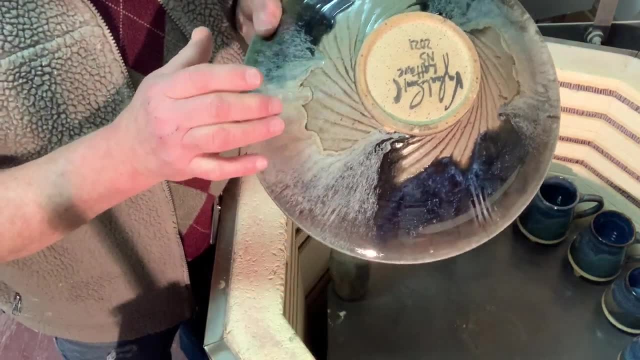 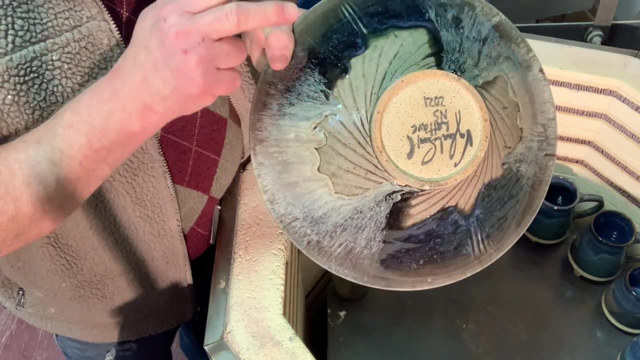 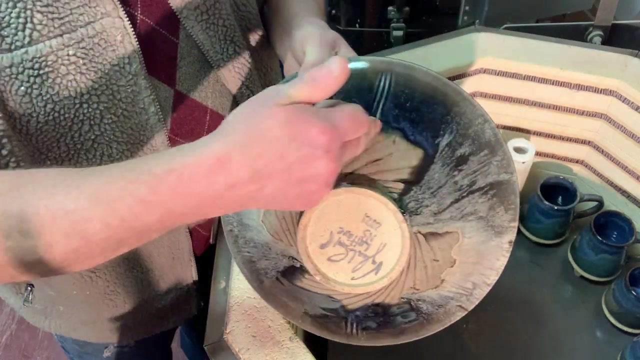 Okay, So outside always tells you a little bit better. Mouse grey over speckled clay. So that's that. mouse brown in Mastering Cone 6 Glazes. My oatmeal was swiped over that way, and on the inside too, And then my dark blue, or bright blue. 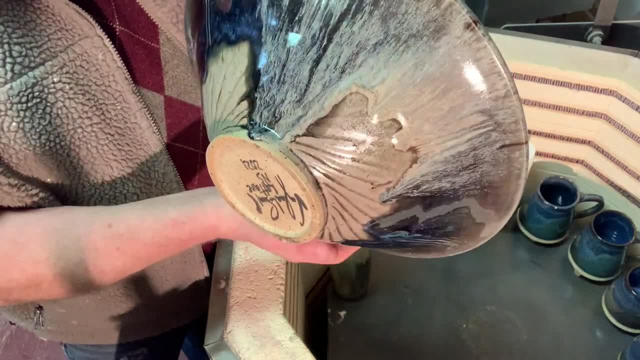 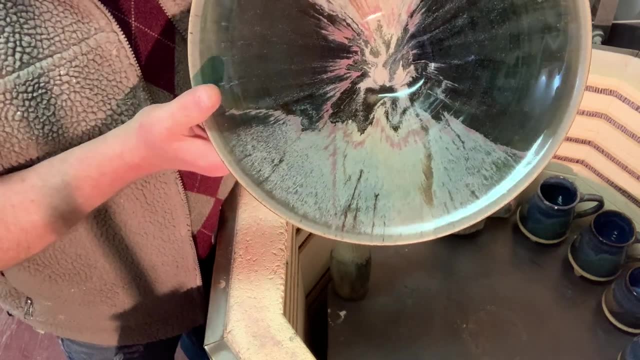 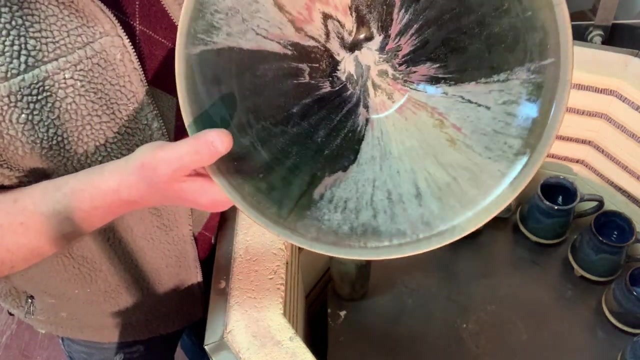 was swept that way. Look at that little run right there Didn't touch the kiln shell Still flat, And then on the inside Slow cool where the glazes kept running down for a long time. So I think I might try a faster cool from. instead of 125 down. I think I might slow the cool down- sorry, faster the cool speed, the cool up from 2225 down to about 2000 and then do a slow cool 2000 to 1750 and see if that reduces the amount of running. 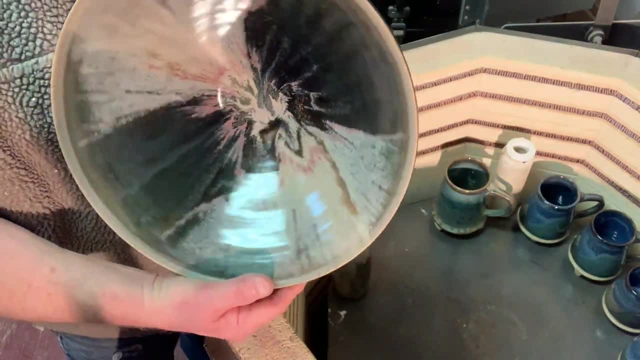 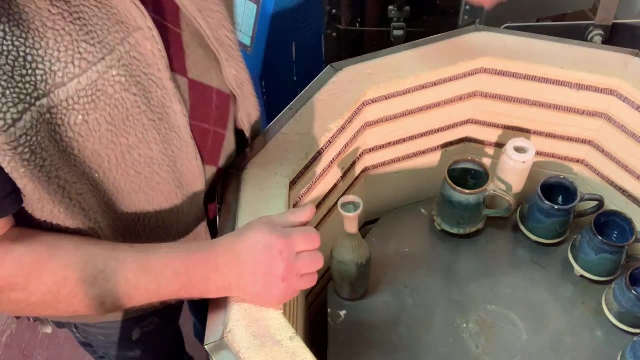 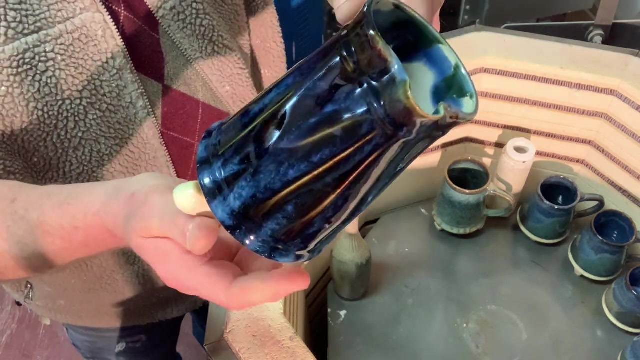 But it's really nice. And then, almost touched the kiln shelf there, Here's another one of those black ones that ran down. This is the licorice with blue over it, and it really does that luminous blue look. But I will have to. 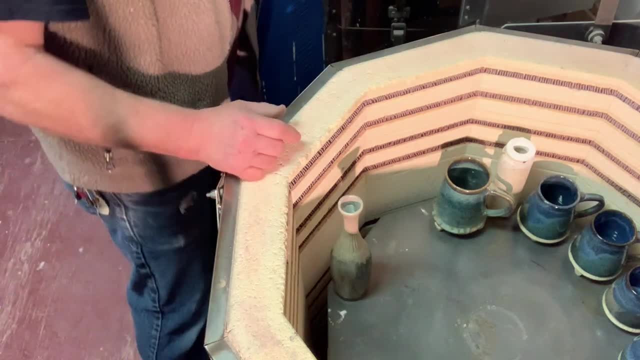 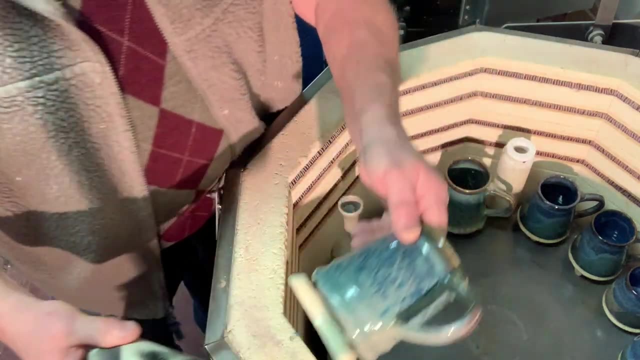 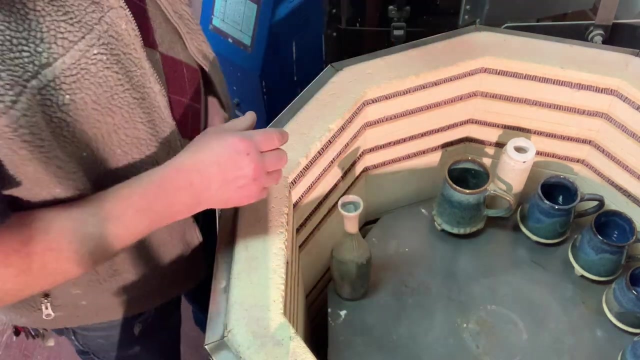 grind that off a little bit there. Here's the grey, which- let's see if I can get one of these to knock this off- And that ran a little bit down there too, Although I think that will still sit flat, It does. 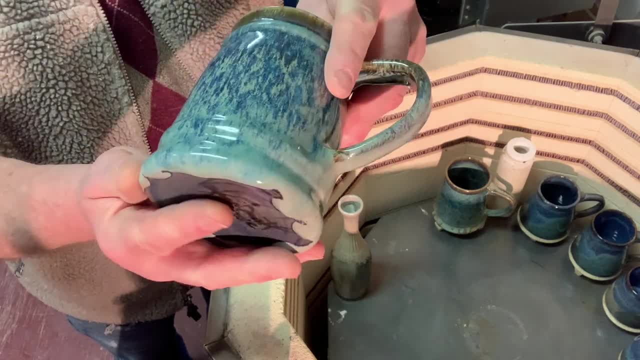 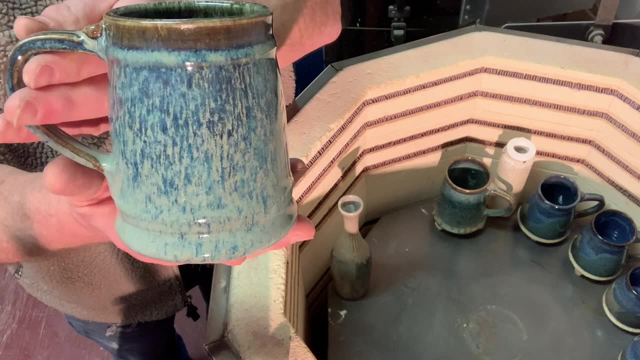 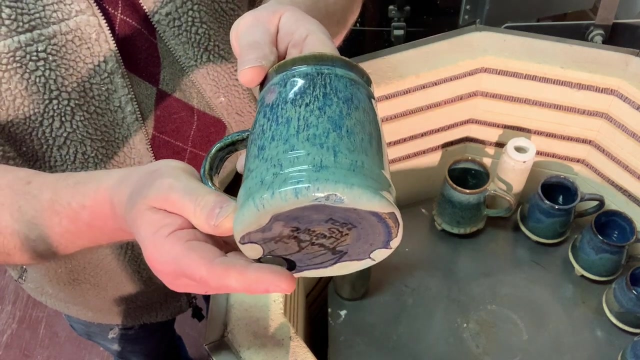 So this is the speckled variegated blue with oatmeal over it, And that's one of the best examples I've seen of that mottling. So that's basically my oatmeal dipped over the top with the variegated blue. 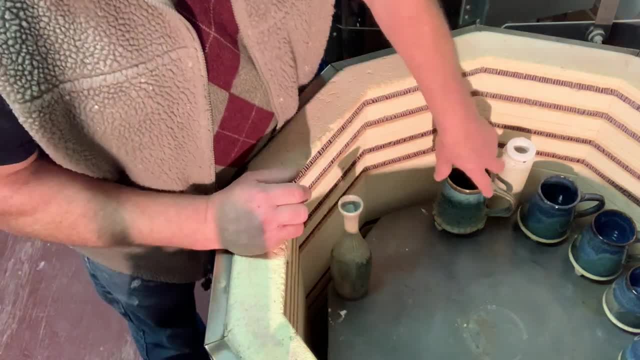 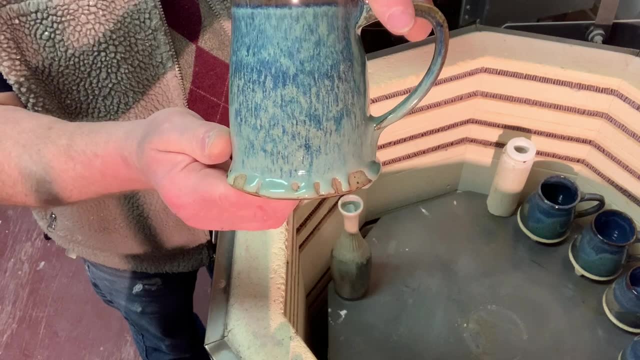 from Mastering Cone 6 Glazes And that sits flat. This one ran too. So this is why I always say with the variegated blue it does tend to run. We got away with it in the other kiln, but this one ran down a lot too. 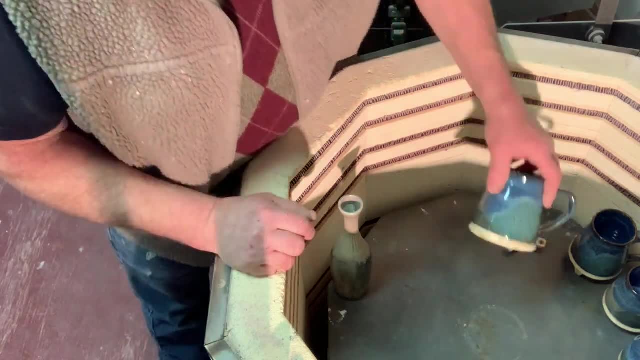 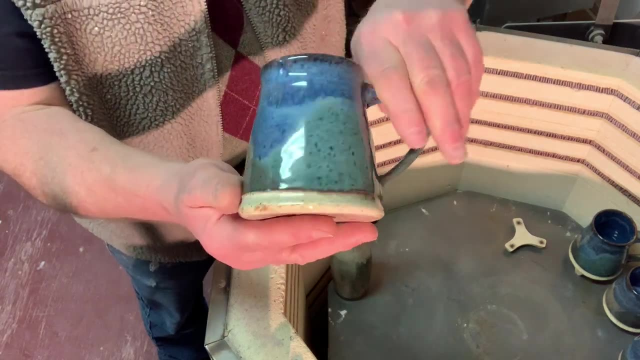 And there's a little bit that needs grinding off there, But then most of my pieces I do a different glaze on the bottom, which is why we don't get the running, And this one I actually had to glaze right to the bottom. 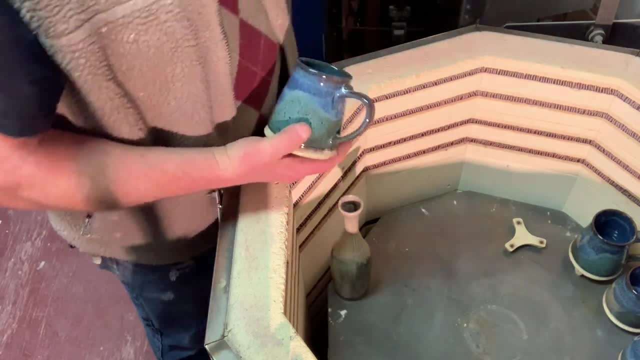 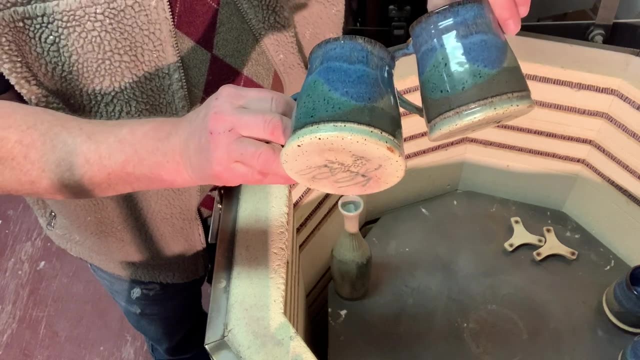 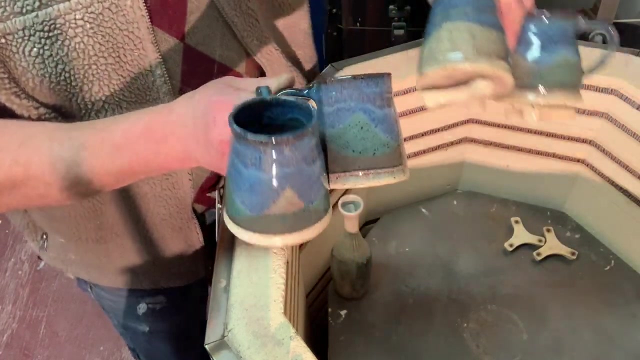 So I've got to stop doing that. These are all my bright blue with dark blue and oatmeal swiped over them, So there's actually a set of four of these. This is left over from the bottle video that I did the other week. 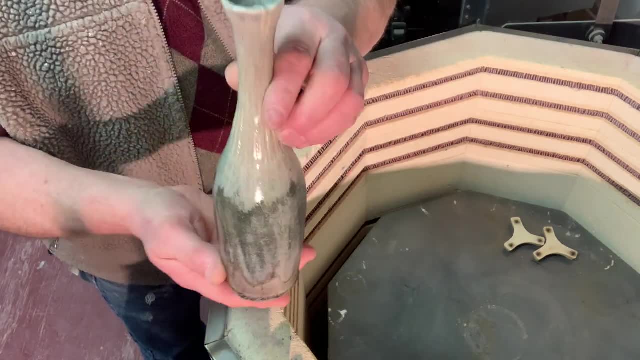 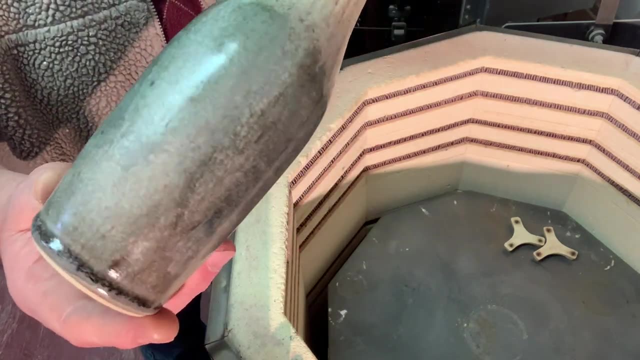 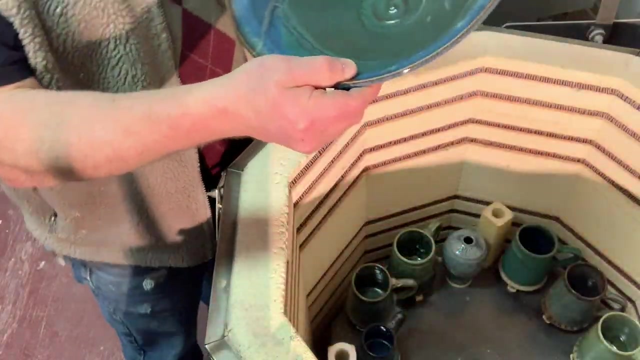 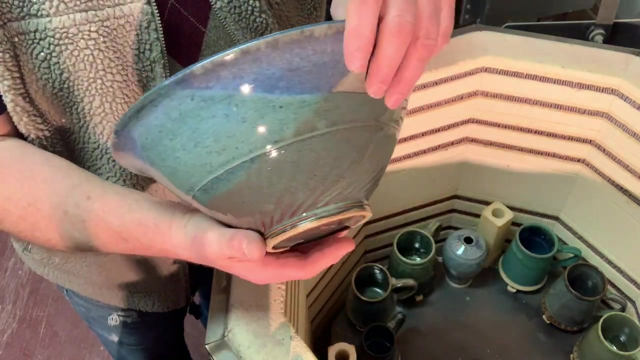 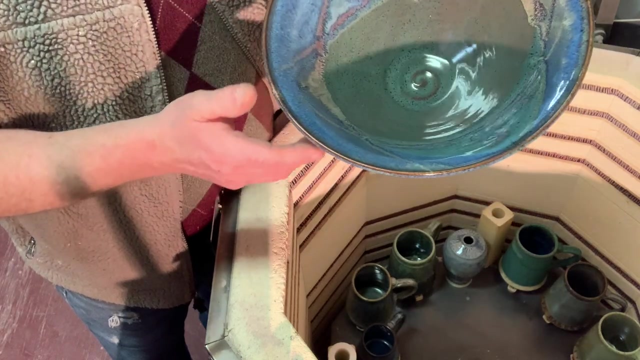 The mouse grey has turned out beautiful in this fire. And then the oatmeal over the top of it. You can see that semi-matte crystalline. That's a pretty ball. And that's basically the bright blue which tends to go green a bit over the top of the. 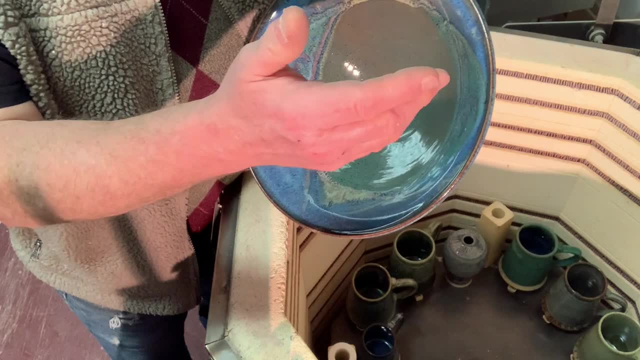 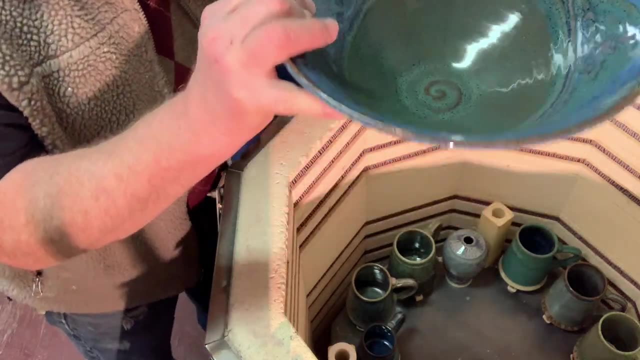 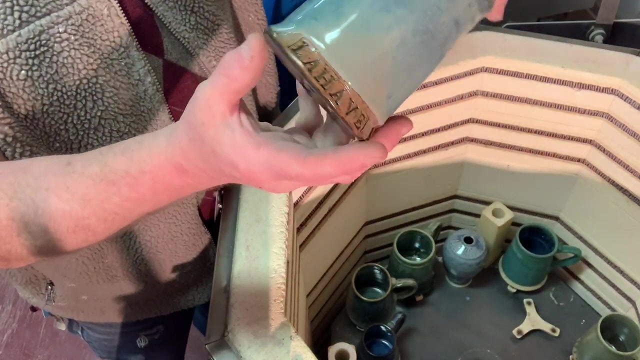 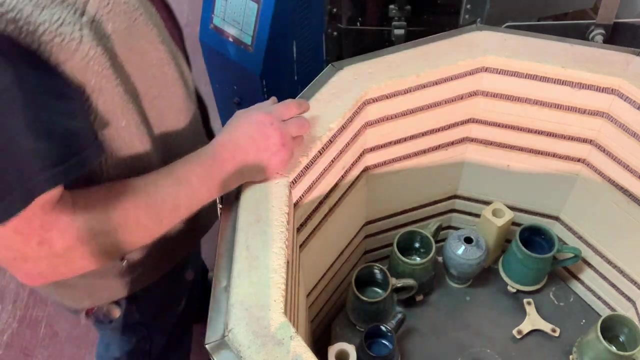 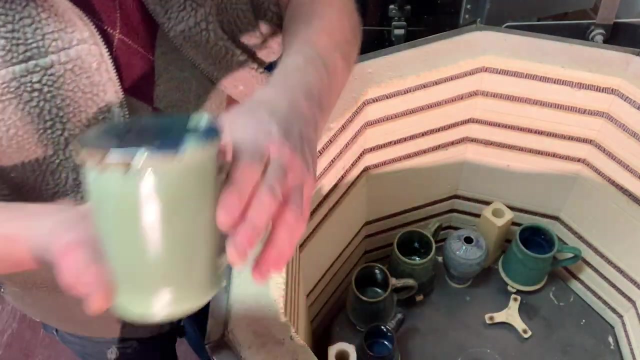 speckled clay, And then my dark blue and my oatmeal swept over it. that way, There you go. That one didn't run. Oh, it did a little bit there, But this is that variegated blue. It's always where the handle is. 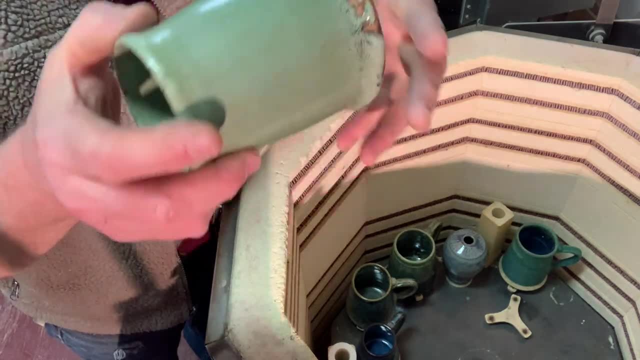 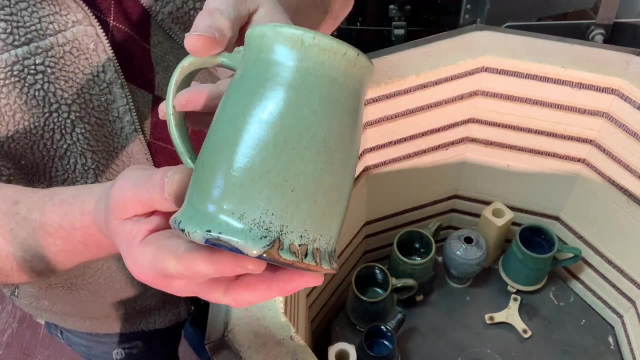 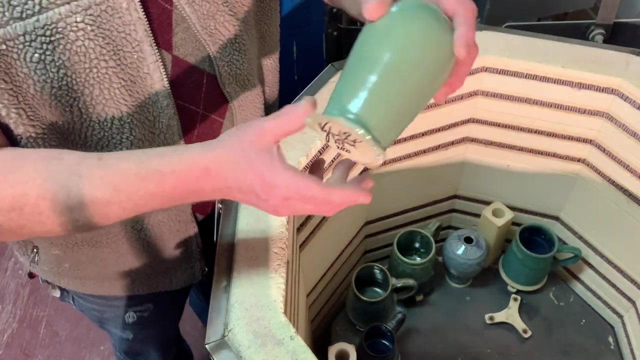 I've pointed that out before. This is that green. It's my apple green. I'm always going to give that recipe to somebody And I've forgotten who it was. Yeah, the green is running like it did in the other kiln. 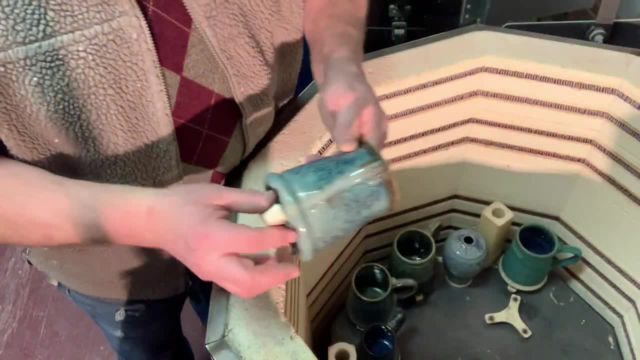 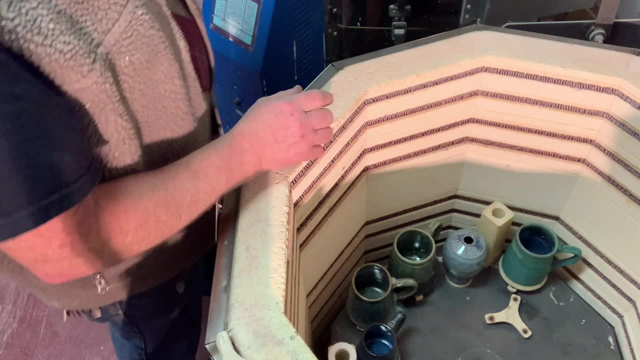 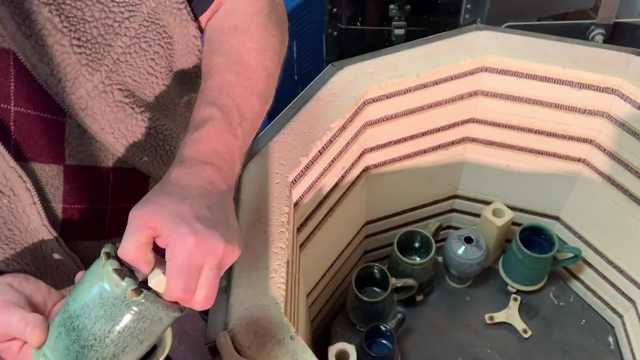 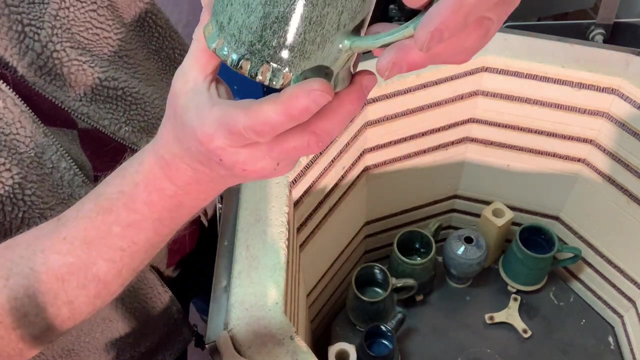 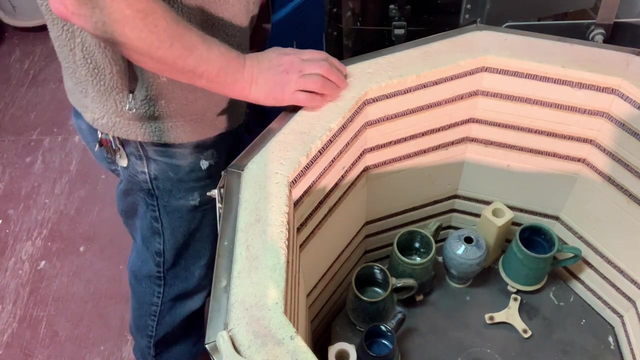 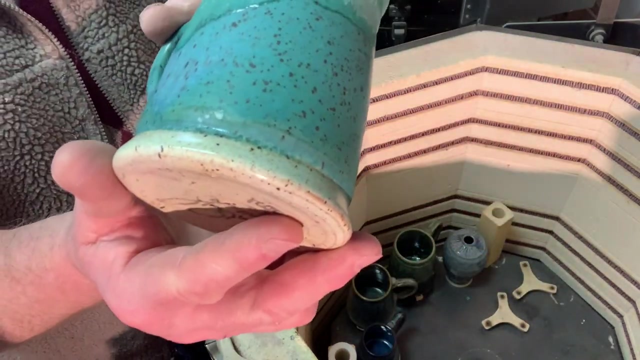 Very giddy blue again. Little runs down there too. I'll probably fire those upside down again. The green and the variegated blue need to be fired slightly lower temperature. Oh, that's pretty. This is the matte turquoise. And then I dipped. 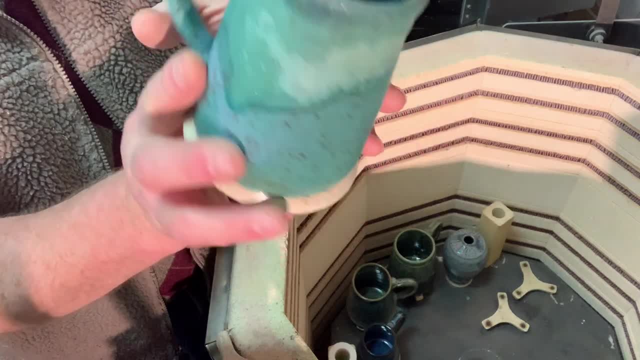 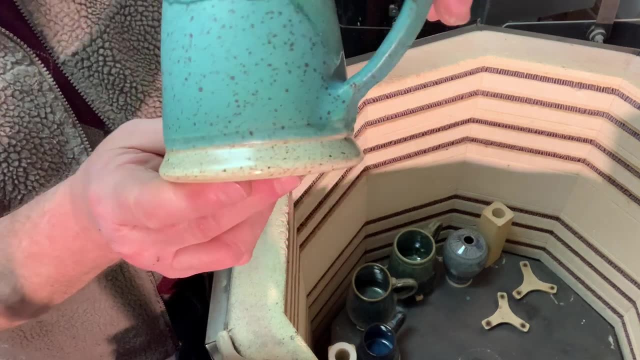 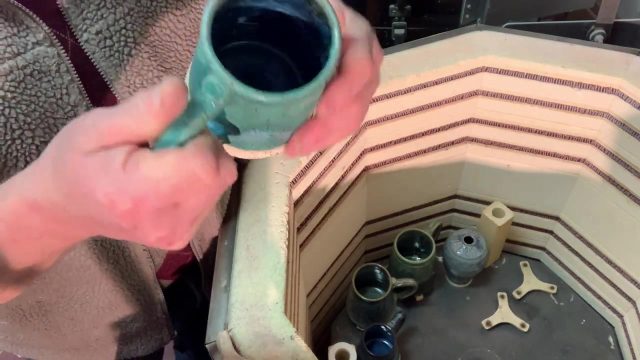 over the top of that. What did I dip over there? Oh, this is the one. I tried the strontium crystal magic again. Now does that feel okay? It's very matte, It's an interesting texture. It's not smooth, It's got a sort of a. 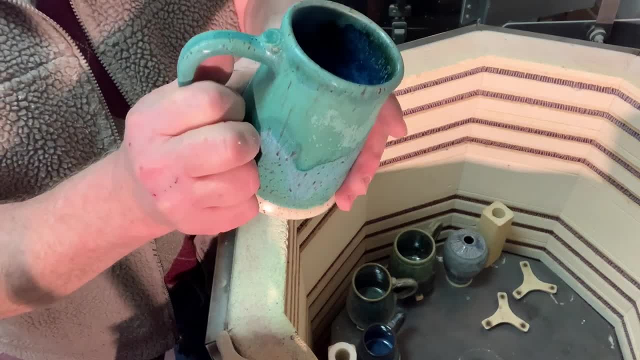 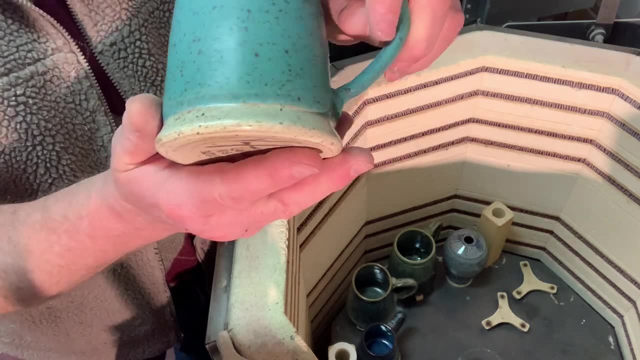 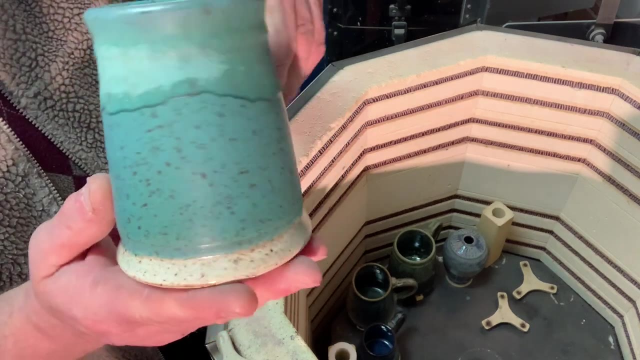 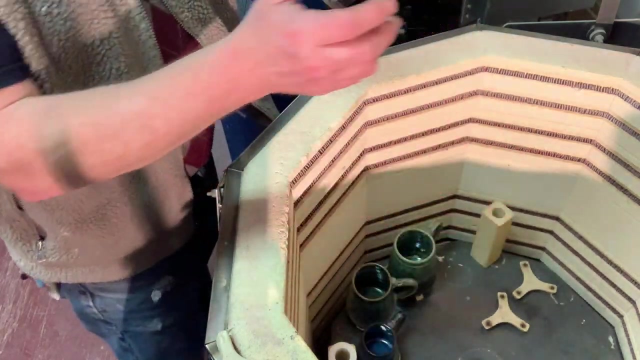 slight roughness- Not rough, but a matte feel to it. I did it over the top of the turquoise, So maybe I should try that underneath next time, But it's really pretty. Look at the way that ran Lotion pumps. 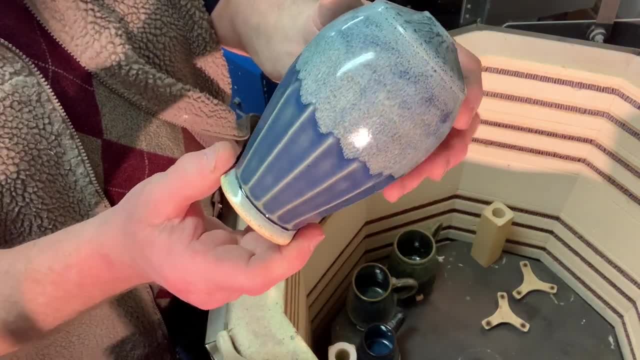 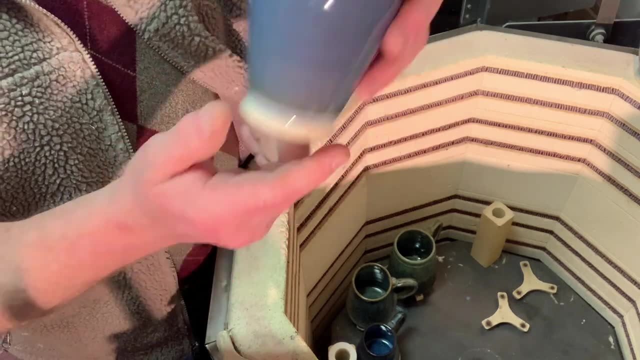 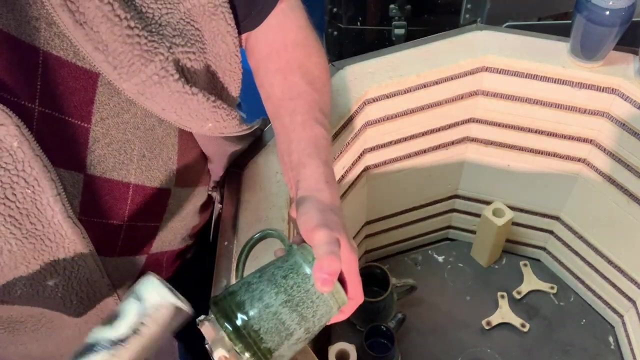 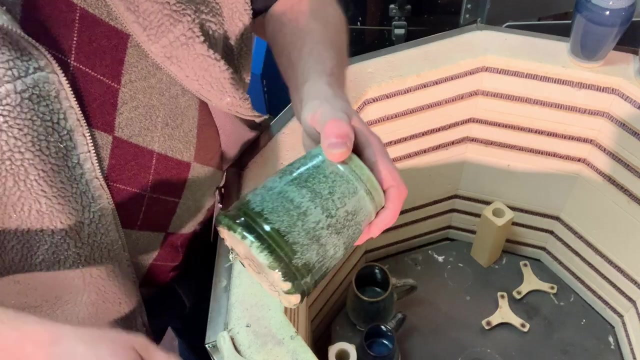 dispensers: Oatmeal over dark blue. Oatmeal over dark blue, without the fluting. Well, that's still stuck on there. Sometimes they come off real easy and other times not. That's the dark green. 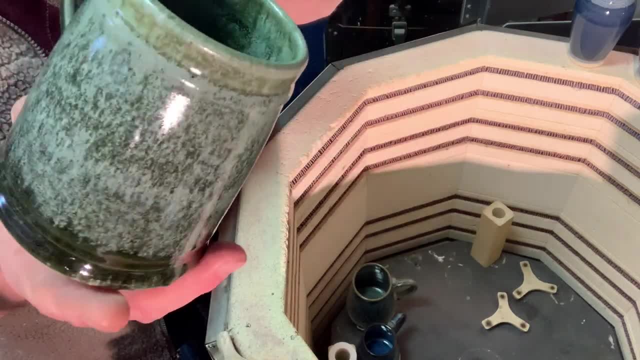 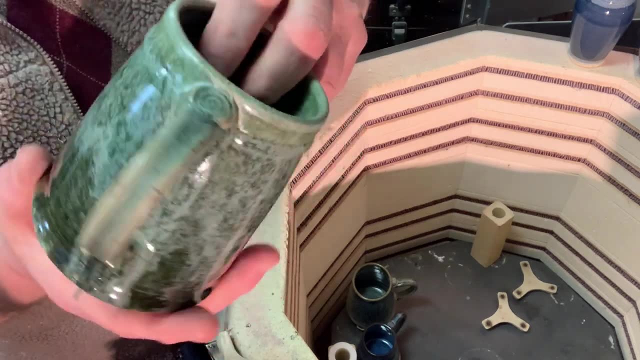 that I have with the oatmeal over the top, But it's always where the handle is. you get a little running that I have to grind, So I'm just going to speed the cool down in the next firing. I've got another firing ready to go, so we'll see. 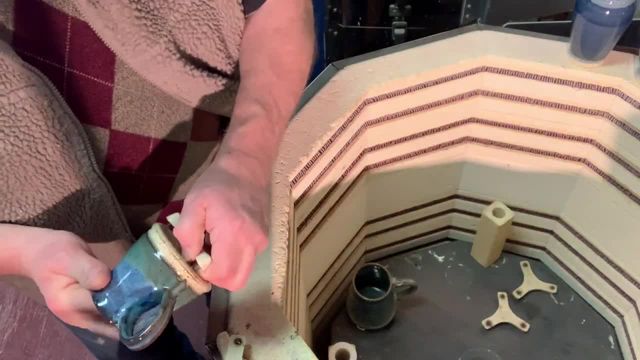 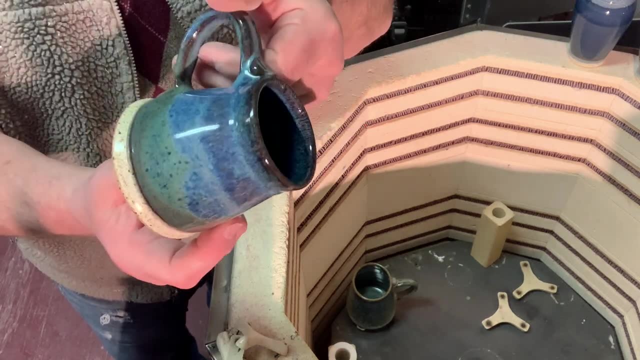 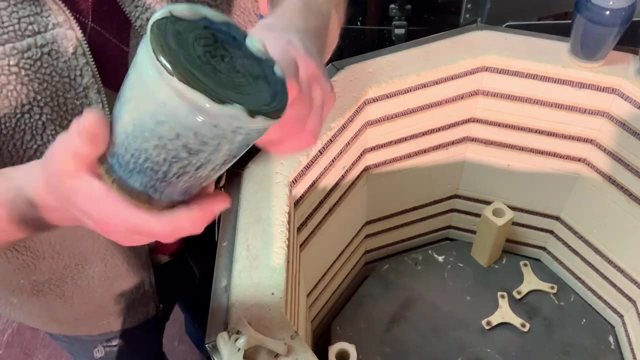 if it works. And yet the blue in all these blue ones, it's perfect. It's one of the things: when you're experimenting with glaze layering over the top of each other, you're always going to get things that do like this, where you're just not sure what it's. 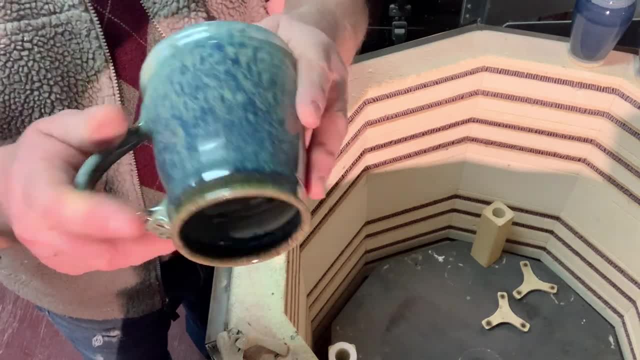 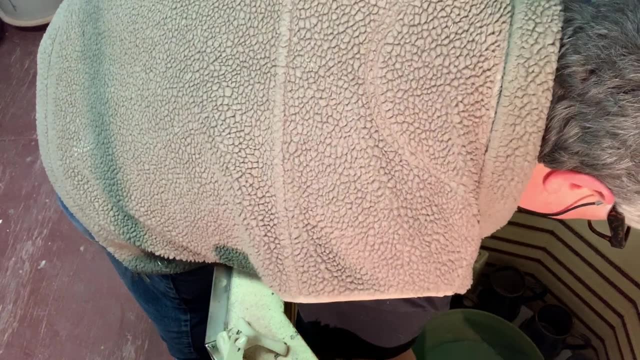 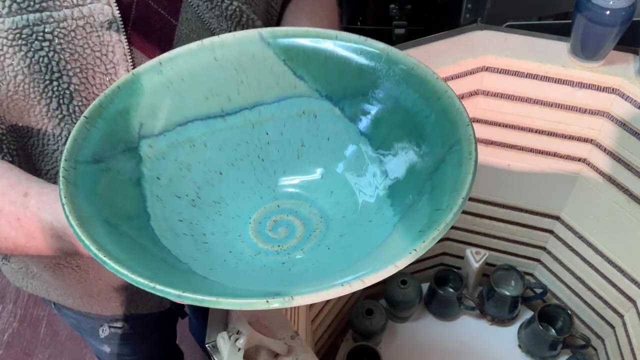 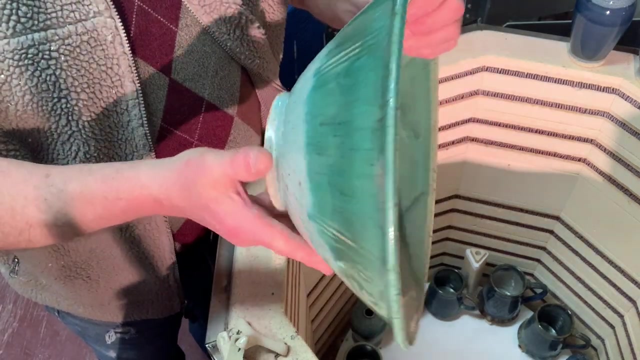 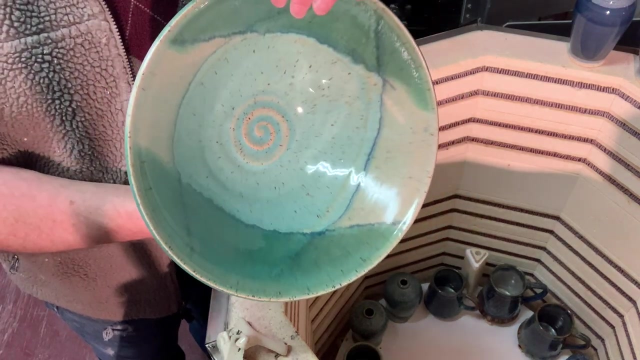 going to do, But I can fire these upside down like I did before and they'd be perfect anyway. This is pretty. the blue, green, copper, red over speckled clay with oatmeal swipe and a green swipe is my yes, yeah, be my green, which is the what I call my dark green, but that's pretty kind of have a fairly 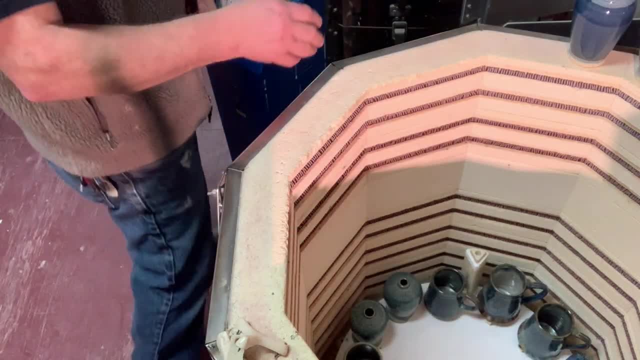 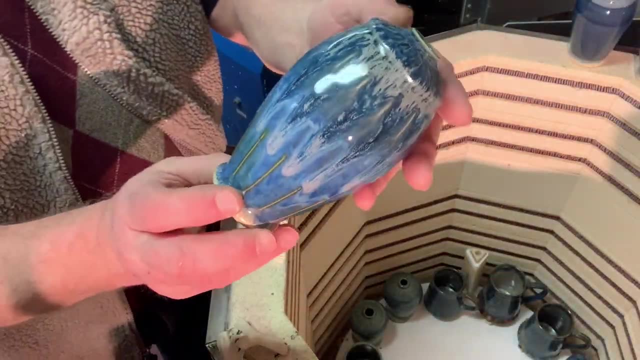 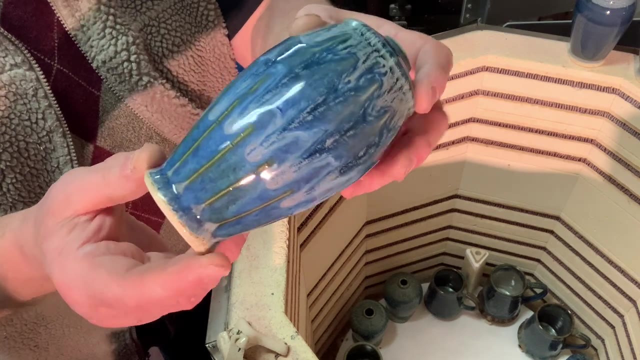 ocean. kind of look on that one. so all three bowls in this firing did well. oh, this is very nice. wow, what did I do here? there's always something that's surprising, but this one I oatmeal glazed over the top and then I think I did a little dark blue. 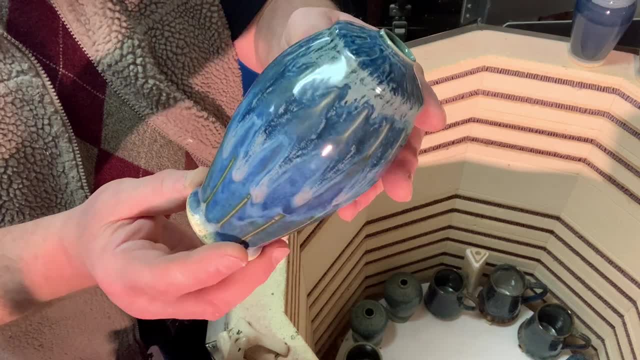 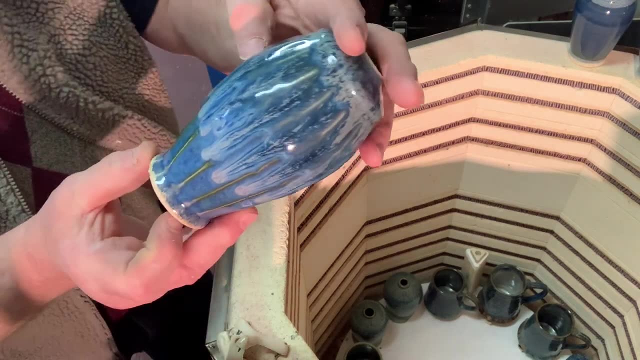 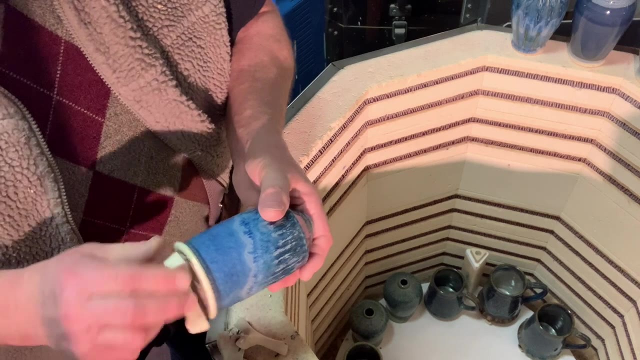 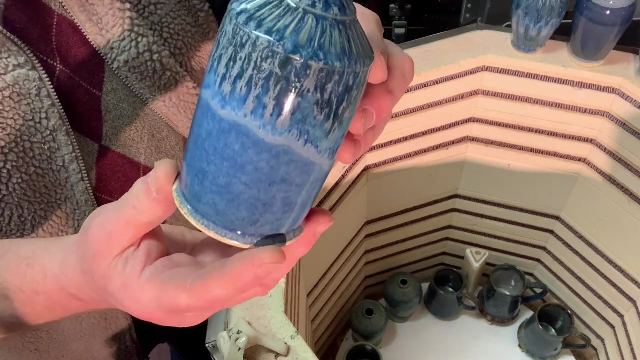 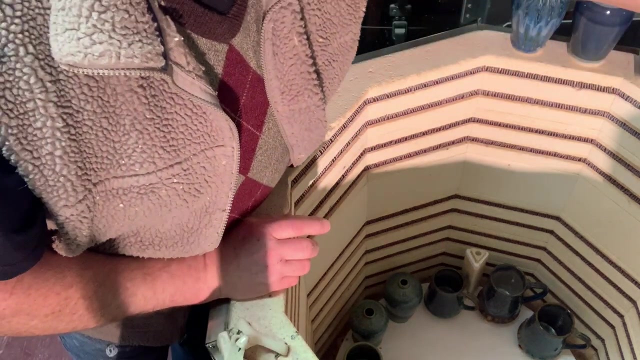 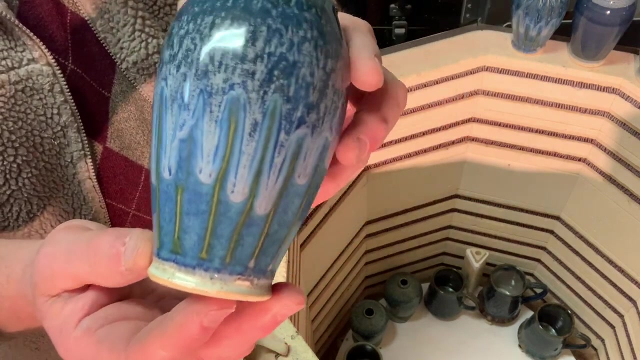 or variegated blue over the top of that. but look at that, that's very pretty. and again, same combination. I've got my oatmeal test on the go at the moment, so we'll be showing results of some new oatmeal glazes. wow, this was very predictable. they all look very much the same. 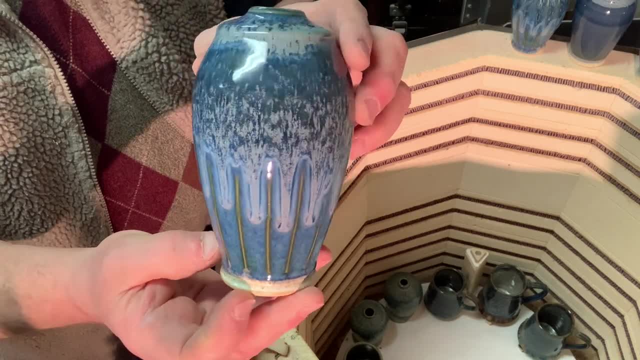 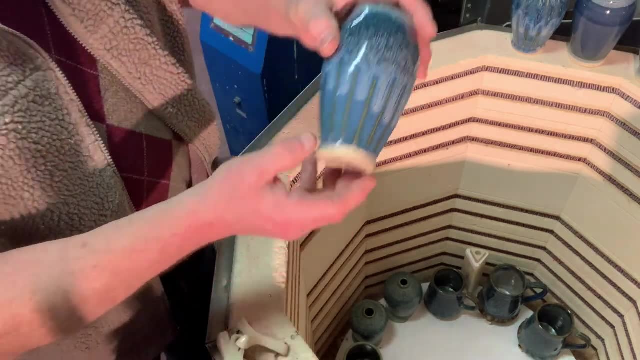 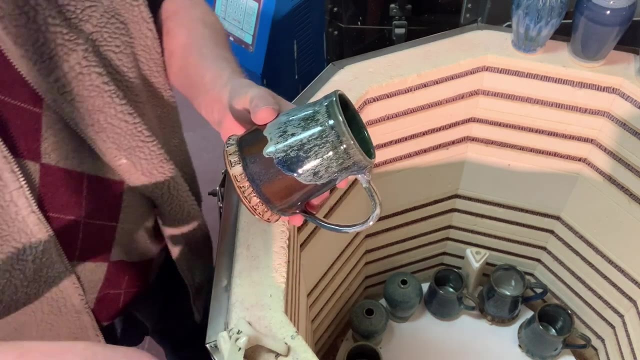 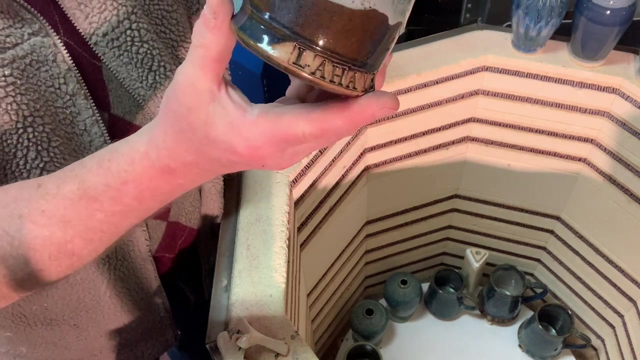 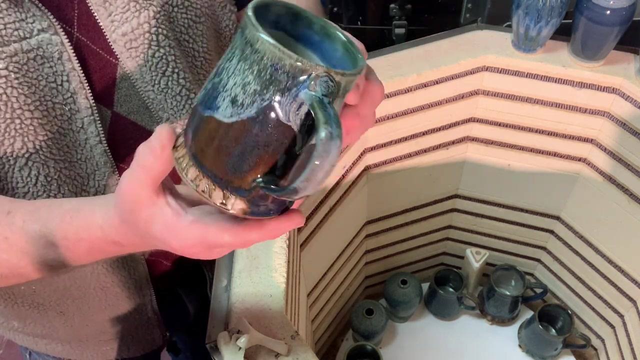 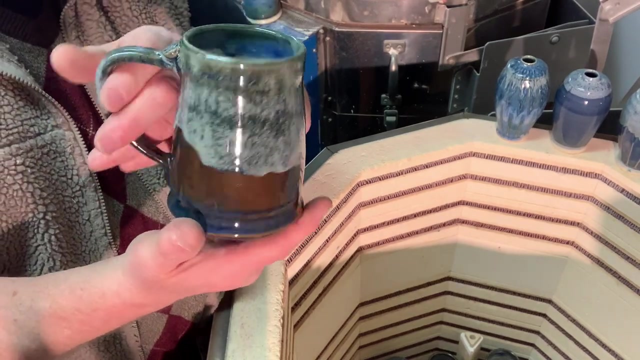 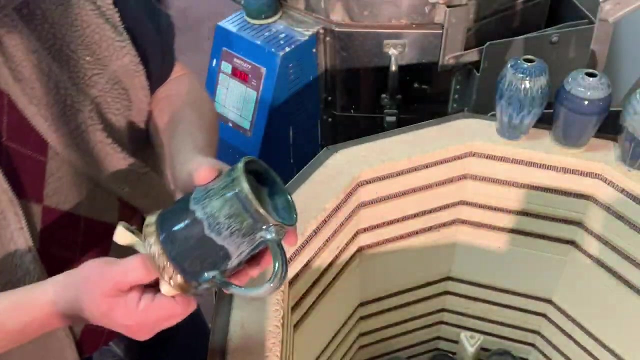 fluted piece, oatmeal and variegated blue over bright blue, running out of space. uh well, this is speckled clay with my oatmeal and I think variegated blue dipped over the top of it. let's lift you up a bit. same again. 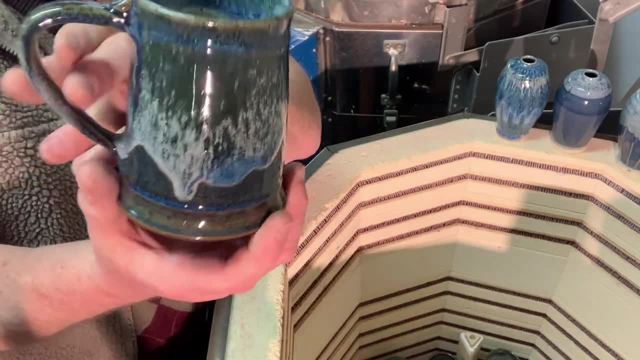 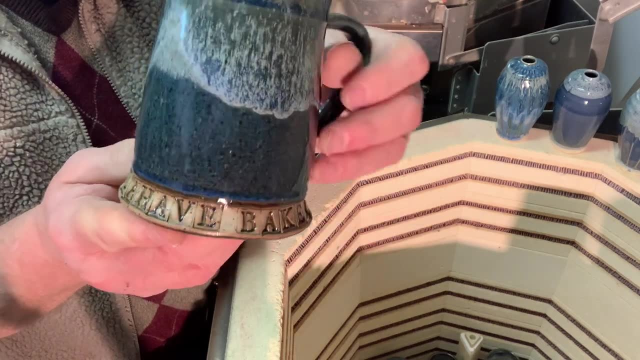 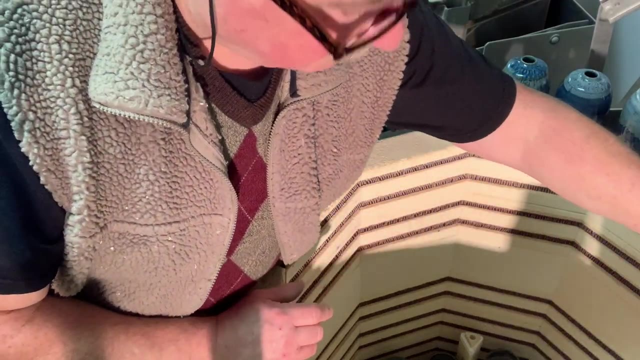 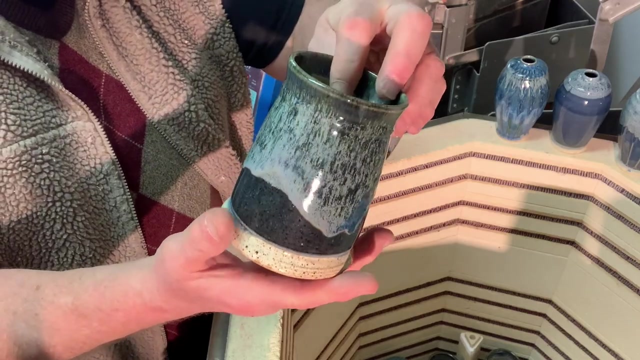 dark. uh, so is it dark blue? no, this is actually. I think it's bright blue. no, it's actually the dark blue. so this is my dark blue with oatmeal and actually the bright blue dipped over the top twice looks like I did this whole layer like this fairly successful combination there. 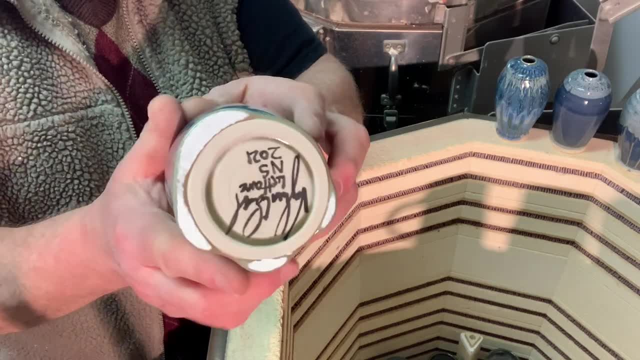 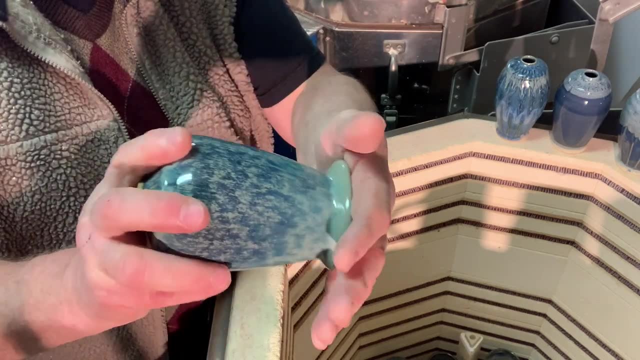 wee. look at that one. that's the variegated blue. but it didn't stick to the kiln shelf. you can see the bat wash on that that gives it. haha, that's funny. you would think that would, because that's a regular kiln shelf with batwash on it is. but it's my original imaging shovel. it was made of iron wheatροpe and there's a 의. 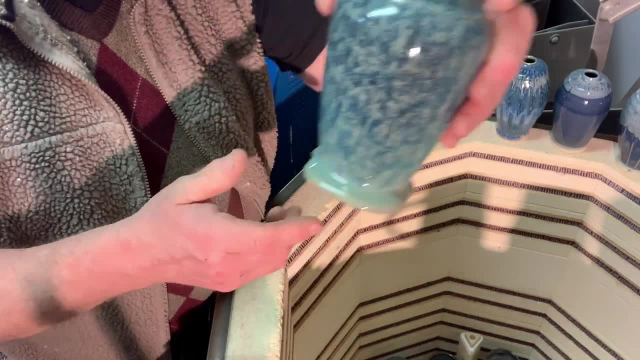 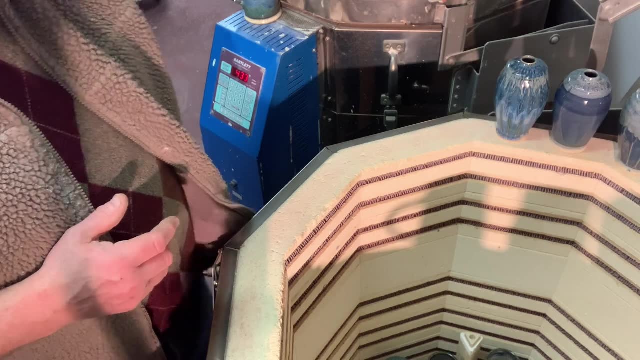 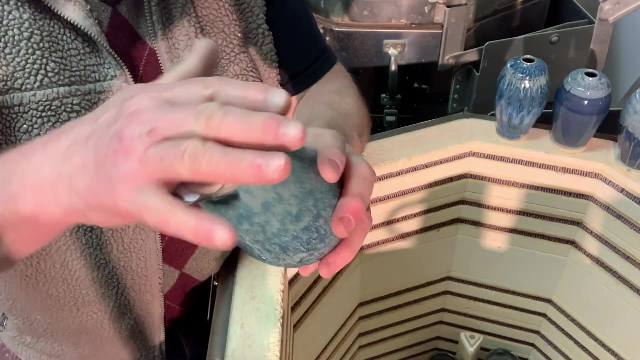 shelf with bat wash on under there. anyway, i think i could leave that. it kind of looks nice. it looks like if it's a lotion dispenser, that the the water is just flowing down over the bottom. happy accidents- same again. just stand it a little bit on the bottom. 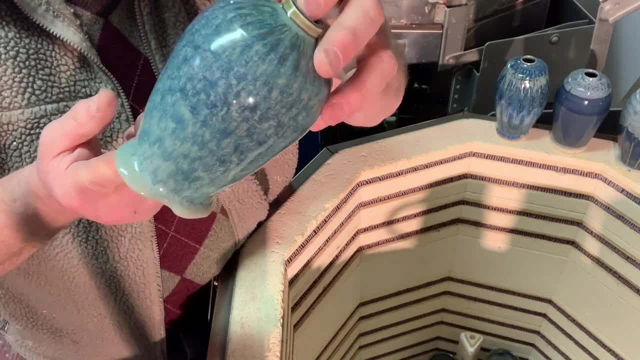 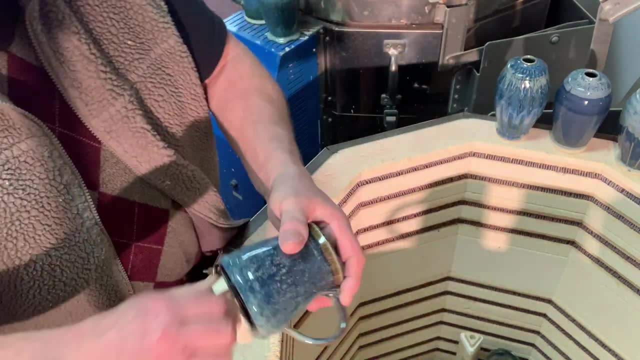 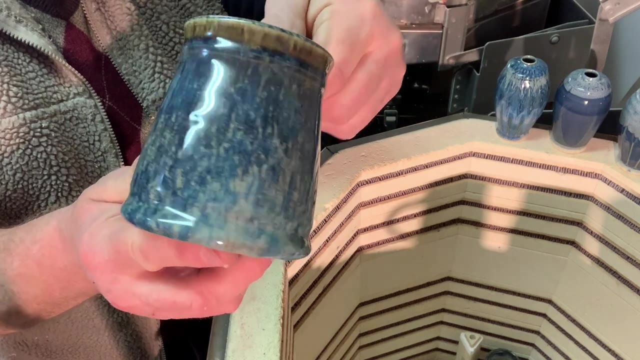 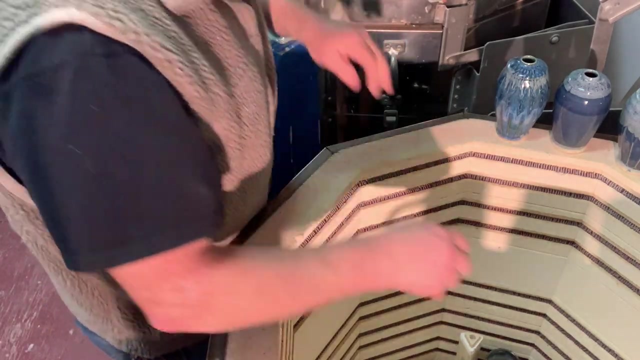 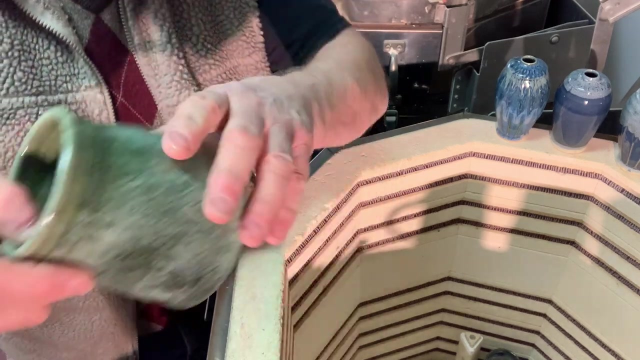 that's odd. it really looks like the feet, since it didn't stick to anything. it's a perfect piece to show the how glazes run. another one of the variegated blue ones, another one of the green ones. so the green ones all have to be fired again. 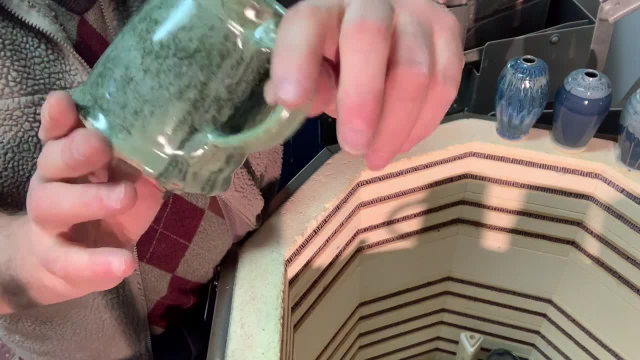 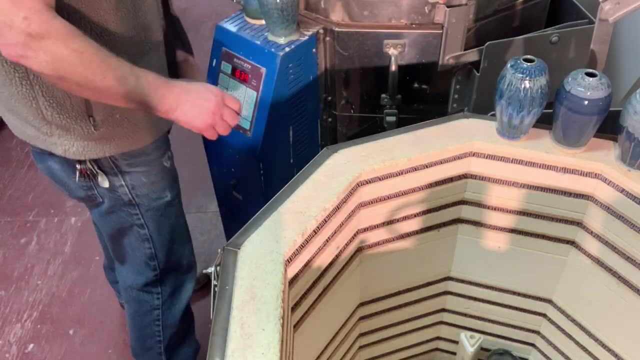 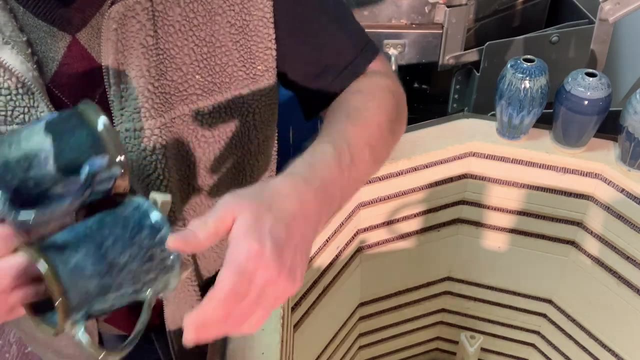 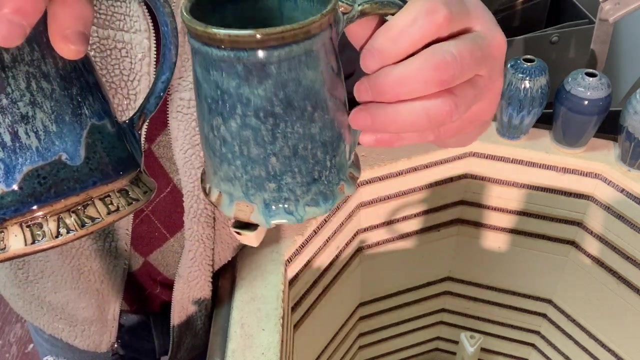 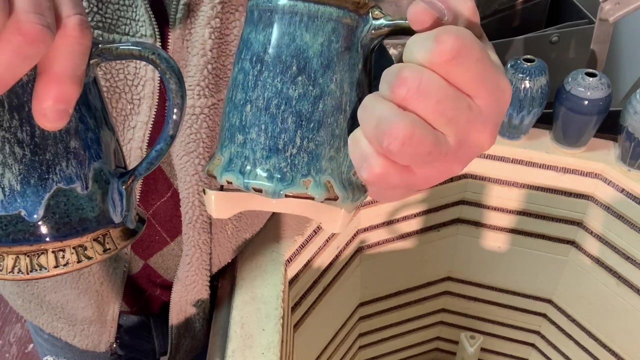 ups, side down. it's just a little bit of a run, but it flattens out if you refire it. and two more, the last two in the firing, and there's the speckle gray, so variegated blue in mastering cone. six glazes definitely runs a lot, so be wary of it. 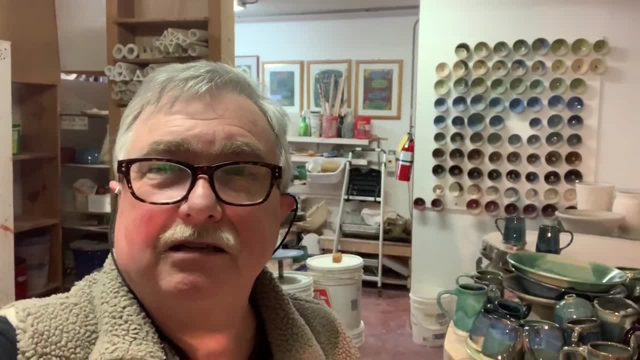 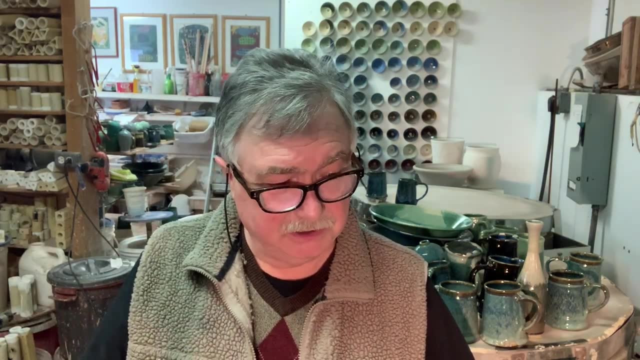 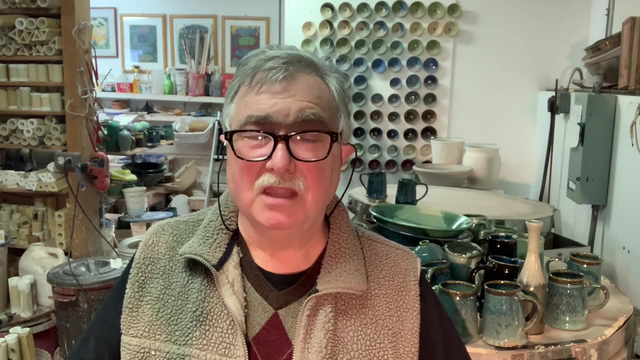 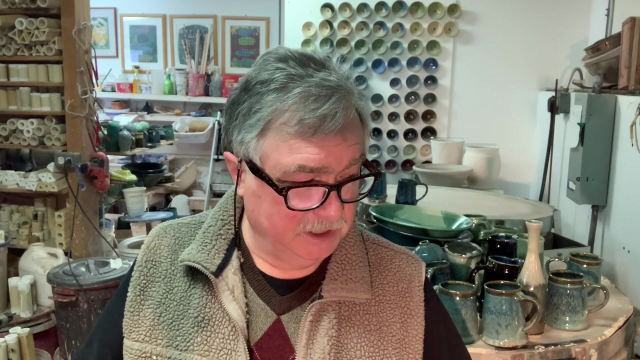 okay, that's the lot there. um, so recap, the green runs. so i'm going to lower the temperature a touch and then i'm going to speed cool the kiln down to 2000 and then i'll slow cool to get the crystals to develop. that's my next firing and i think, uh, the so variegated blue and the green were the ones that 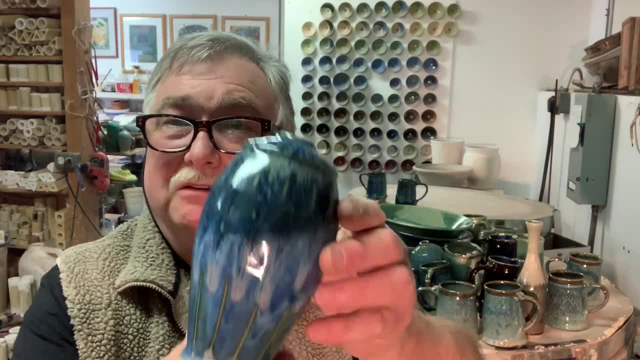 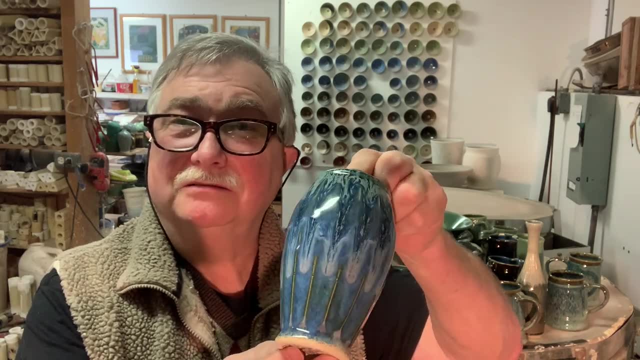 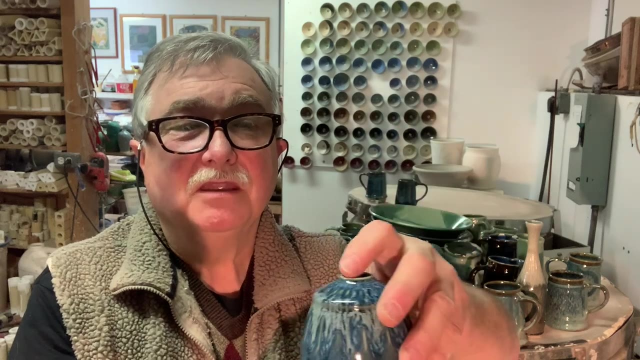 firings, but there's also some amazing results that came out of this firing that I actually didn't expect that I thought it would be interesting: Bright blue with oatmeal and then with variegated blue over the top. Pretty amazing that one. 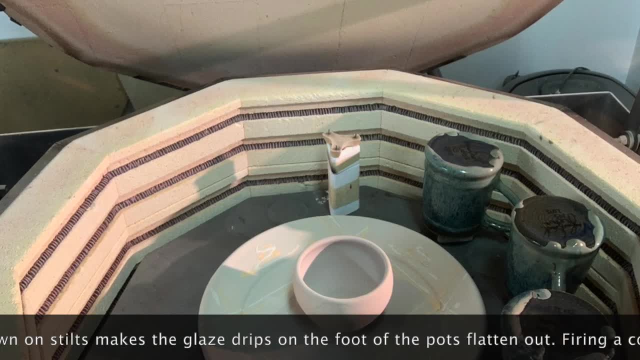 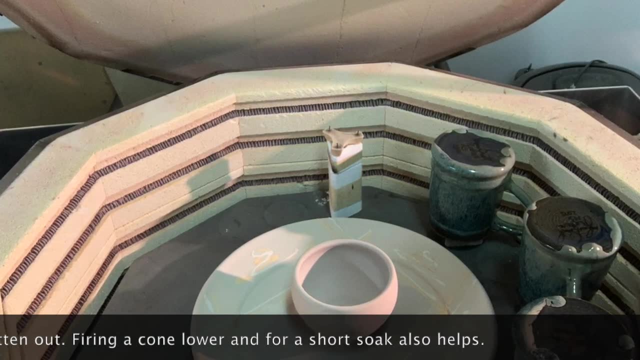 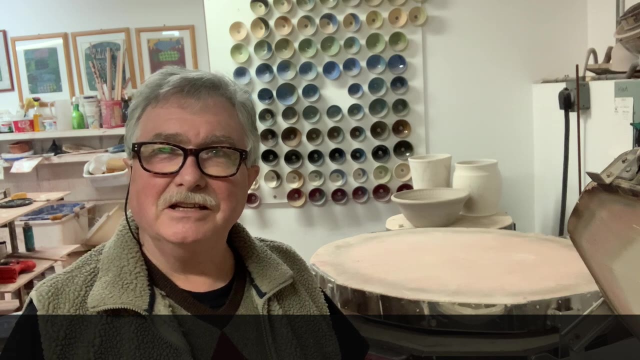 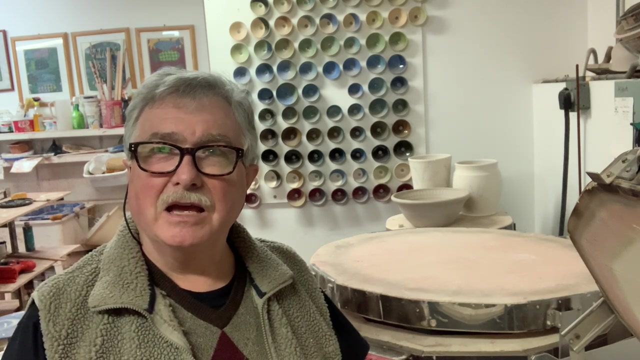 Hi, this is The Other Kiln. It's a clear glaze Cone 6,. so transparent glaze and hand-painted underglaze painting, just like the video I did with the mugs recently. So I'm going to show you how to do that. So I'm going to show you how to do that. 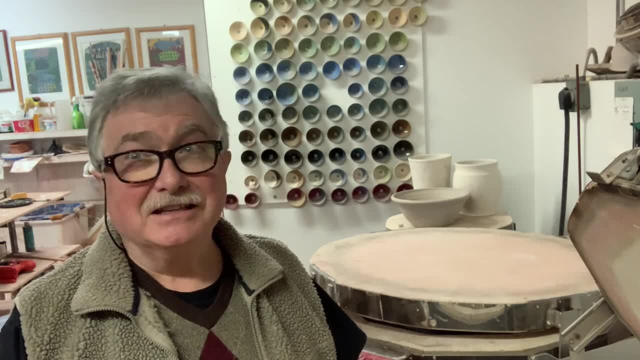 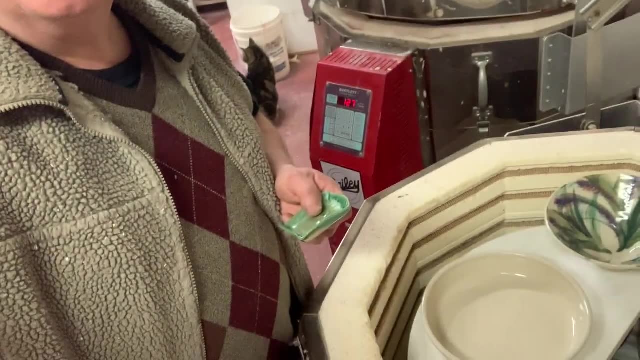 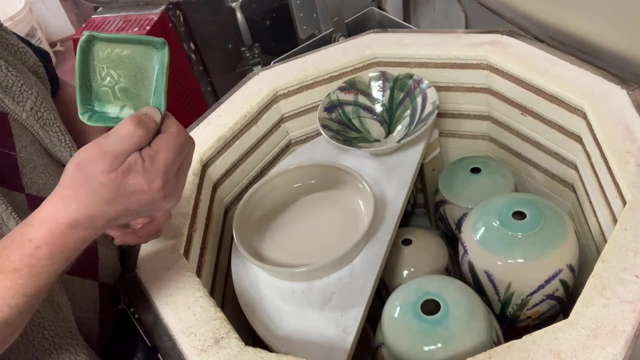 But larger pieces obviously. Now it's exciting, Not what I was just describing: Kiln filler. There we go. This was a little kiln filler. I had room for it. It's nice to have a bunch of these. You just, you know, put your rings in or a little bit of relish or something. but 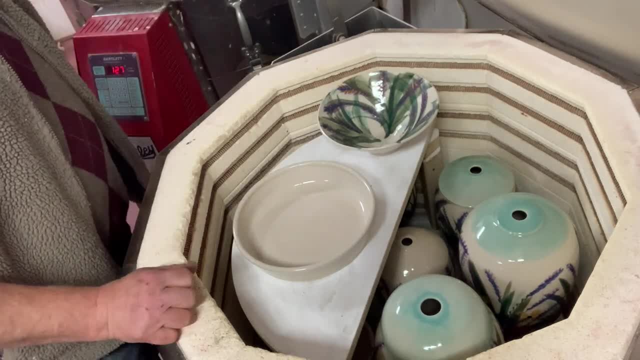 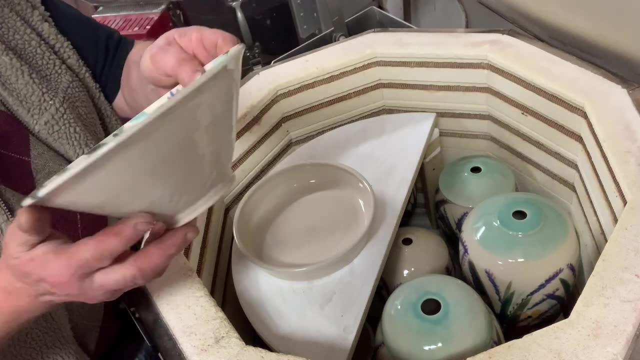 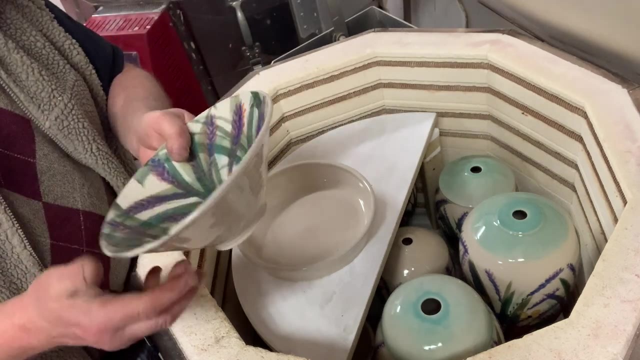 we make a bunch of these just to go in the kiln. They take up no space and so they can just fill up a space. This is my Cone 6. Clear glaze: I've developed it. It does not craze. Having said that, you know crazing can happen. 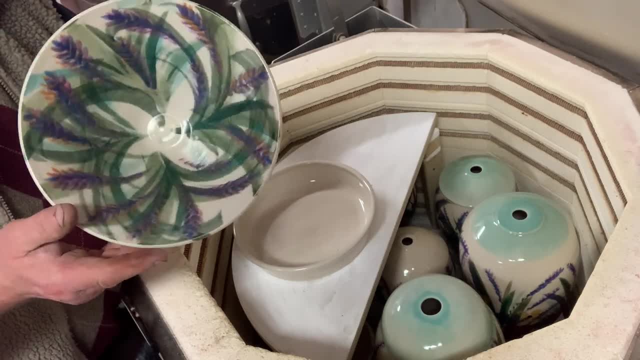 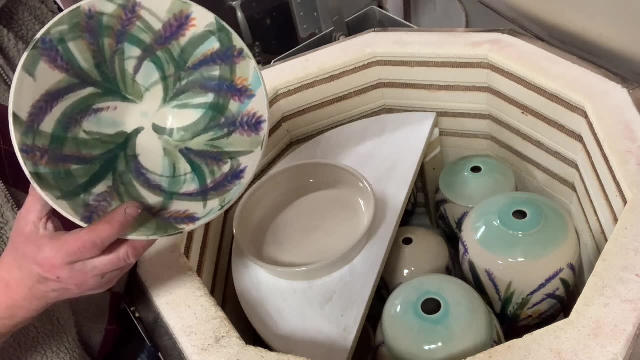 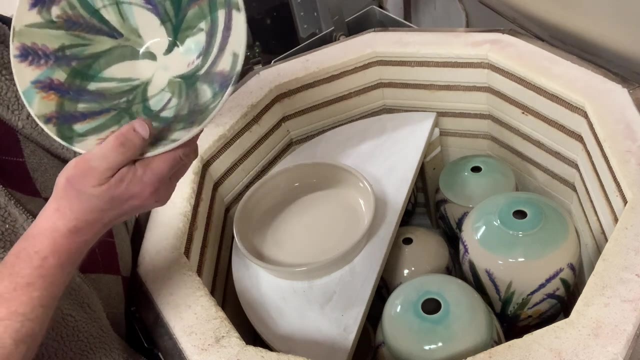 years later, so you can never guarantee it. There you go. This is just like those mugs I painted, but I did a series of bowls and they're all different. This, as you can see, is about eight inches across. I don't know if you call these lupins or what, but they're. 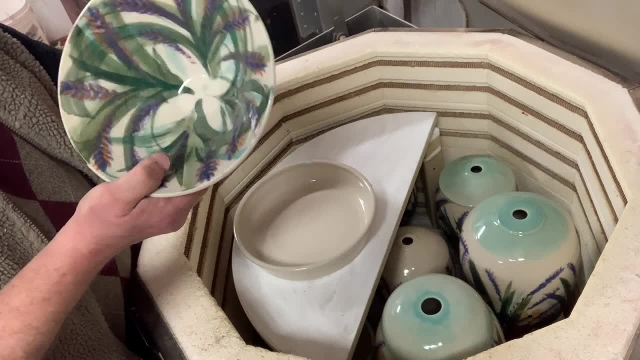 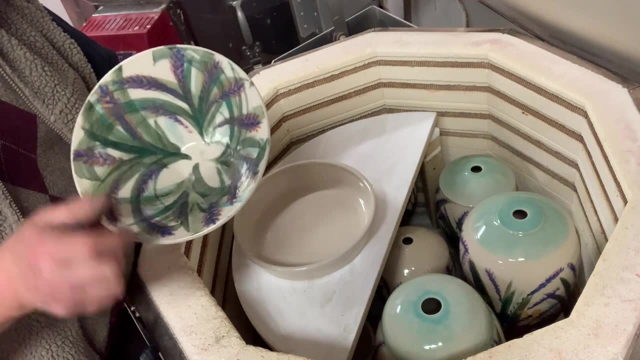 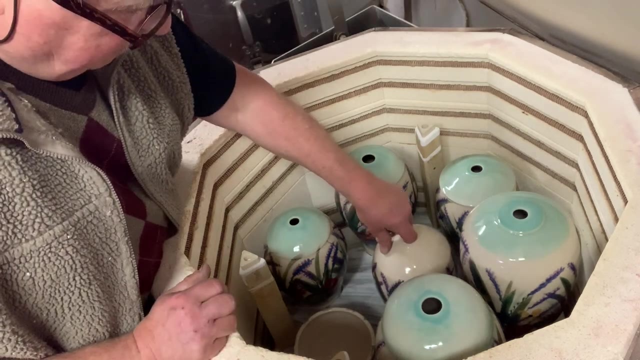 they could even be um lavender. i mean, i just make these flowers up. they're done with the brushes, the japanese style brushes, and i kind of let the brush make its mark when i'm painting. so if they're very fluid, okay. this is all experimental, so we do not know if they work. 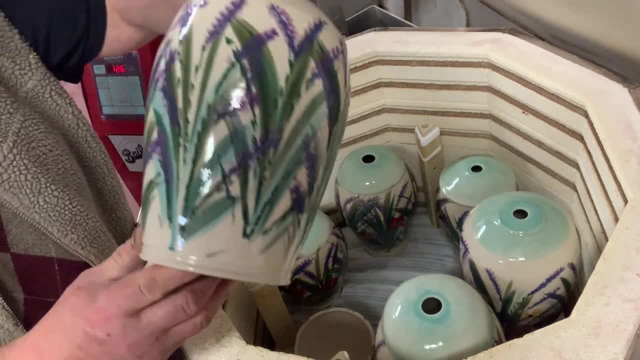 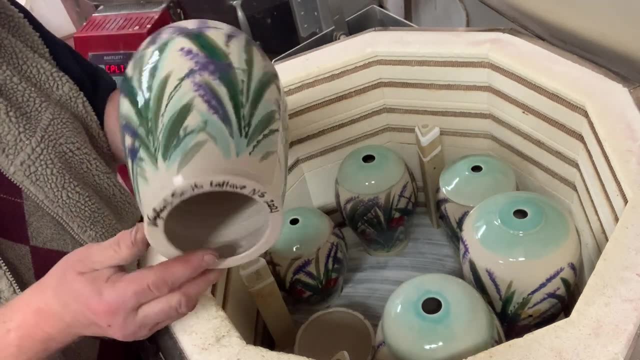 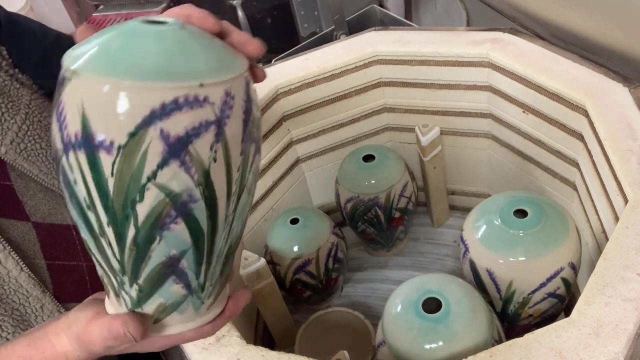 well or not. um, that one is a lamp base, so i threw it, just like i did my lotion pumps and vases in front. um, i also used my blue, green, copper red on the top, um, just to kind of accent, because i had that same sort of green in there, but also it kind of makes you think of the sky. 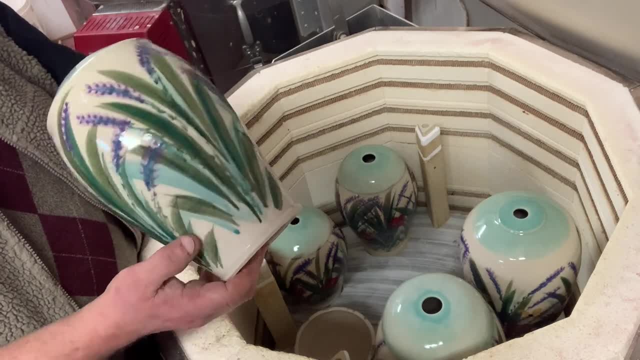 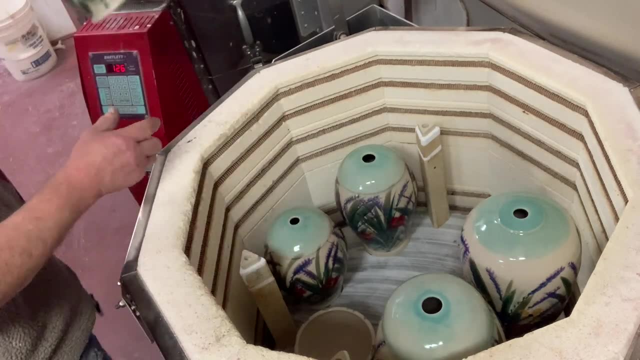 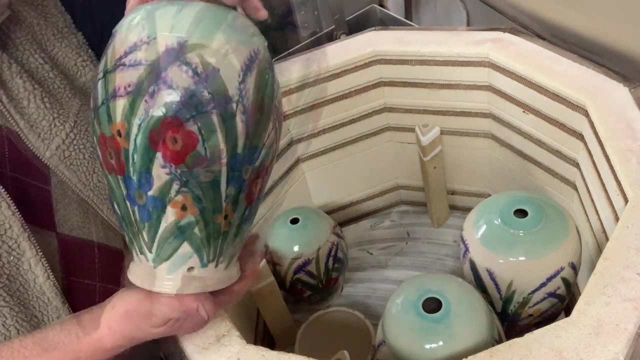 so these should be nice when i get them all fitted with the electrics. they sell lamp kits at bailey pottery supply. i've always bought those because it all comes complete. okay, now i went more elaborate. you know i i my stencil work that i've just shown in a video is very popular. 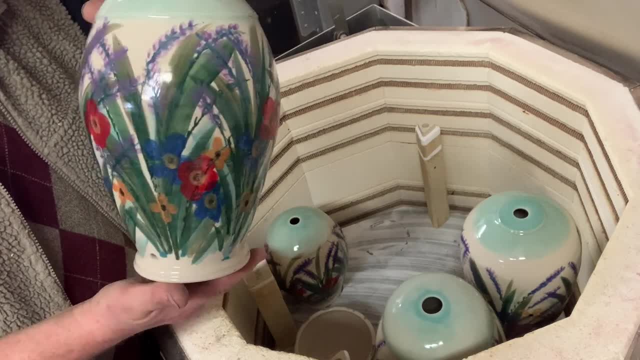 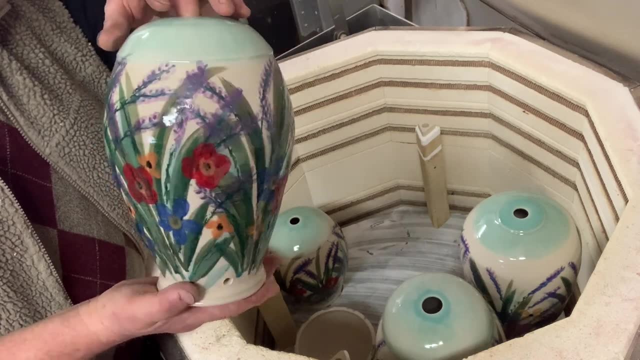 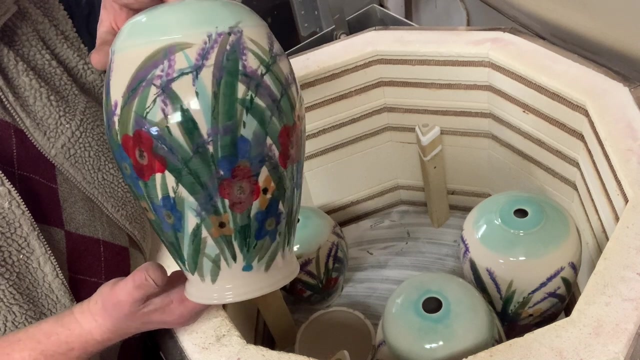 and i kind of i've done it for 40 years nearly, so i'm enjoying doing these. they're a lot more loose and the japanese brush that i have- i've got so many of those brushes and they're all big, small, different sizes, different points and- and i'll demonstrate- maybe some bigger pieces like this, because i've got four large ones going- 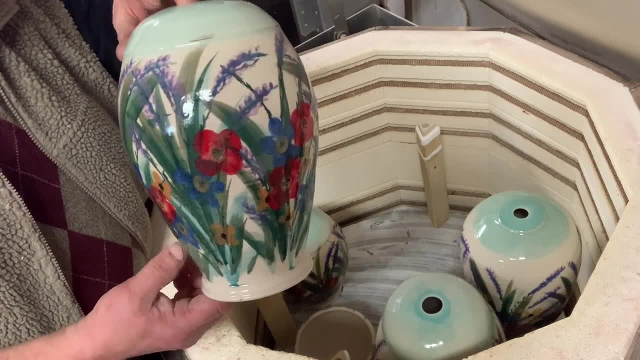 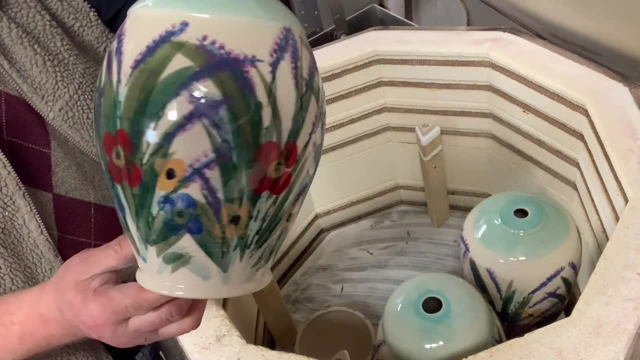 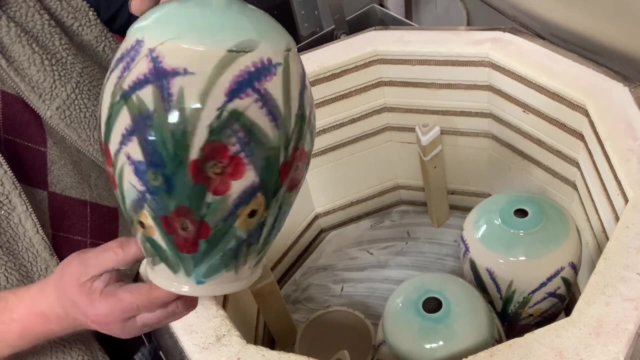 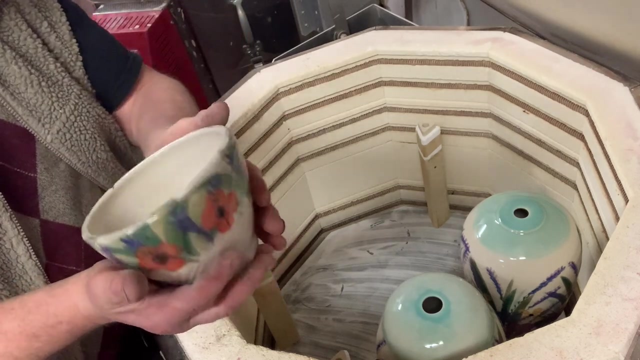 to the kiln too. um but um, these are doing pretty nice as experimental pieces, so another one of those make a nice pair. if anybody's interested in any of these pieces, just give me a shout, email or phone. it's at the end of the video. a nice little bit. you know, soup ball a bit heavier. 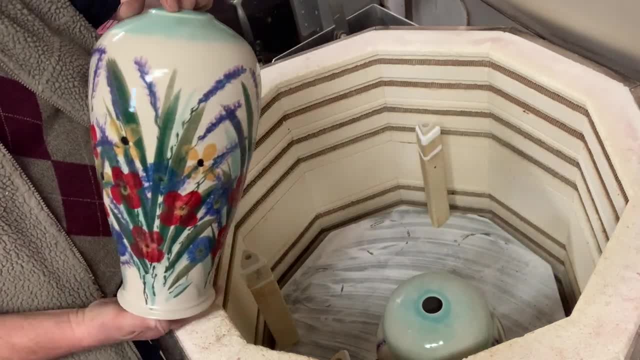 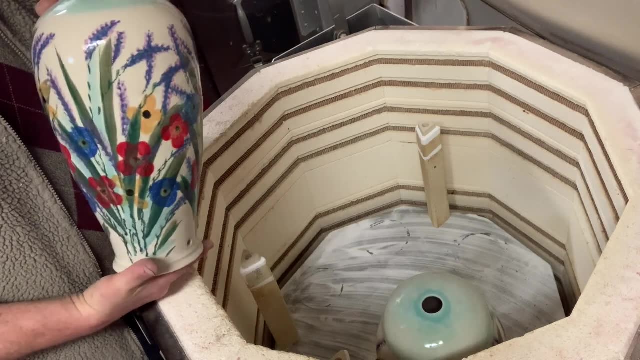 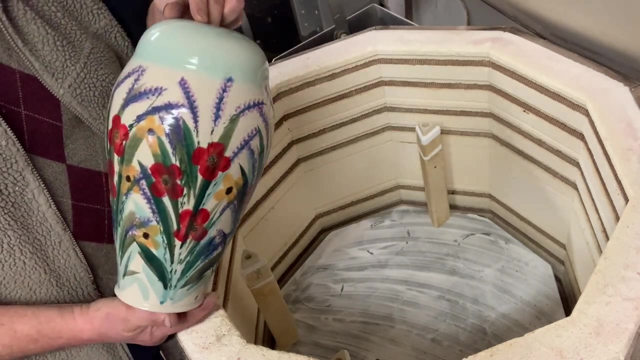 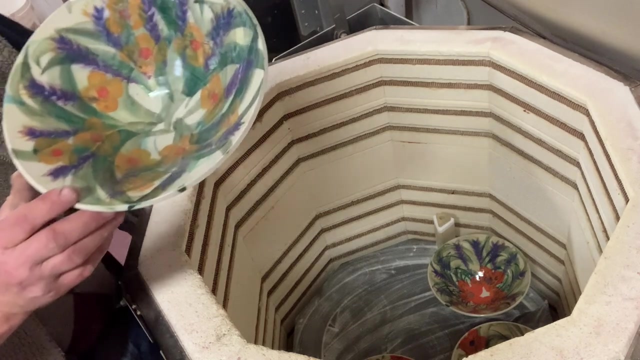 bigger lamp base. sometimes i make a bottom for these as well, so i might do that, because that makes them even larger. but let me know what you think. these are all brand new for me. a bunch, somebody, okay. what do we have? all right, what do you think? am i on a wild goose chase? 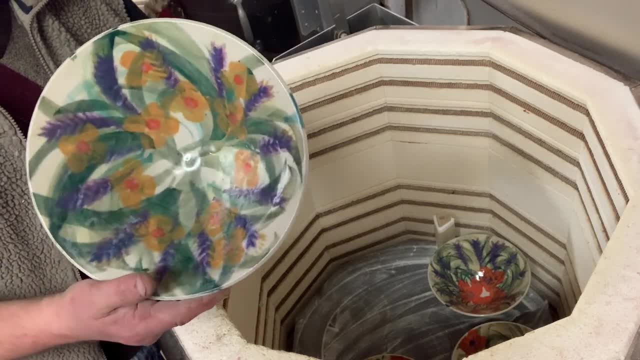 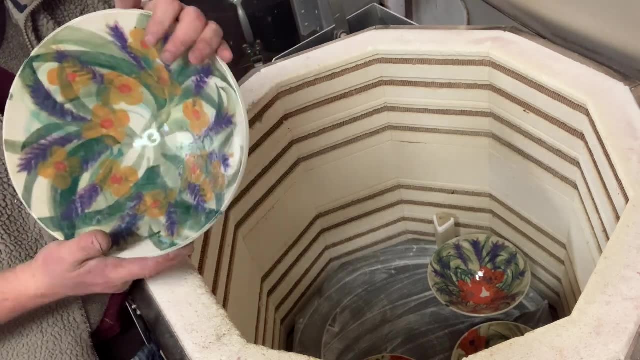 okay, all right. all right, wild goose chase here. i enjoyed doing them. they've never been in my showroom. these are brand new pieces. the mugs are selling really well. i've got two styles of the mugs in the showroom now and they're doing really well. 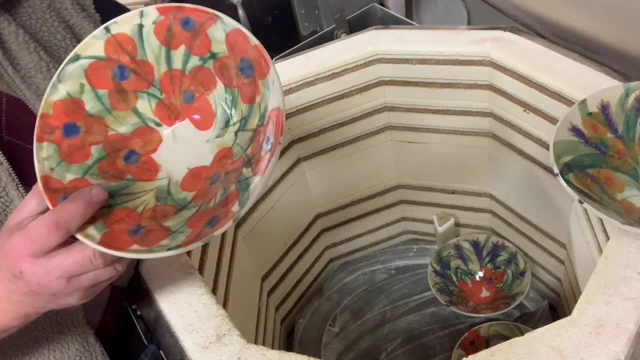 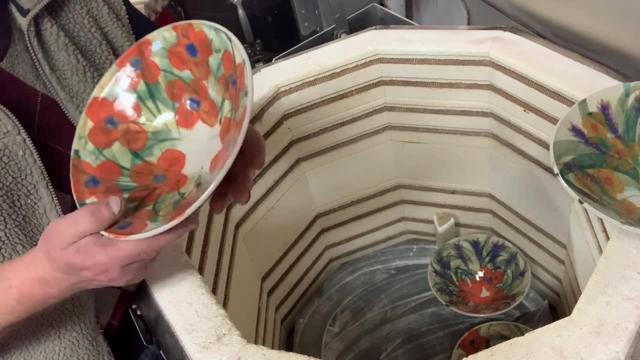 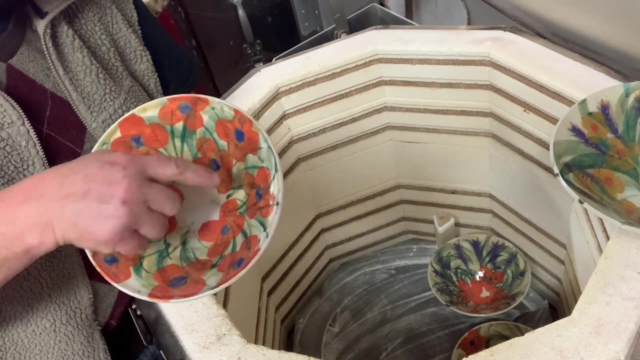 but here we've got some balls and i'm playing there you go poppies. so- and this is i can show you, this is the paint brush. so this is the paint brush. if i place it down and just kind of went like that, it made that shape. 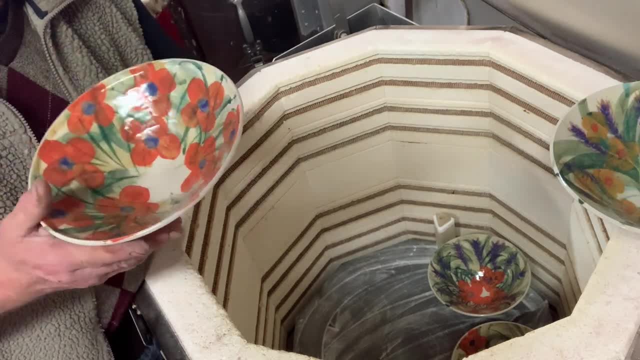 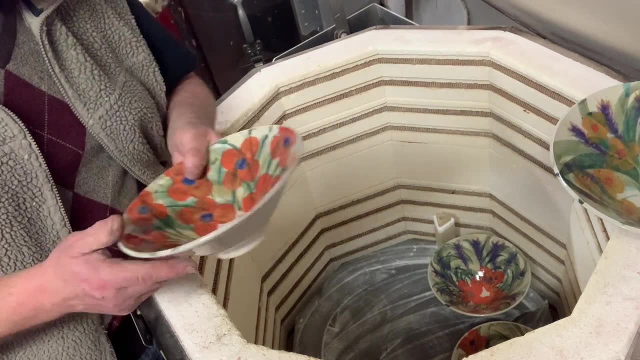 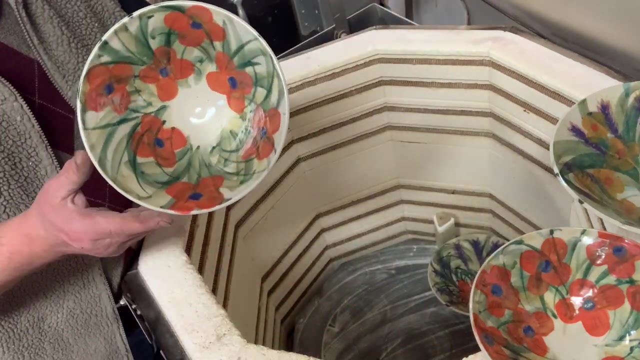 so i'm really allowing the paint brushes that i have to kind of dictate a little bit what i'm doing. but that's part of it. i enjoy the natural, quick, spontaneous part of it. there's another one. there is yellow in these too, but the yellow has faded out. 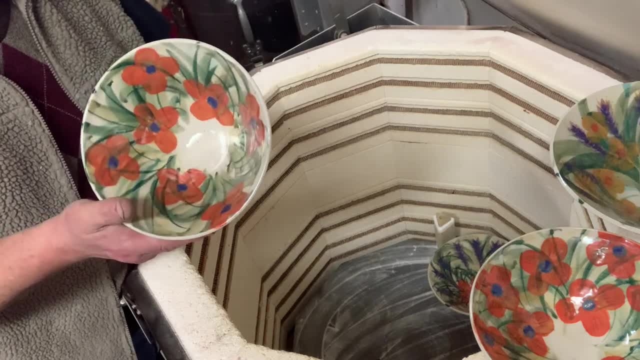 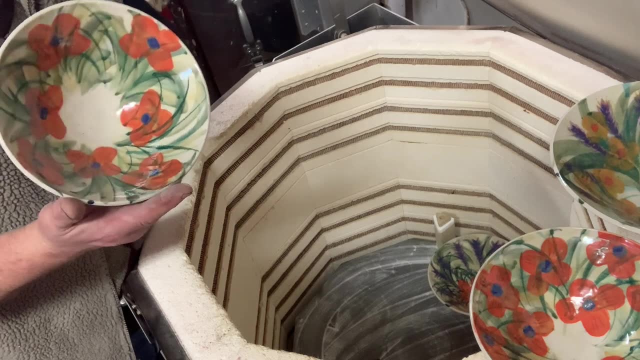 i don't know what that means, whether it's this needs to have a much thicker coat, i guess. but you'll see. you can see a little bit of yellow, i hope, in there, but it has not shown up as far as the intensity of the red. so maybe the red is a bit too intense and 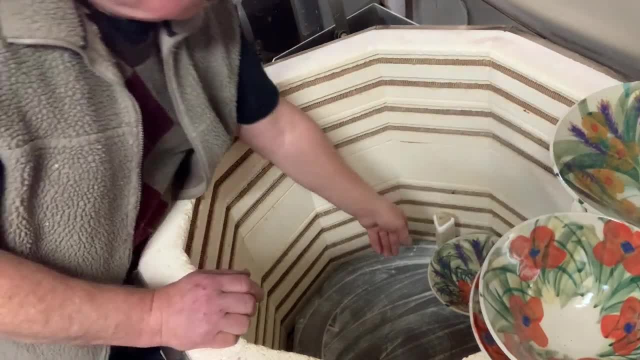 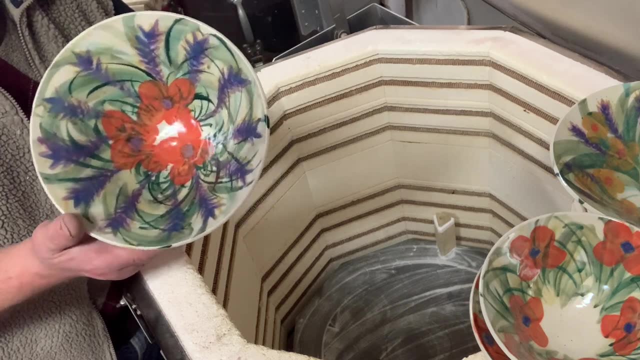 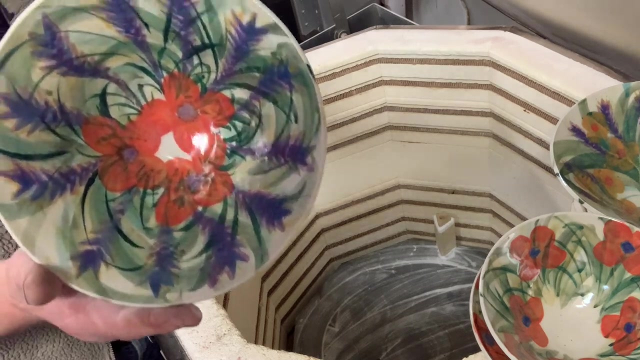 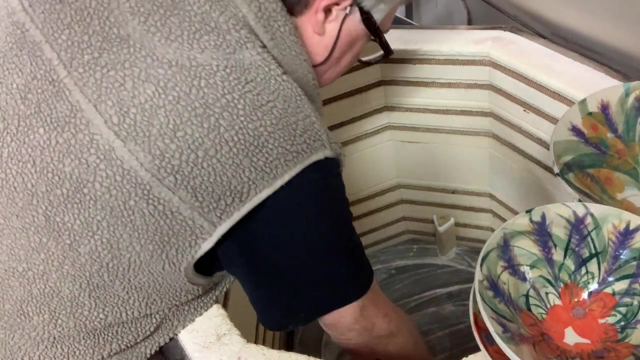 the yellow steps back a little bit, and then here's the purple and the red again. i think the red's a bit too intense. maybe the purple is really nice and there is some yellow in the purple. let's see what we have. down deep there's two large balls, so i've got one of them out there already. 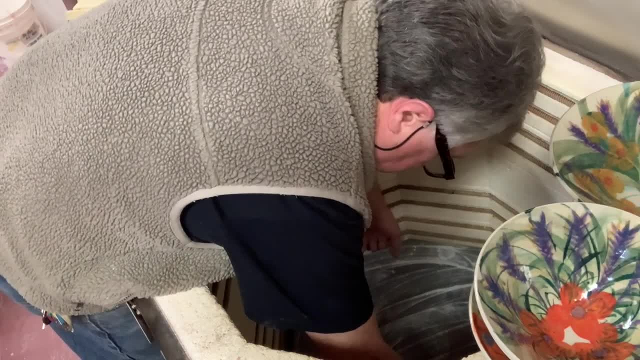 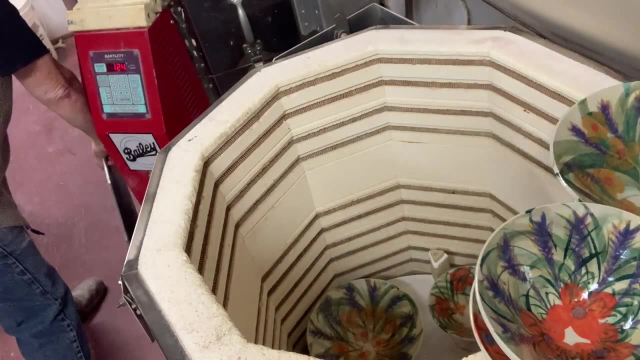 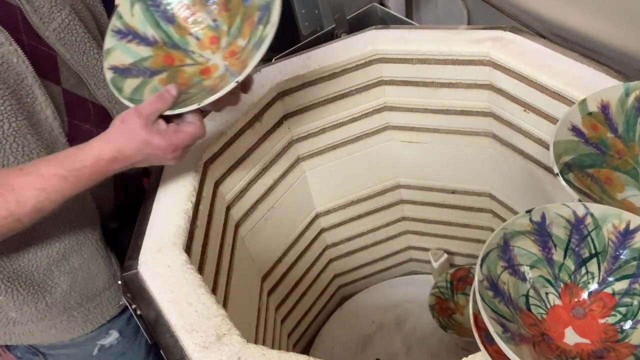 it's good to experiment when we we're doing pottery. for years, i just, you know, like to keep changing things up a little bit. yeah, these are pretty much like the ones you just saw, i think. so both of the big balls are very much the same, like this. 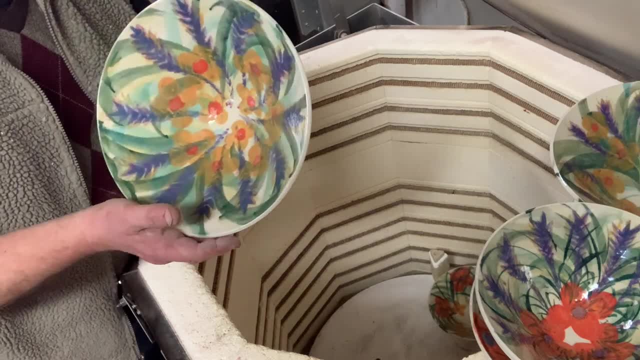 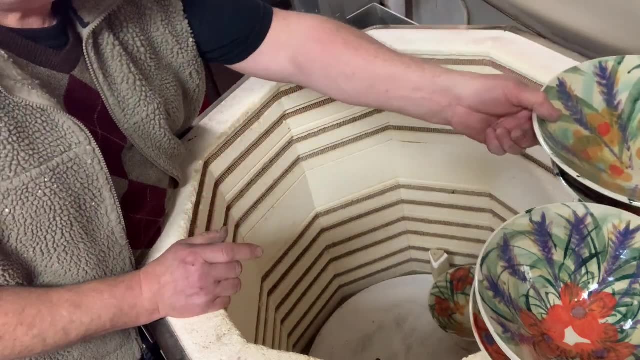 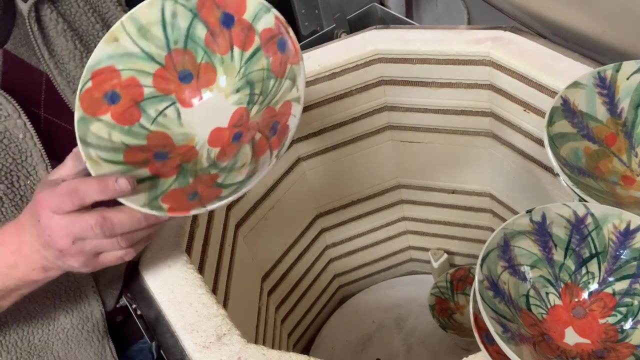 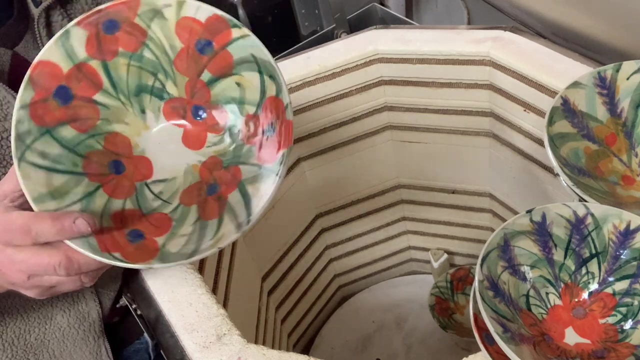 they're still a little hot to lift up. it says 122 degrees in the kiln pyrometer but this feels a bit hotter than that. but it was on the bottom. there's one without the, the flower, the leaf. i like the leaf direction, you know, with the sweeping motion of the paintbrush. 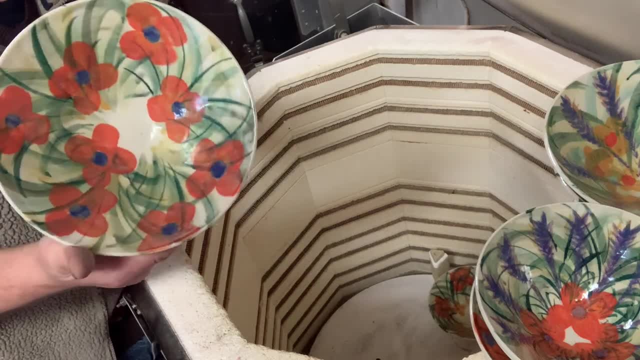 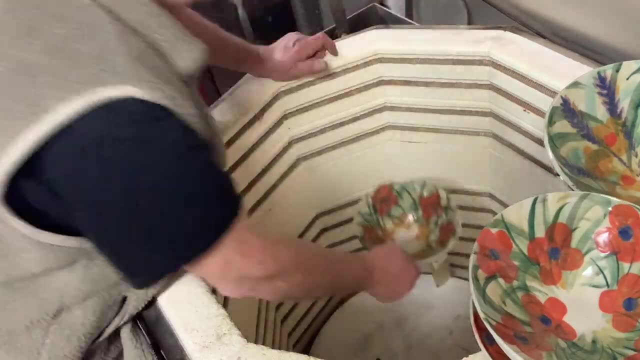 but i think i have to change the flowers a little bit. maybe the red flowers are just too much. it's interesting because you don't know when you paint these underglazes. a lot of them say they need three coats and others are supposed to be transparent, some of them. 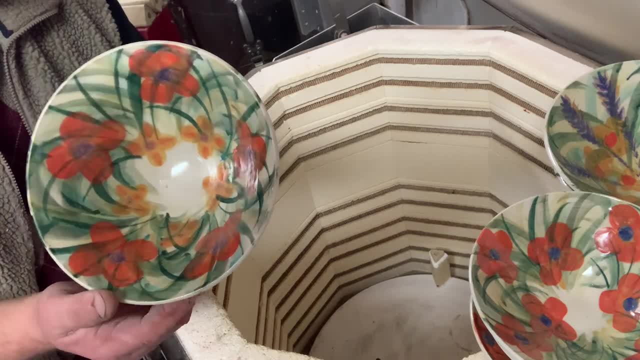 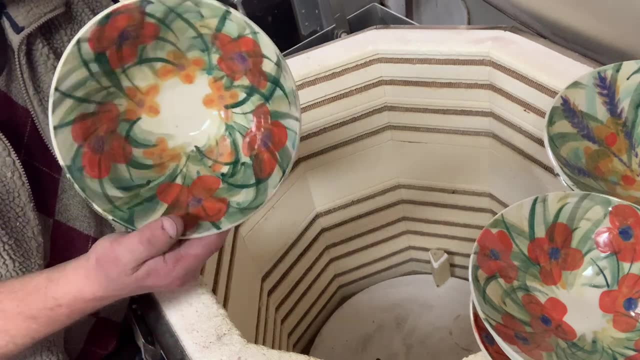 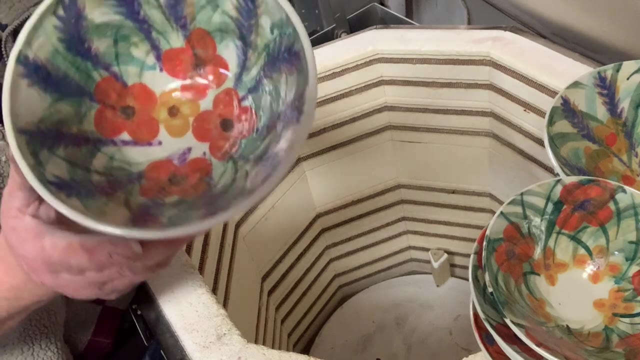 oh, there's some new yellow and orange flowers underneath there as well, so, and that yellow showed up at least, but most of the yellow has faded out. i just ordered some new underglazes, and there's another little mixture of all of it: yellow, some reds. 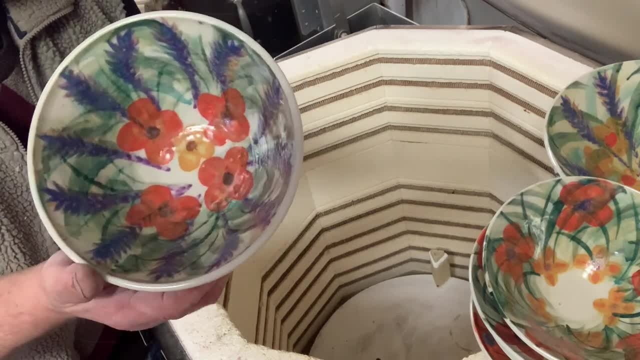 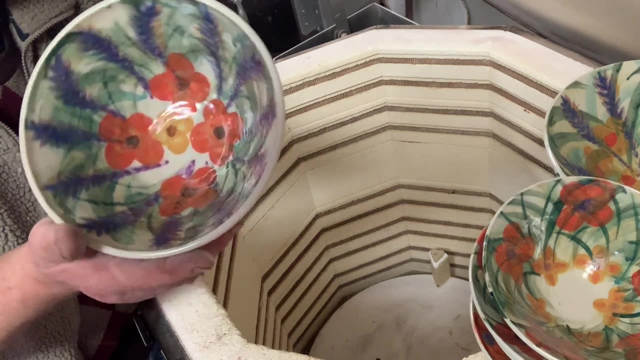 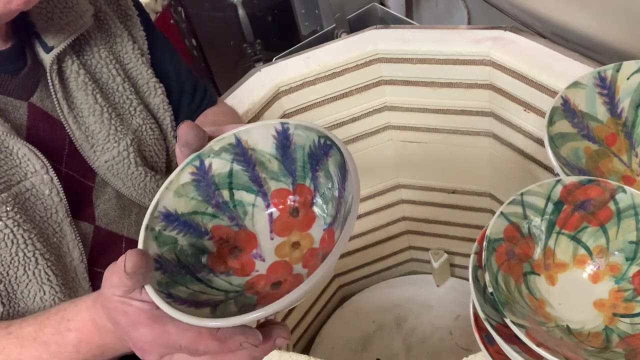 first impressions on my part. you can make comments and let me know. is the reds a bit too strong? hey, but maybe people like red. i like the lupin type flowers and the yellow ones. i wish i'd done a little bit more in the yellow. i don't think that was actually red. maybe that was the deep neon orange that they had. 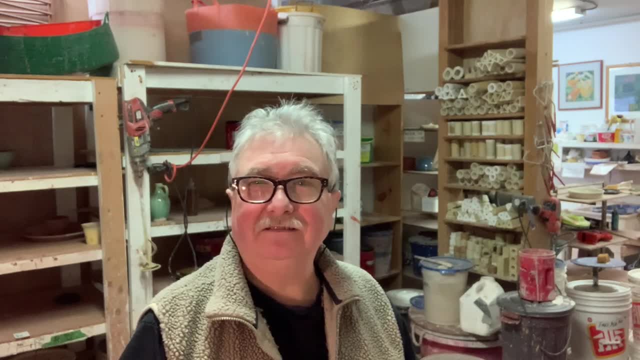 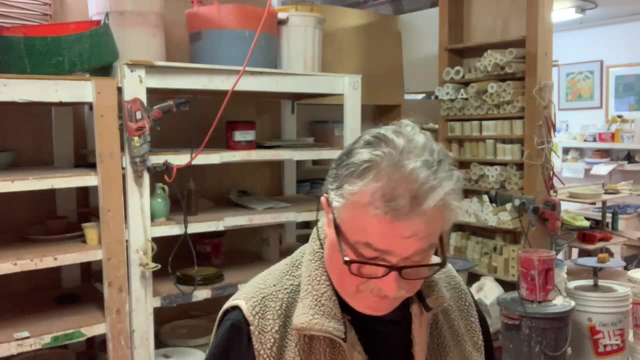 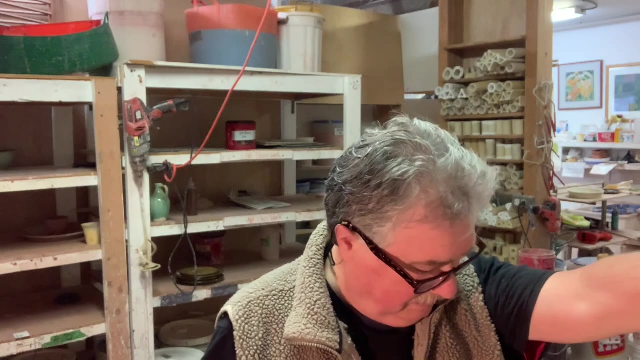 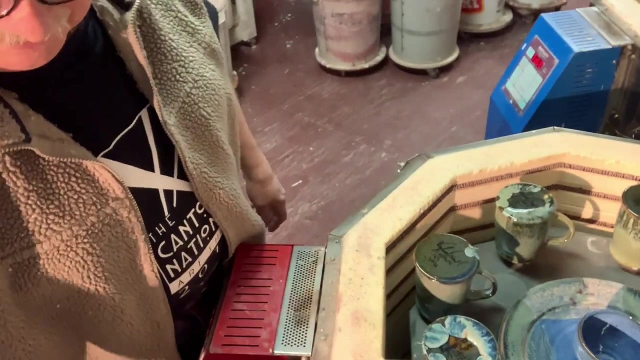 okay, all those um runs and melts and sticks and stones, whatever, um, i've refired them. let's see, surprise, surprise, what's the temperature? 120, okay to open. all right, so this is what you do if you get all these runs. let's get you all dressed up a little bit better. 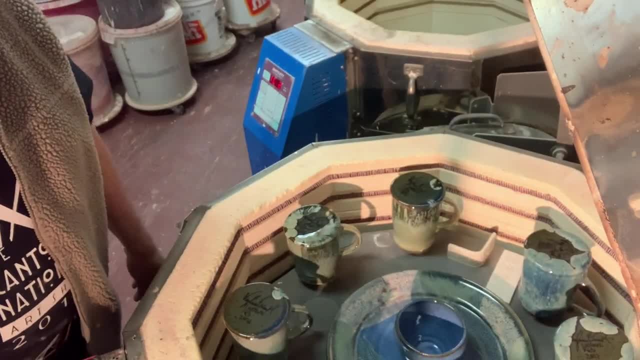 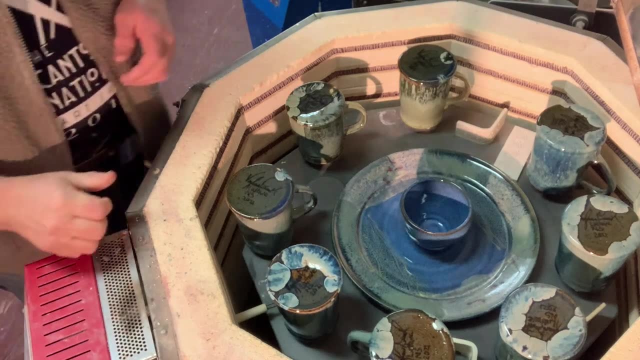 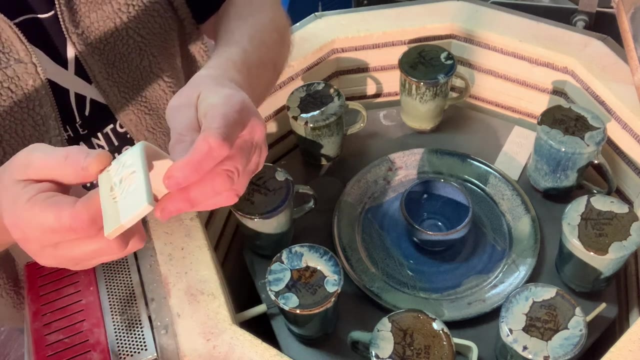 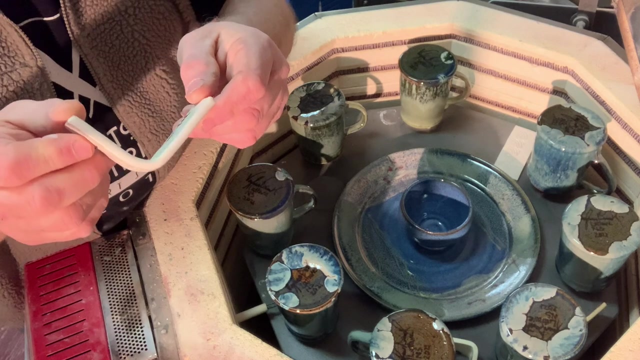 i got a light one, so i'm trying not to block the light too. um, okay, so i refied. i've got lots of things in here. um, so, oatmeal tests. wow, what did this one worked? which one is this? this is david lee and i, so these are two of the same writingυχ that i used to use in 1973. 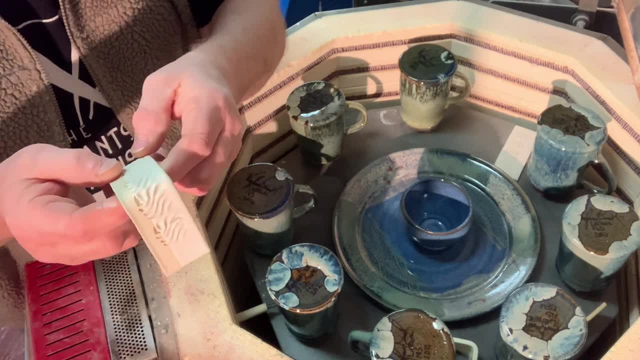 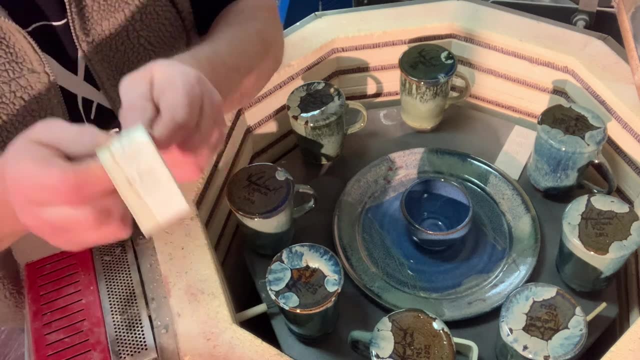 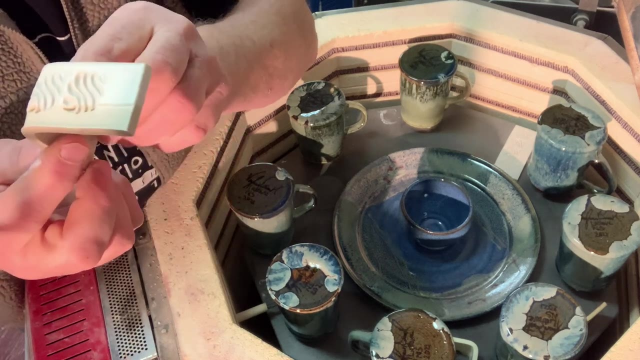 and i've changed it so that it will fight a cone six from cone eight. oh wow, it is. and this does not use any tin or any titanium in it. and look how white it is and it's silky, shiny. first test. i'm not even going to guess yet, because they're all first test. they're not burst. 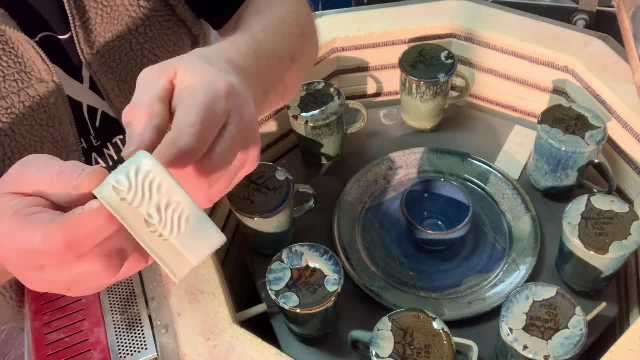 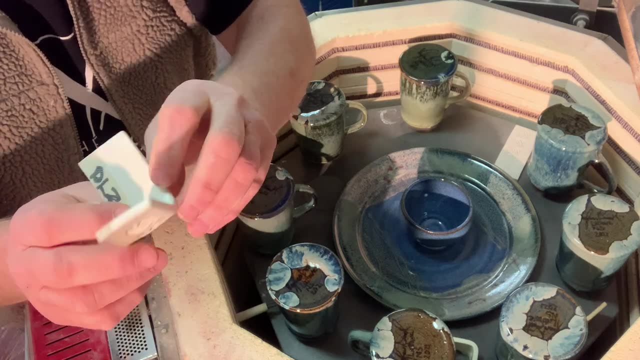 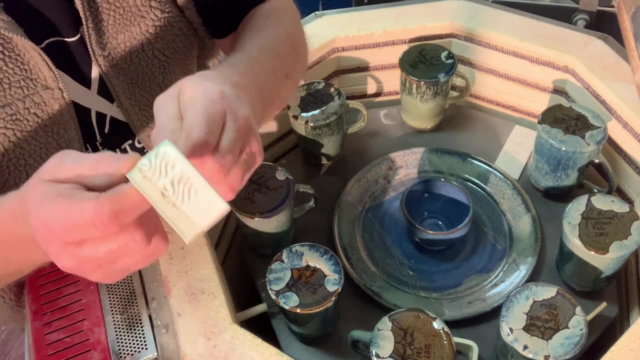 going to change this. this worked perfectly. this is what I remember. I changed it to a. I just changed the feldspars, basically, oh wow, I'll have to look at the recipe, but this is great, all right. my oatmeal has tin in it- seven percent- and that's expensive. this has no tin in it and it's white. 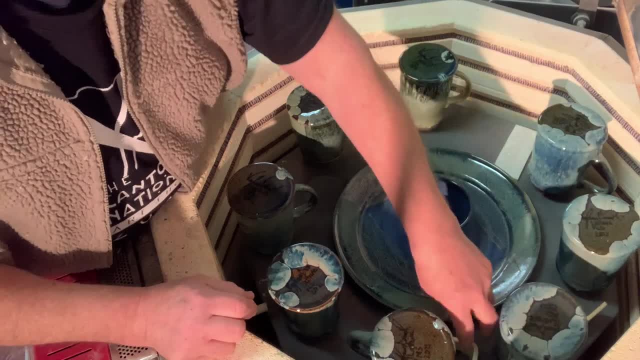 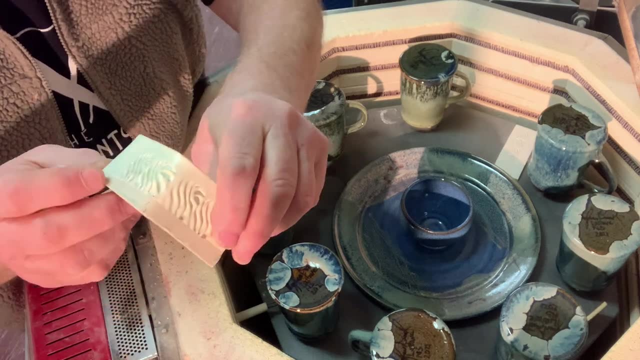 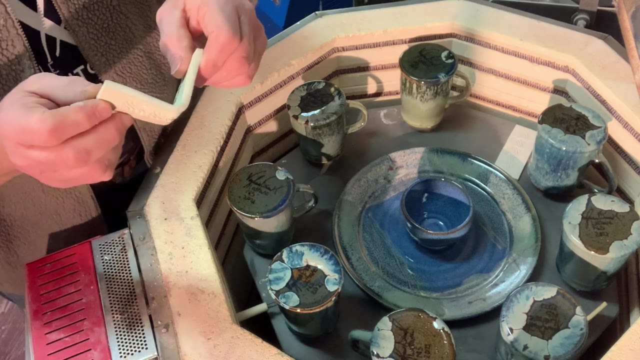 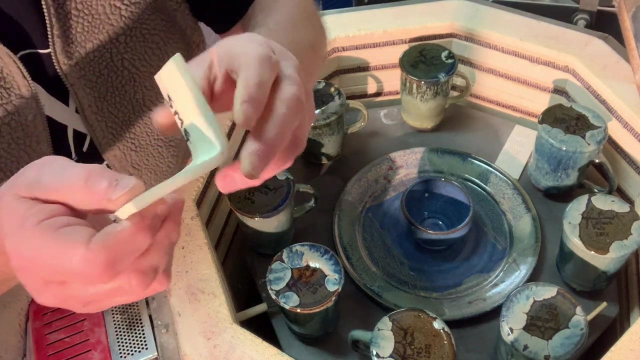 so this is great. wow, this one's great too. look at that. it's got a slight creaminess, more yellow, and this is SMG. which one was that? um, I'll have to look at my buckets. SMG satin matte glaze. I got this one and modified it out of- uh, I think it was John Britt's book. I'll have to look it up in my recipe. 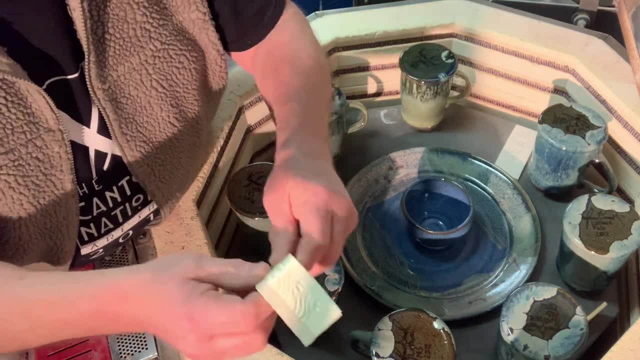 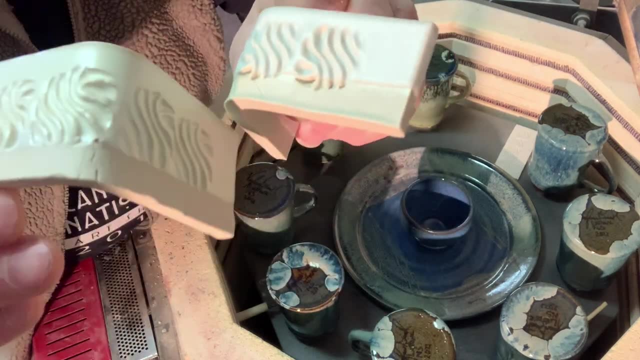 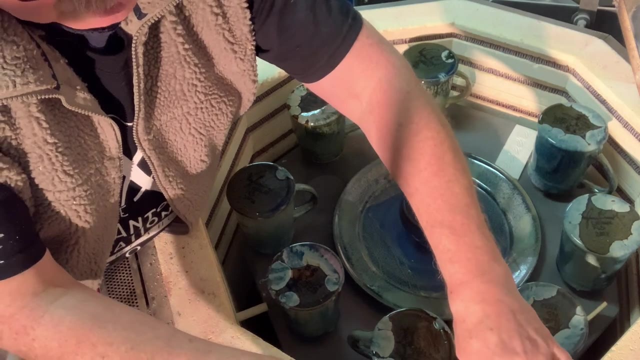 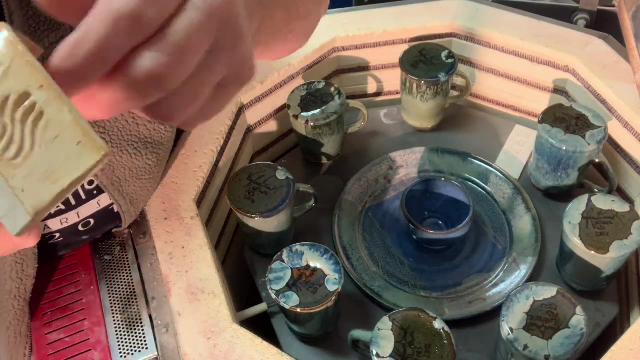 book, but that's great too. I should hold them up close so you can see better the light is not sure if you can get it just right, but it's satin matte. both of these are look. they look perfect. that's why I was saying with my oatmeal glaze it may not be the best one. oh my god, look at that. can you see this in the? 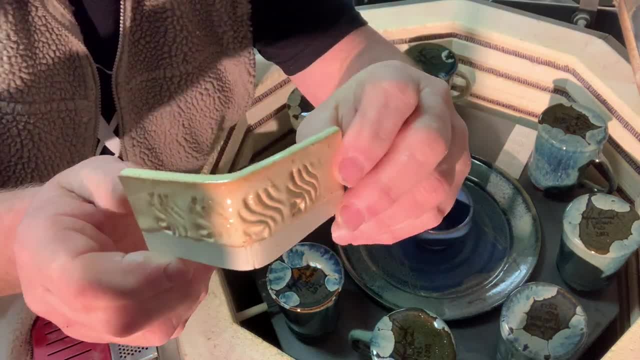 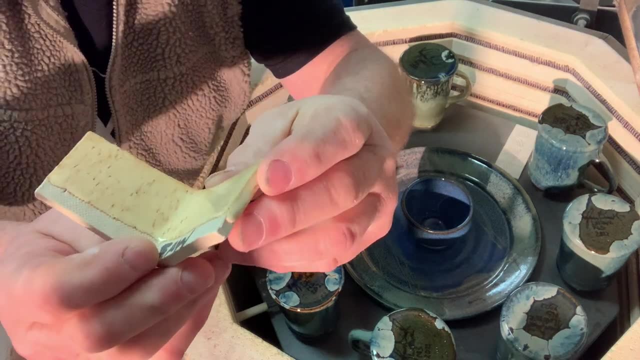 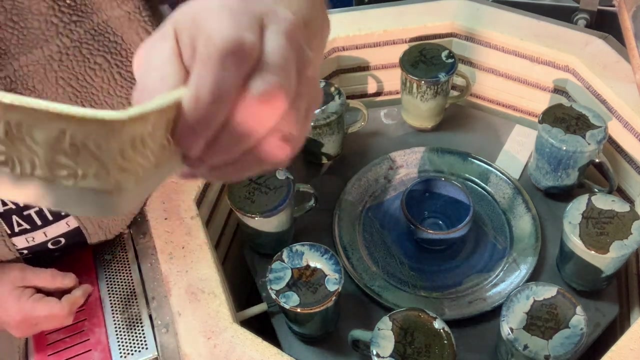 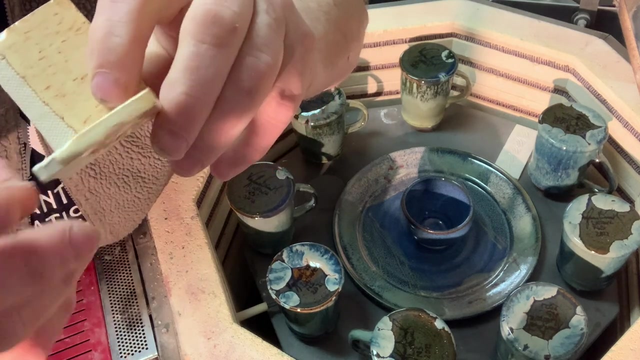 light. oh wow, I now have eight oatmeals. oh, look at this. this is beautiful. what one was this? this is the folk art white. I got this one. where did I find this one folk art white? I'll have to look in my recipe book. um, but that's intense. that is a keeper, for sure. 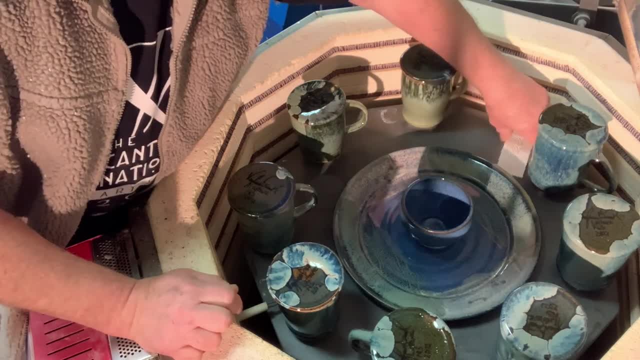 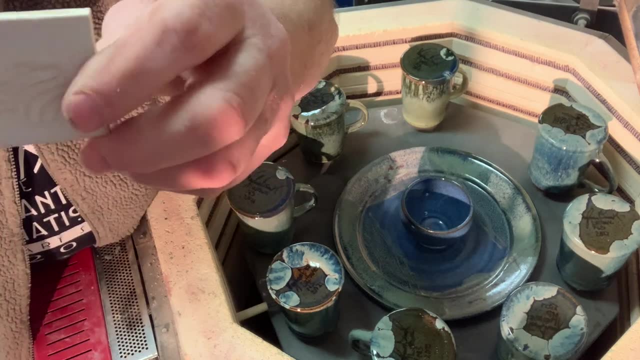 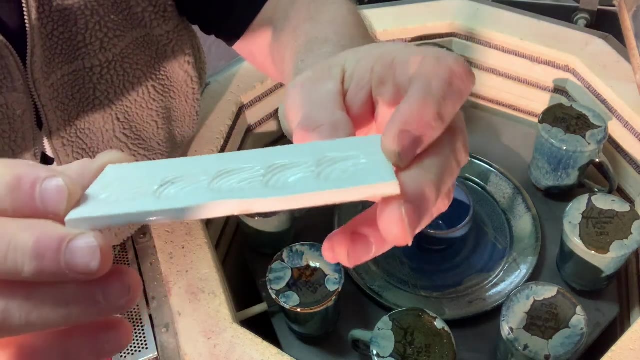 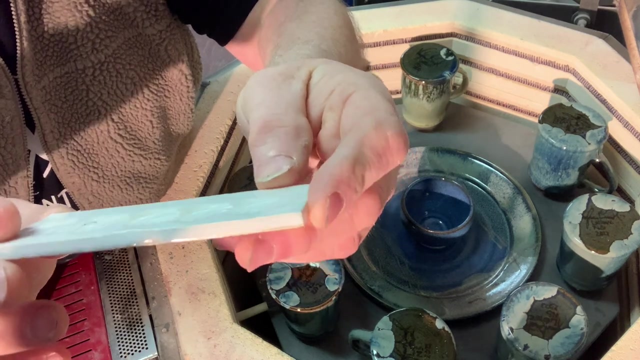 so three out of three wonderful. look at that. this one is a great white glaze, valcushing white. look at that, it's a. this one is beautiful too. I could make this into oatmeal by adding my iron ochre, which is what I did to this one. 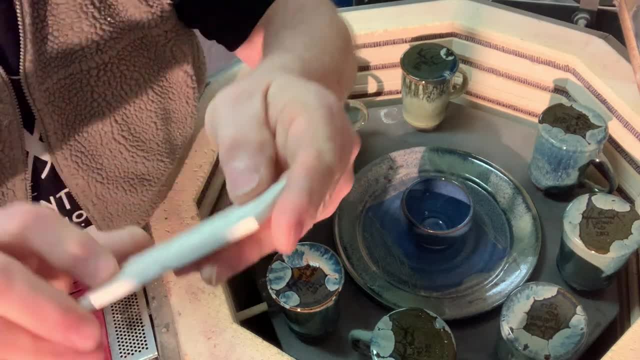 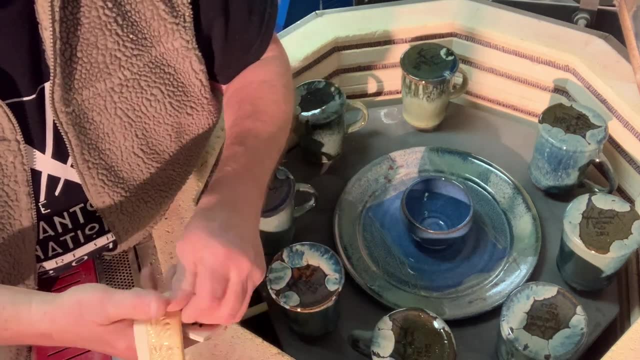 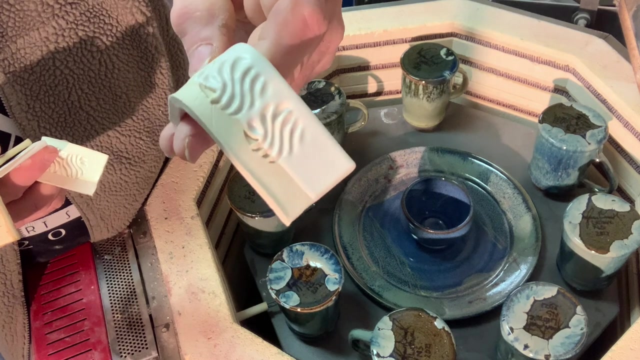 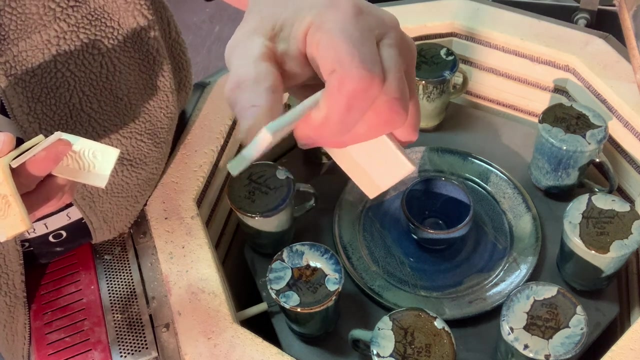 okay, so we're going to flip this over. this onebb got four new and look that none of them ran. i mean these are perfect straight off. but the david leach white satin is great because it's got the semi-matte quality without any titanium. this is just a glaze and it also has a shine to it. feels very smooth, so my 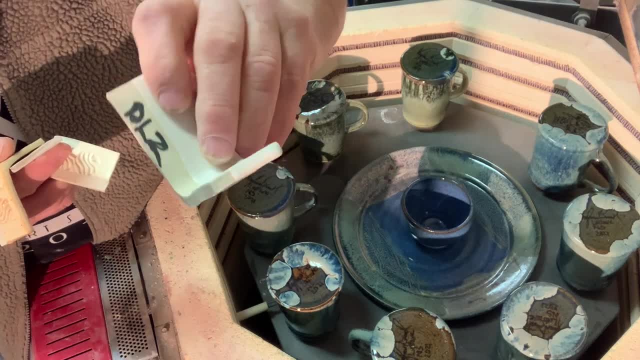 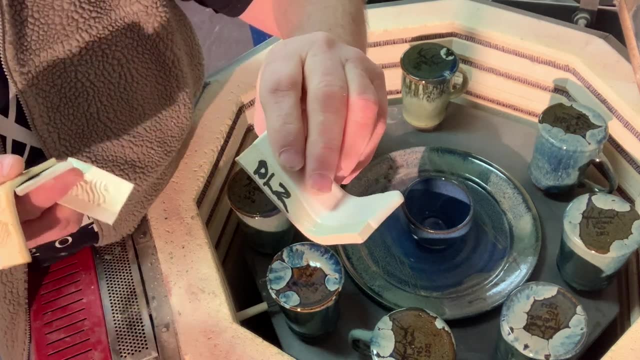 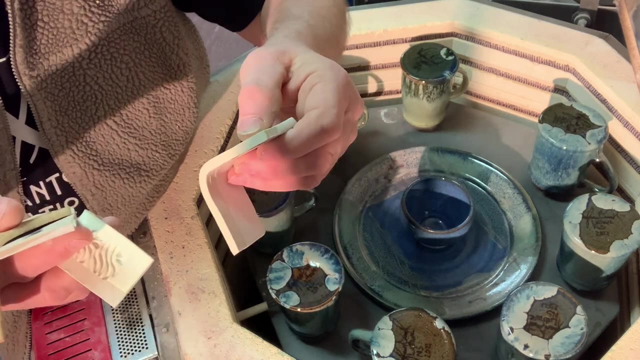 guess is, this one will be fine the way it is. i don't need to add any tin to it at all. and over the top of gloss glazes. i'm hoping that's my next series of tests, so i'm going to put it over my ten miku gold and over my bright blue and over my turquoise to see how each of these works. 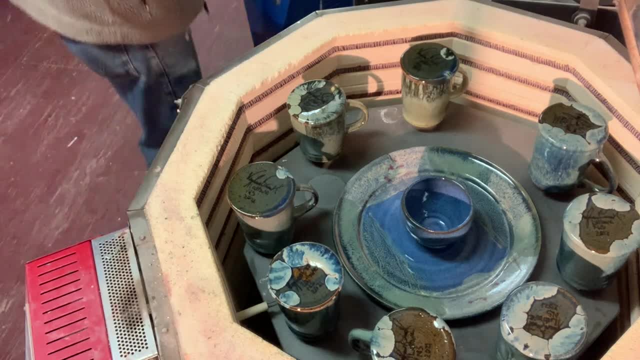 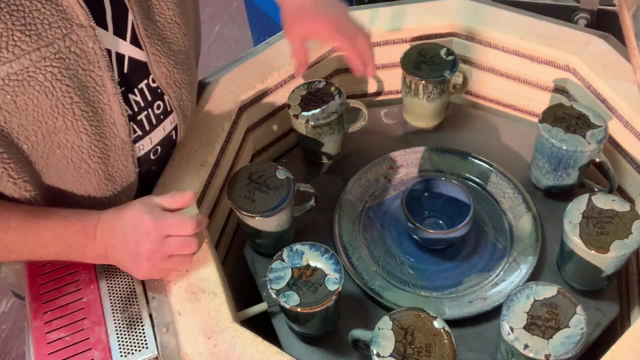 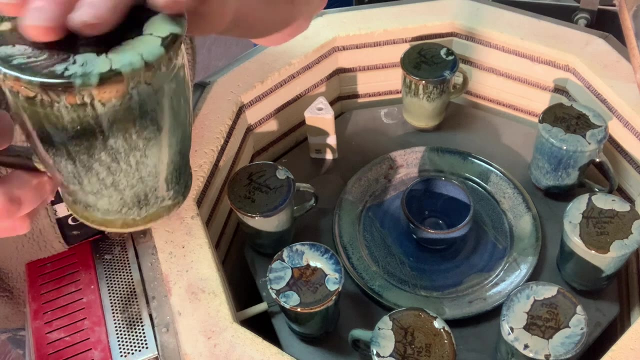 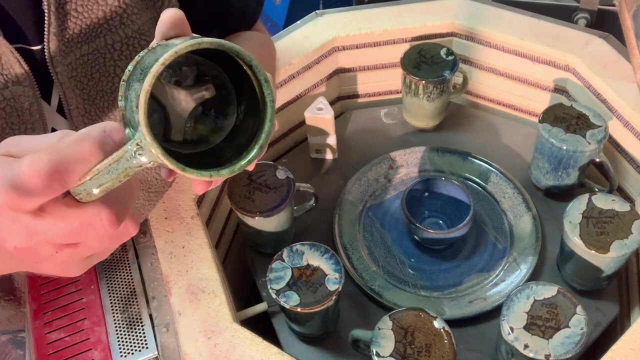 so i'm going to make some test pieces today. that in itself makes this a successful firing, but look what we did here. okay, these are all the ones where the bottom was bubbly and it's flat. so that's firing. there's the still inside, if you can see it. so fire with. 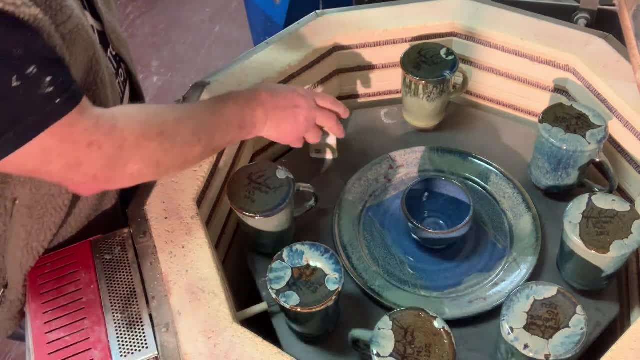 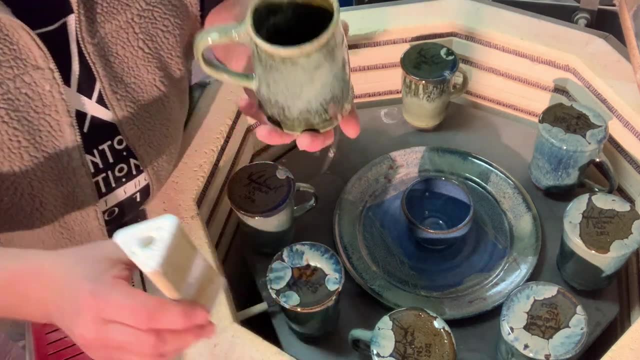 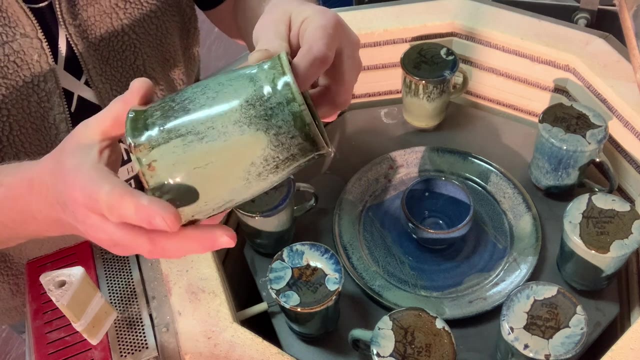 the stilt inside and basically sit it on some props so your rim doesn't touch the actual kiln shelf, and that's how you get them to from what was a, you know, a big grinding job with these, if i had to do it, um, but re-firing them on stilts works better, because the bottom, no doubt, is going to be. 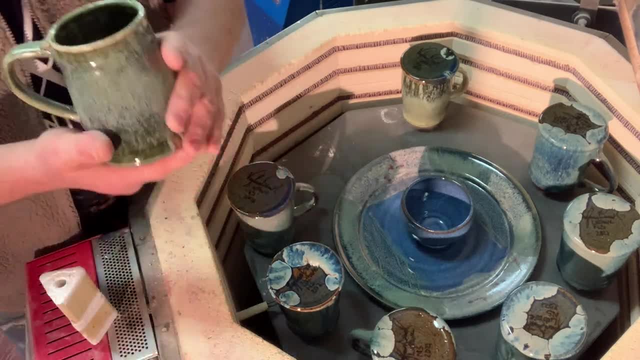 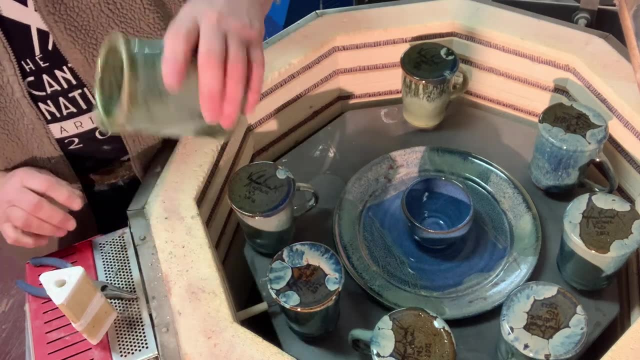 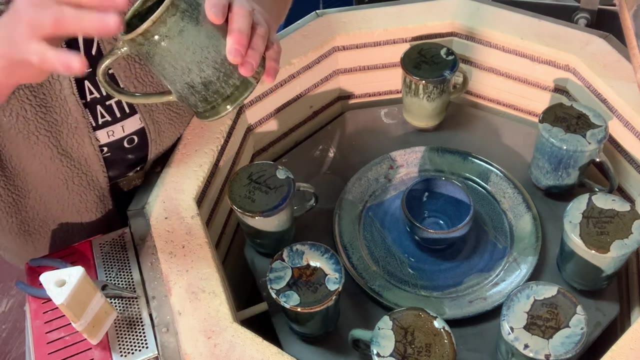 grinding marks at all and all that. so, and let's see if i can get the stilt out, because that's usually you just have to tap it and it falls right out. there. you go no stilt inside and then basically, if you can find a drill grinding thing, just kind of touch each one of those. 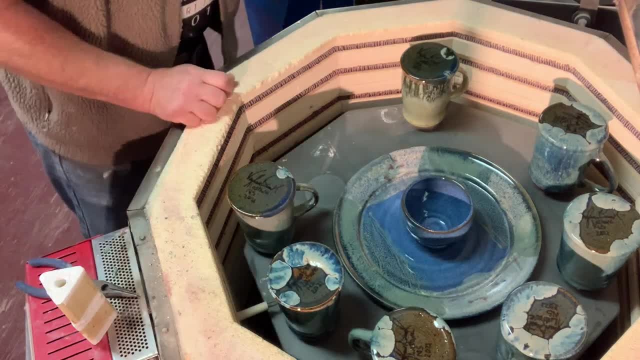 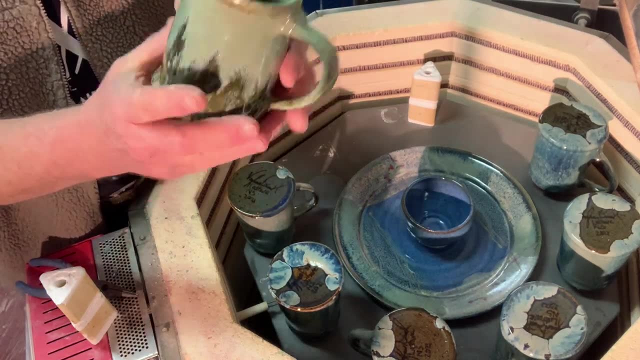 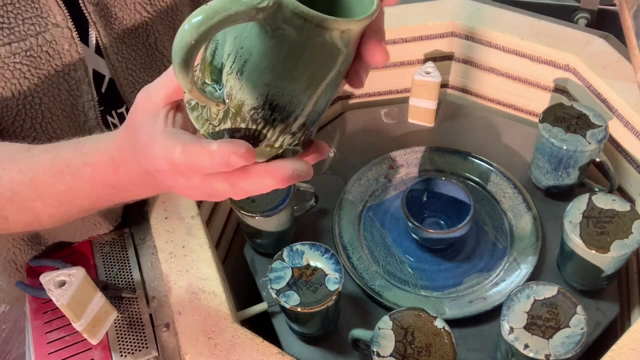 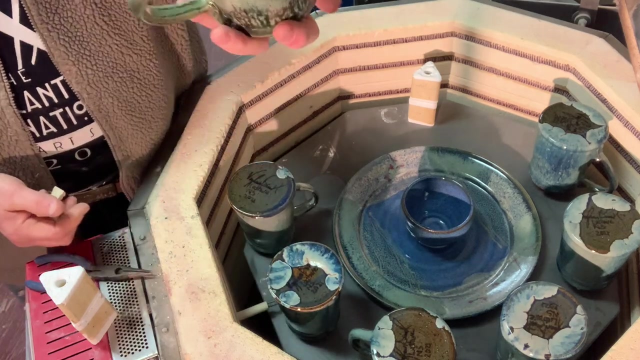 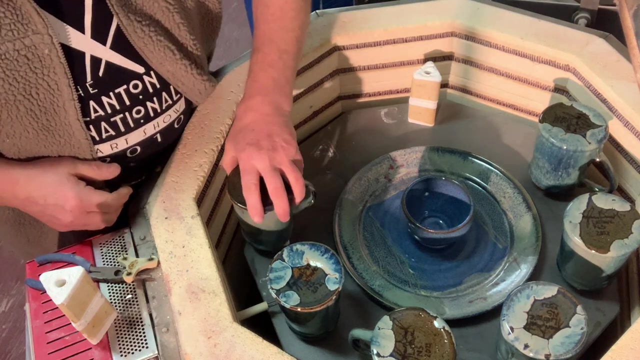 three sharp points and that'll blunt them. same again, and even the writing's showing up. this had run right into the writing before and you can now read the writing perfect, so let's see if i get that stilt out. yep, so another success. and all of these basically had run and made the bottom bubbly. not bubbly, but you know what i mean. 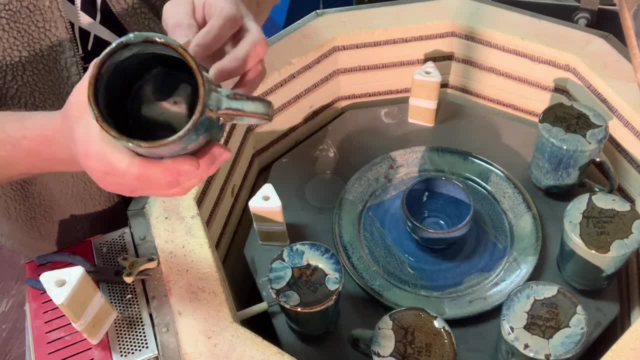 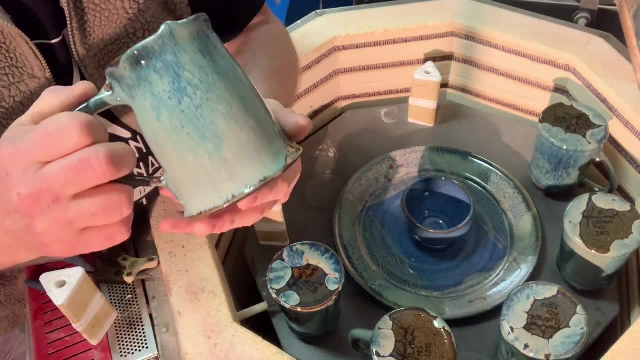 is like lumpy and all that, and now they're all perfect. this one, you can see, ran to the rim and gave me a little bump right on the rim, but it's on the opposite side of where people will drink out of it, unless they're left-handed. 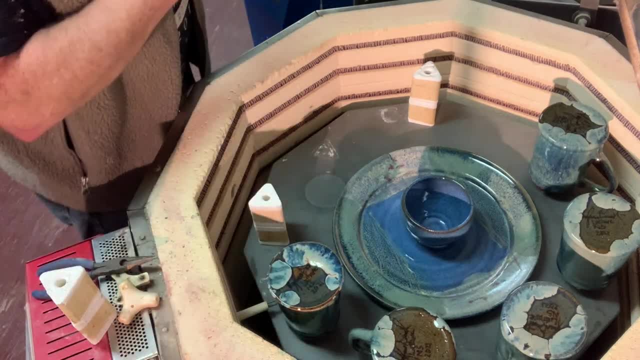 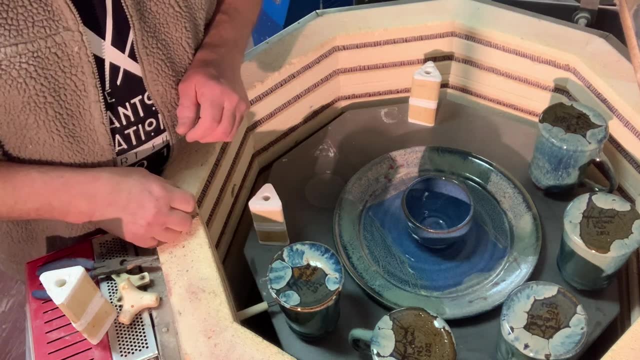 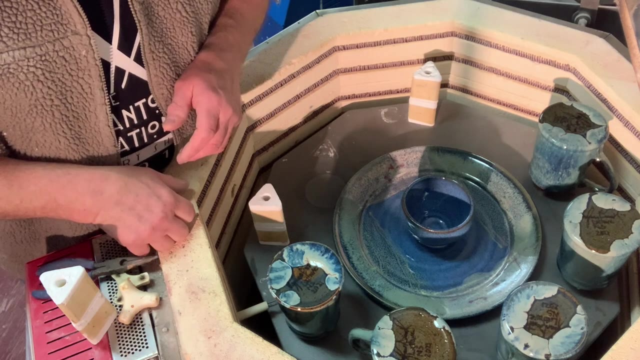 but that's the variegated blue which is really bad for running. now the profile on this is: i fired it to 2205 with a 20 minute soak and then speed cooled it down to 1750, which means let it cool. naturally didn't slow the cool down at all and then soak for. 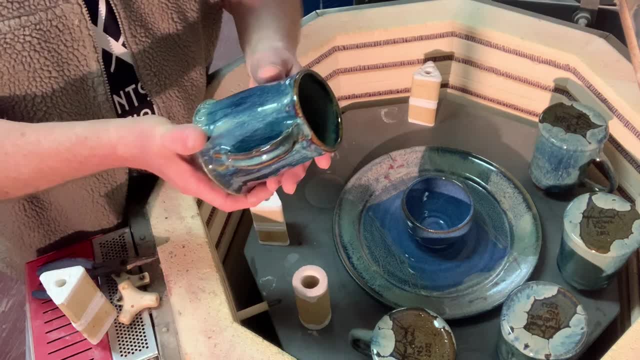 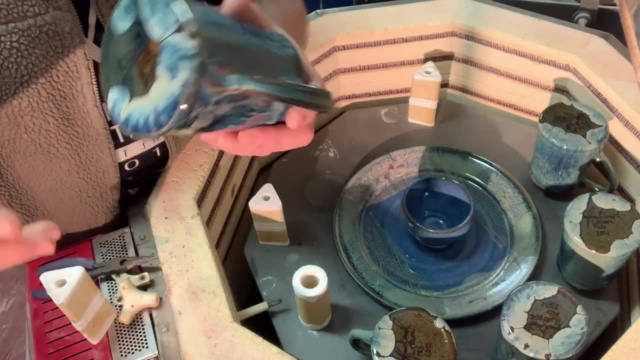 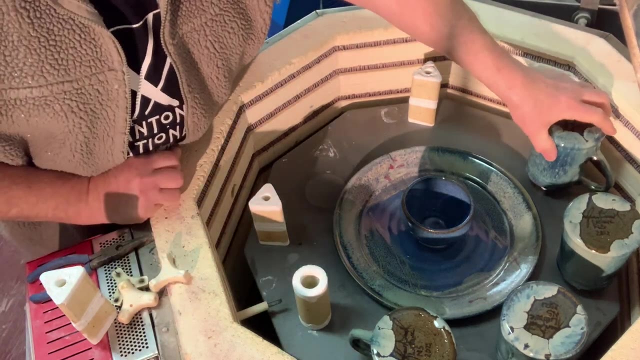 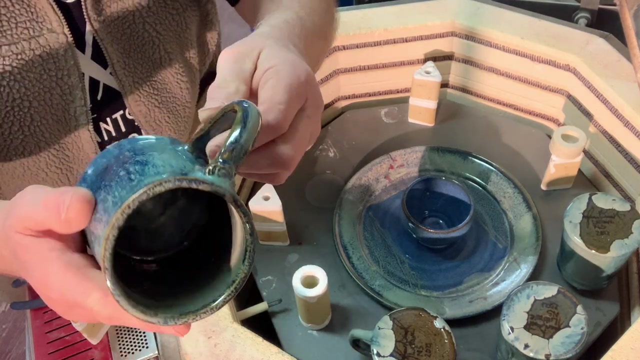 an hour at 1750.. and that one did good too, see, they didn't run to the rim except for that one, but they flattened out on the bottom. so this kiln is actually solving several problems. this firing, another flat one on the bottom stilts out. no running on the rim. 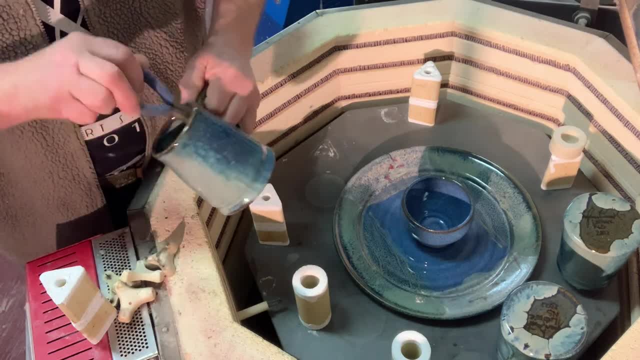 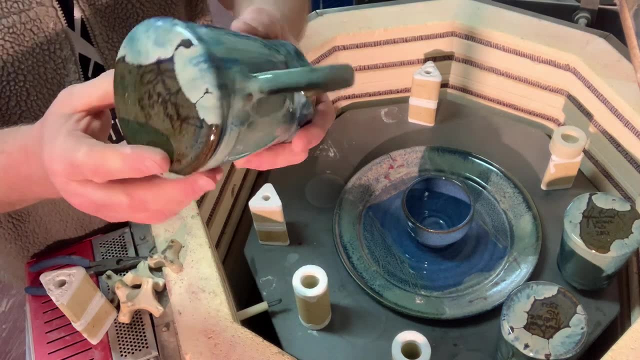 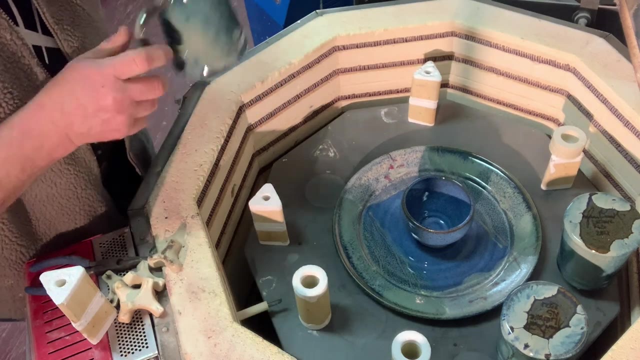 this is a major. i've been meaning to basically try and make these oatmeal's for a while, because people have been asking and i wanted to see, because i just had an oatmeal, i mean, who knows if it was a good one or not- but now i've got four that look like they're as good or better than my oatmeal. 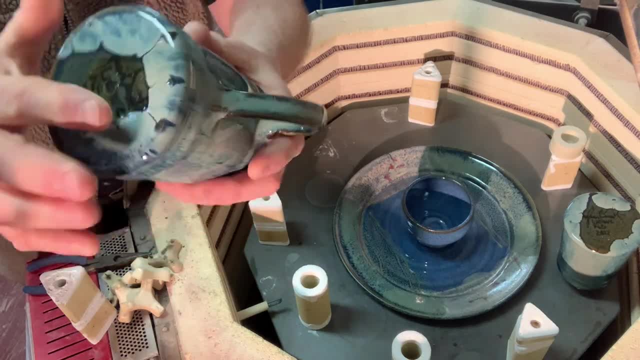 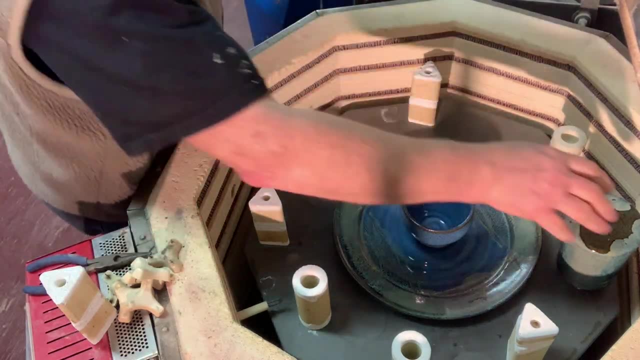 so no running on the rims, so it was time to just write. so i'm gonna try and make some more of this and see if i can do it. so i'm just gonna try to make this completely flat on the bottom without any grinding. perfect, the nicest word in the english language. 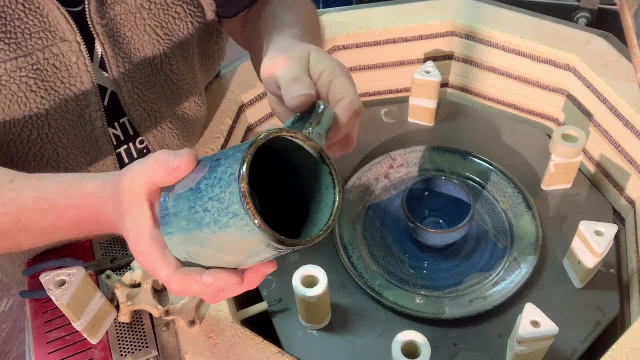 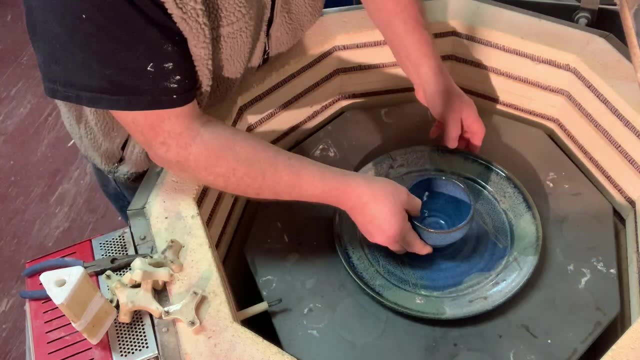 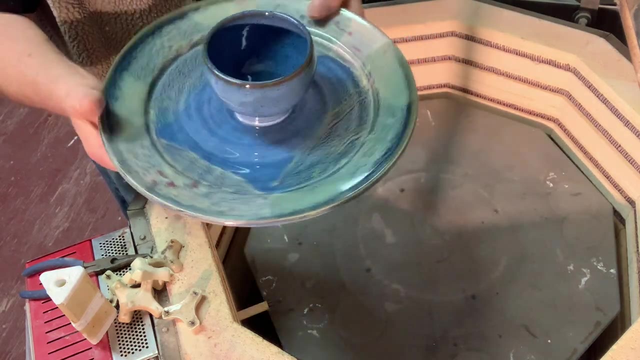 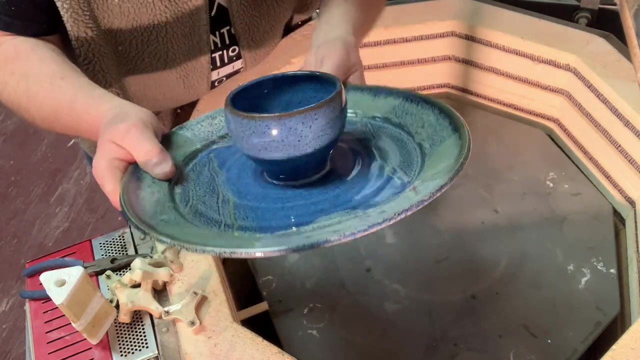 all right. look, the crystals are even more than the first firing, so i'm a little surprised that we don't have any glaze bubbles. but i lowered the temperature of full. I've done a lot of firings. I go through cycles a couple of weeks- I'm just starting- a couple of weeks of throwing building inventory and then basically, but also planting seeds. It's spring, It's a pretty oh, that's a nice, oh- chip and dips. That's why I have a lot of chip and dips in here. 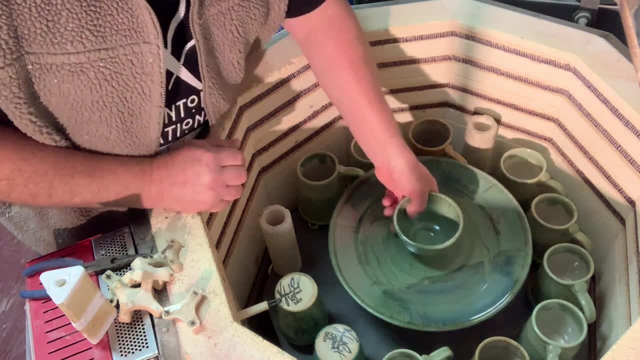 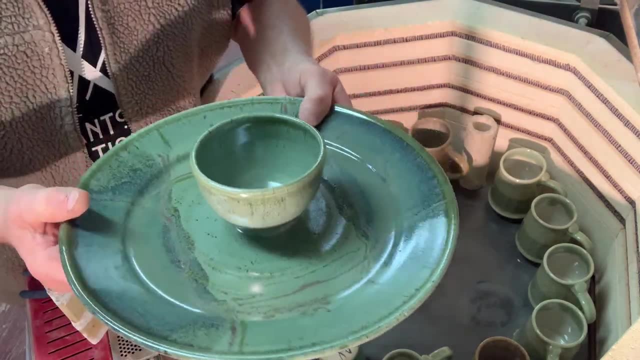 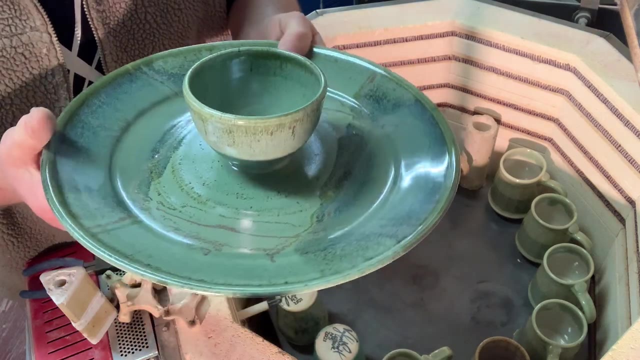 Oh, okay, I think we this is the nicest of all these kale loaves. Okay, There's a really nice chip and dip with my green glaze. I keep in. I'll take a picture of my recipe. It's called Maggie Jerk Green because I got it from a lady called Maggie Jerk who lived in Nova Scotia here. 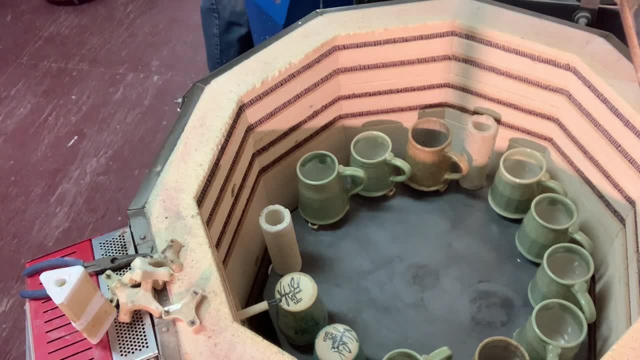 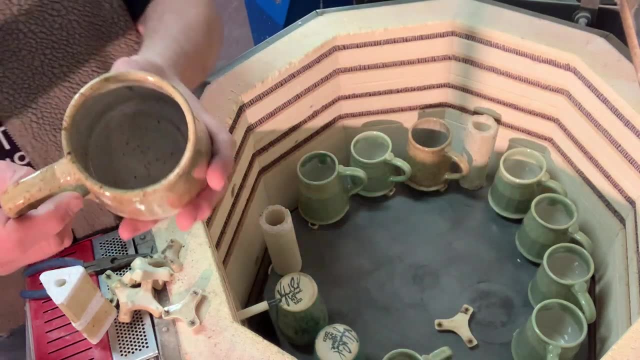 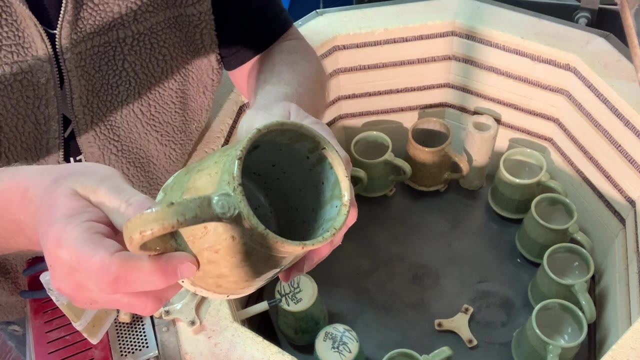 Very pretty. And now what? What did we do with these? These are the refires of the fake ash, And this worked perfectly too. I dipped my oatmeal like this in my oatmeal, over the top of the fake ash, which wasn't doing too good. It had blistered a bit And this now looks better. Really nice. 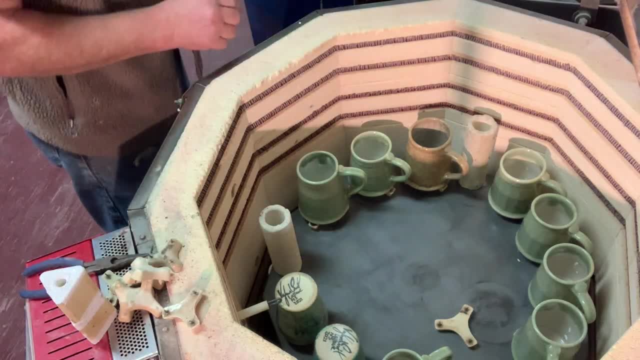 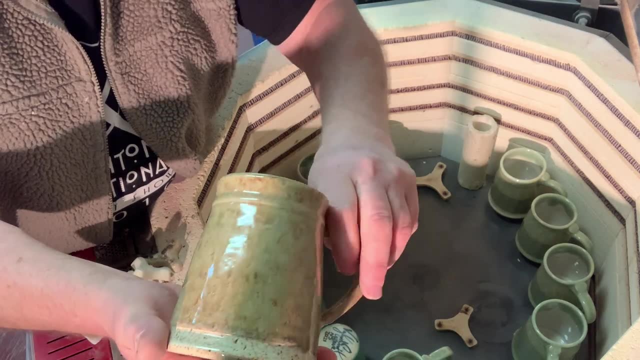 So that worked too. So we sold the fake ash. So when I do the fake ash it looks like I have to double dip with your green glaze. I don't want the oatmeal over the top if I want it to work the way it is, But I am going to try raising its temperature by putting some more silica in it. 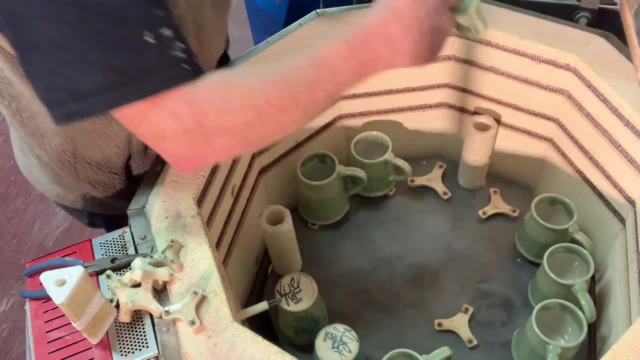 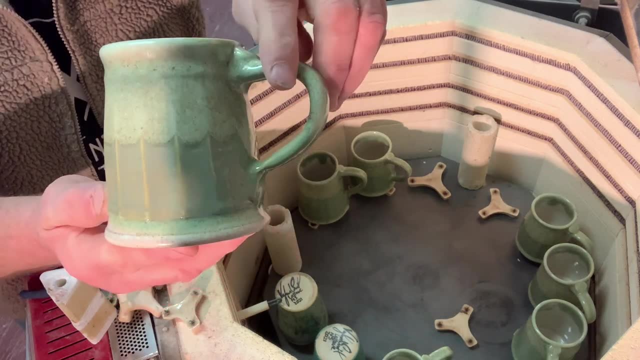 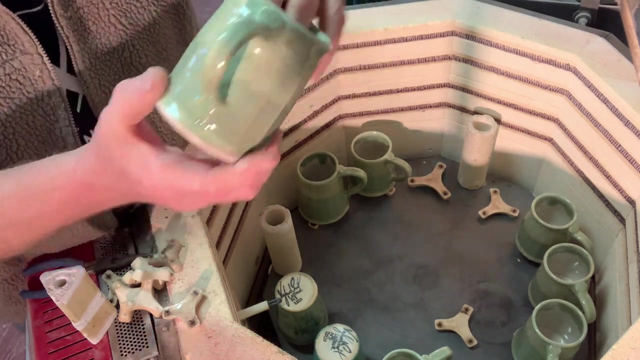 Any more fake ash? Nope. Then we have a glaze I don't use very often. I call it rutile green Copper carbonate with some rutile in it. I'll have to look what else is in the recipe. It's very pretty though. 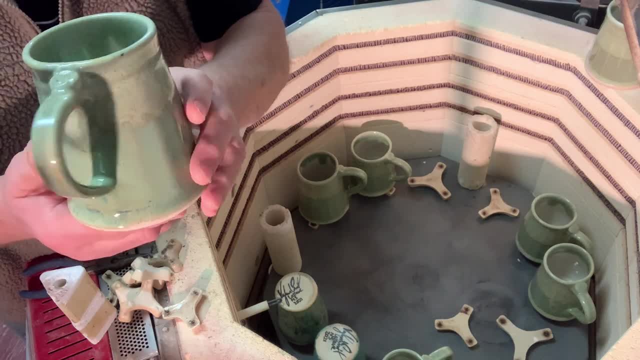 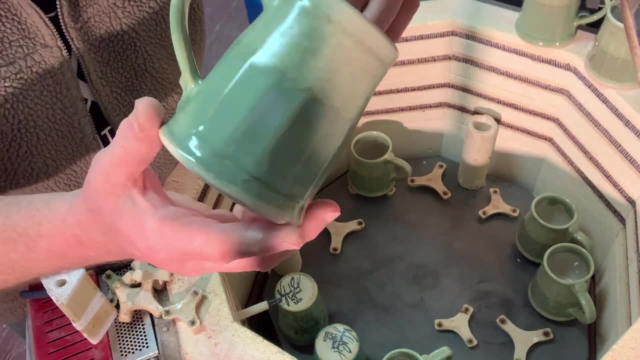 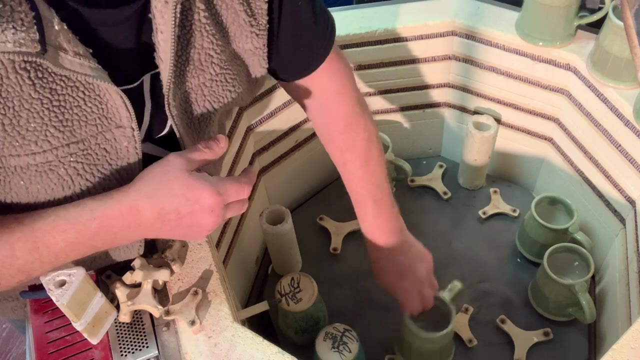 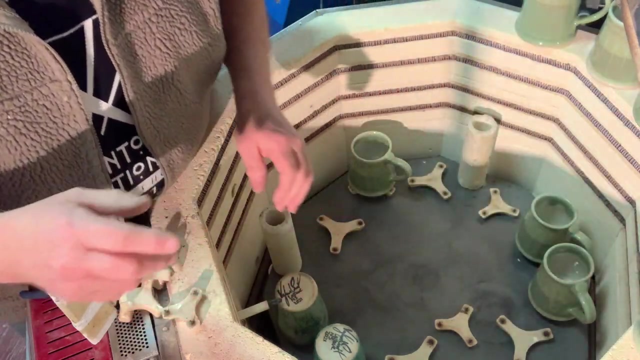 I'll try and hold them in the light. Very pretty, I remember doing these all the same: glazes on each piece, on each level. And there's another interesting test here Coming up. Let's see if I can hold you over there. 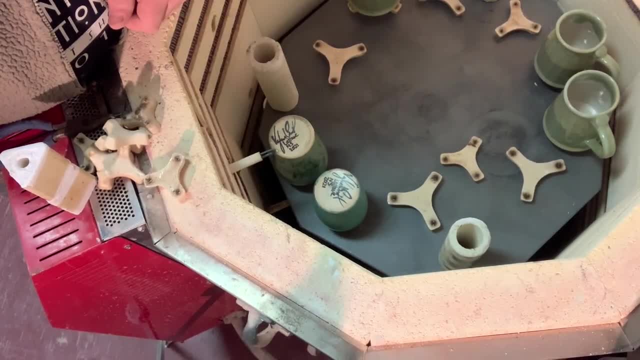 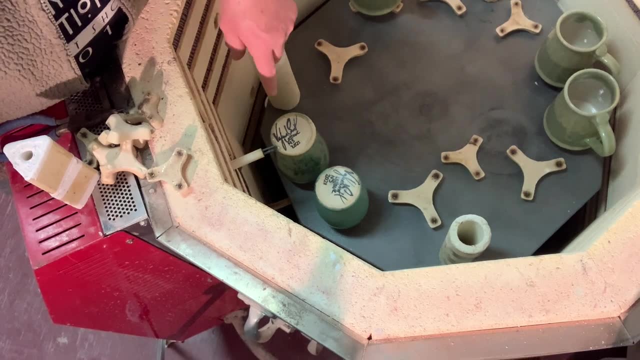 I fired these two pieces upside down on their rims, their lotion dispensers. I said this earlier in the video Because they had run over the bottom And I wanted to see whether I could get that run to go. You saw it earlier in the video. 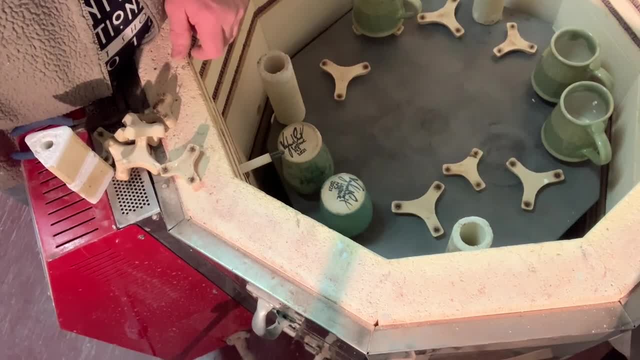 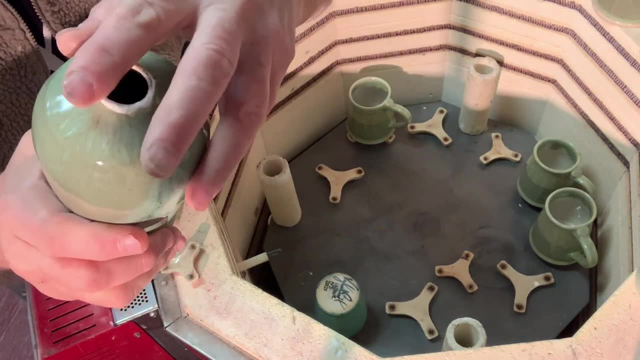 Without sticking to the kiln shelf. But we'll see what it is. Let's lift that up again. Yep, it didn't stick to the kiln shelf And these are lotion pumps, So they're going to have a plastic cap over this area here. 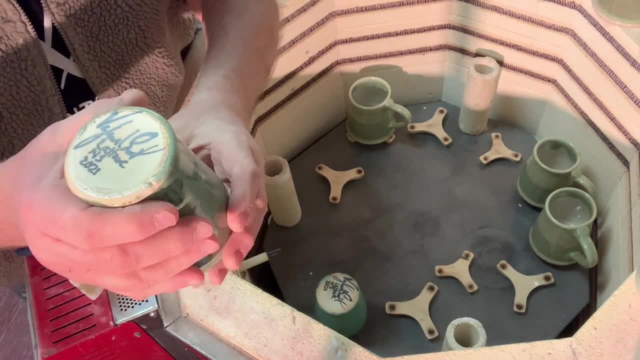 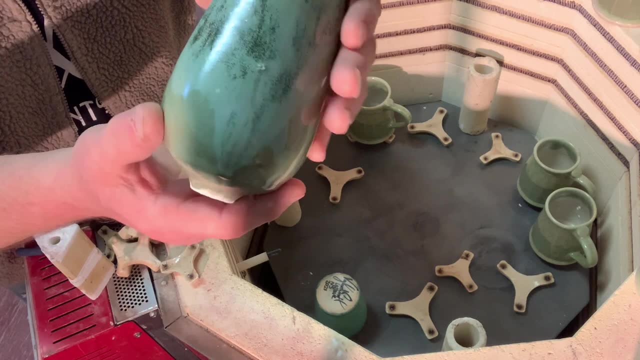 So what I did? because they had run all the way big kind of over the bottom here, I fired it upside down to get that run to melt in And you can see from the melt it's gone all the way back in without going down to the kiln shelf. 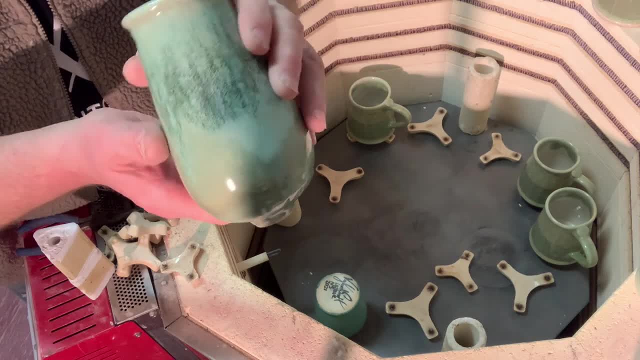 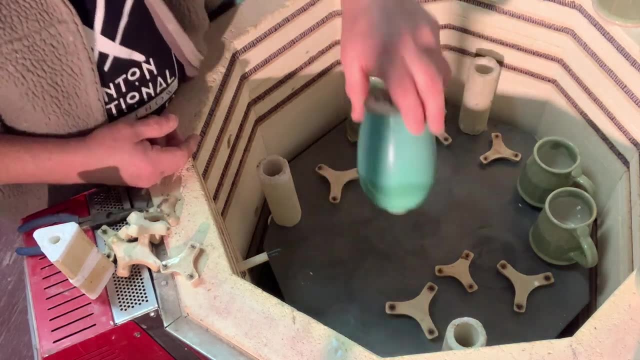 But now I can stick the plastic stopper over there to actually save these pieces too. And the same with this one. Yep, worked again. This is the one that had. this one did. these shells are great because they don't let anything stick to them. 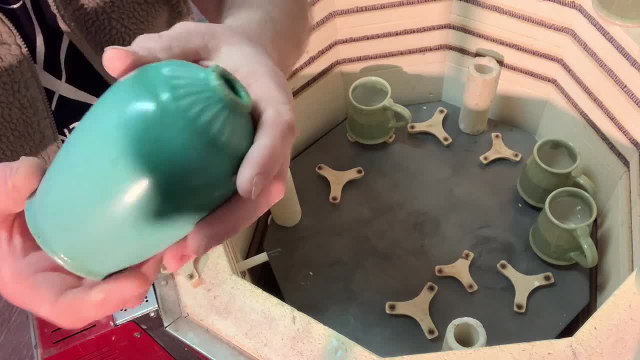 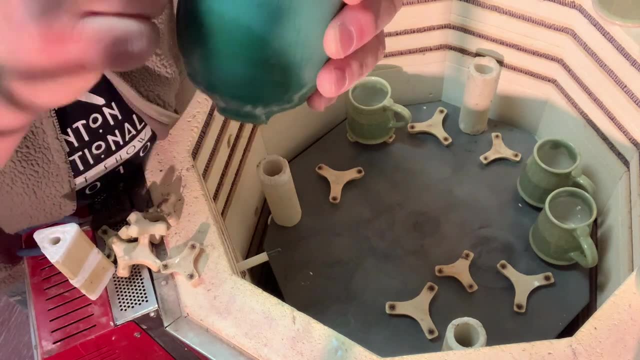 And I can just light sandpaper that and stick the plastic cap off. And this is the one that had the glaze spread out all over. It was really white And it melted. You can see how it melts down that way. So you've got that line. 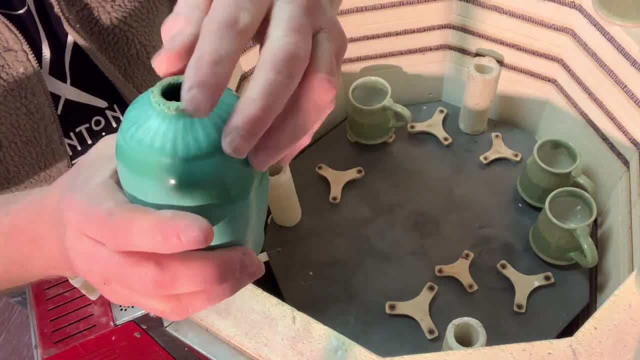 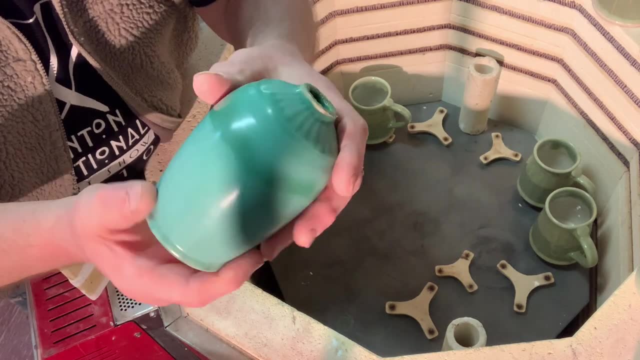 But basically bottom is now perfect. The top is a little rough And I'm going to stick my little plastic lotion cap over that and that'll be gone. So that was a complete save as well. So then we've got some more of these rutile green. 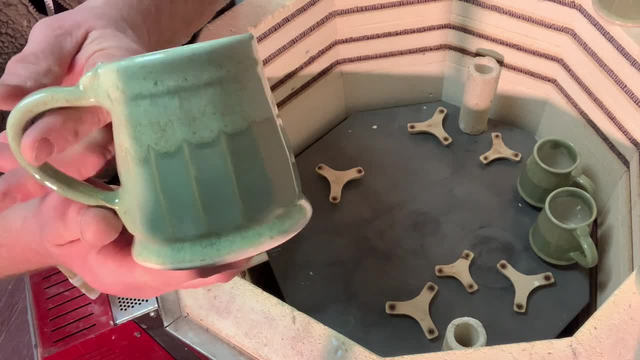 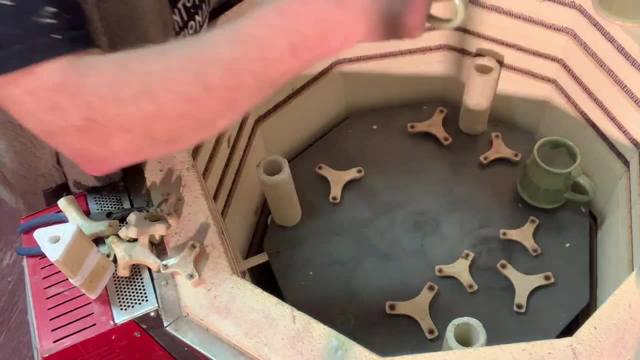 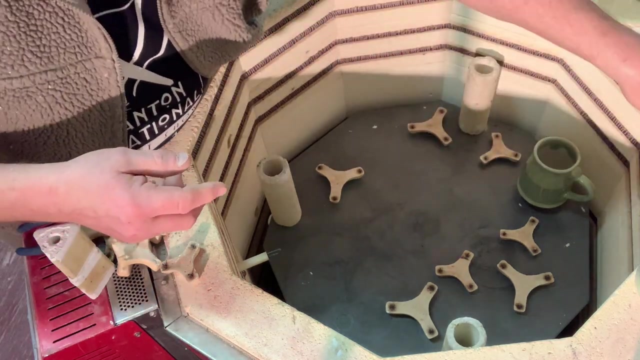 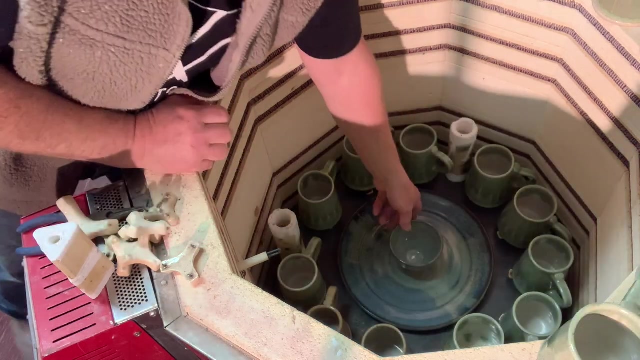 These are actually really pretty. I don't use this glaze very often. There you go, Of course, with the fluting, it always makes glaze look really pretty. So we have a set of these. Okay, another chip and dip. That's how I did this, all the way down. 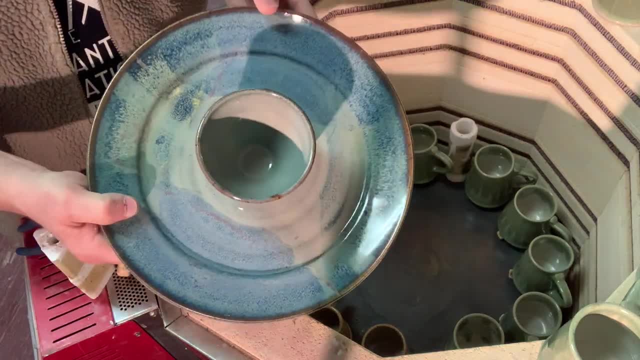 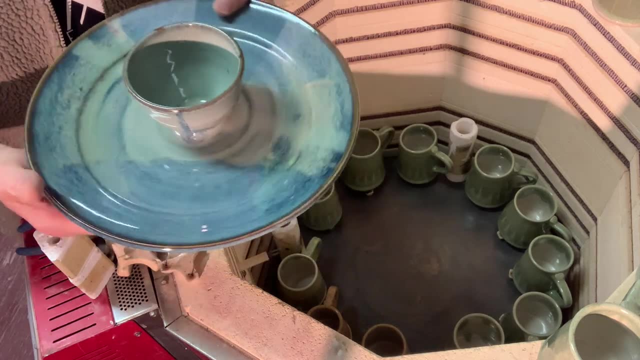 With variegated blue. I'm not sure if you just heard that, but my cat is scampering around all over the place. He's an old man, He's 14 years old And he's a kitten right here in the studio. 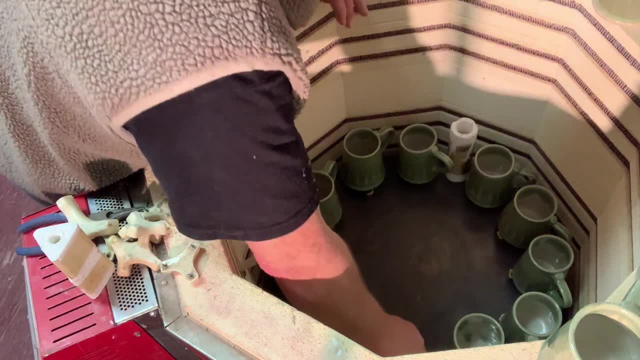 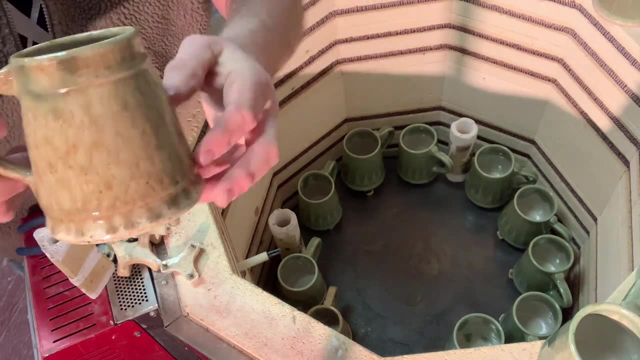 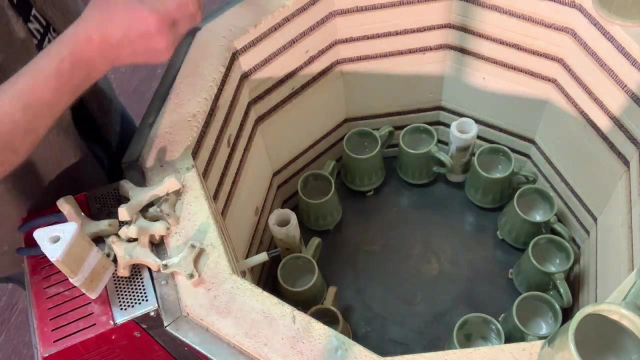 He's like thunder feet all the way across the upper floor here. This fake ash really does look nice with the oatmeal over it. You can see how it runs down. But these were terrible after the last firing. Now they're good. That's another fake ash. 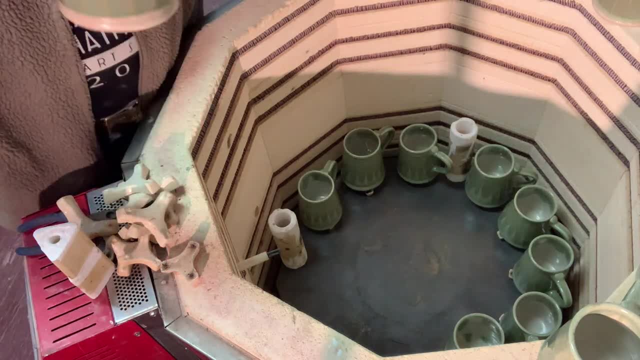 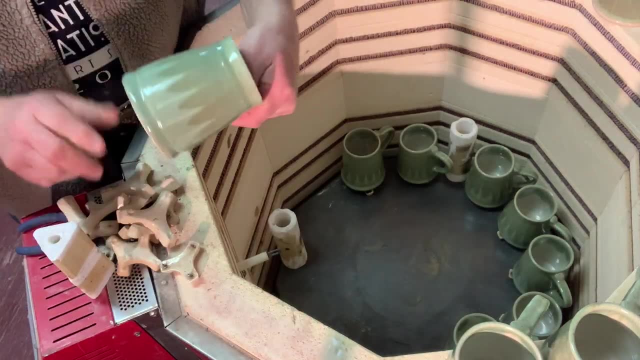 And then we have a whole bunch of the. What did I do to the? That's another one of the rutile green with the oatmeal over it. This one is my- Oh look, there's one that ran. This is the apple green again. 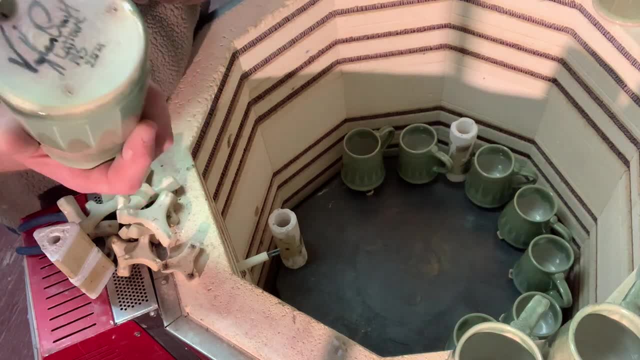 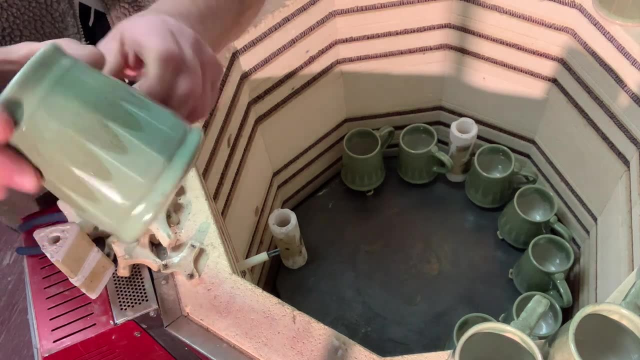 So even at a lower cone, where the handle is, it ran all the way down And then I'll grind that a little bit. That won't be bad at all. But there's some nice run marks on that. So I had apple green here with something dipped over the top. 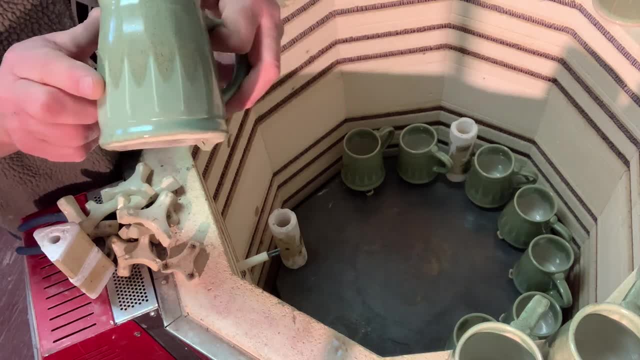 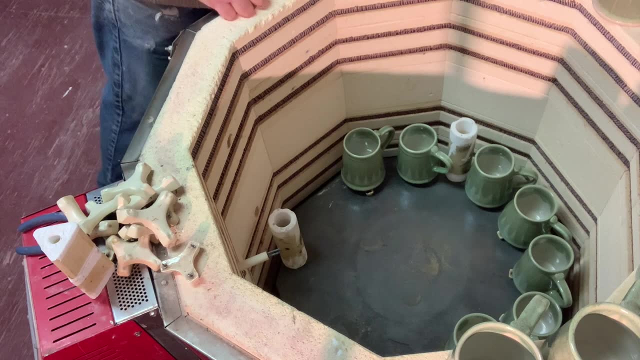 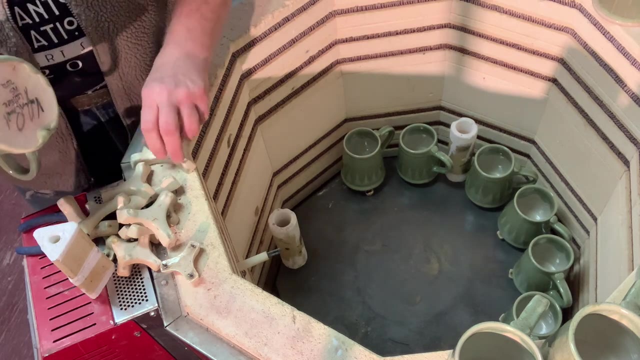 And the way it did that pattern like a crown all the way down, But the apple green definitely runs. I'm going to try that and see what that apple green And it's the same again on this one- Just a little bit right at the handle where it runs a little bit more. 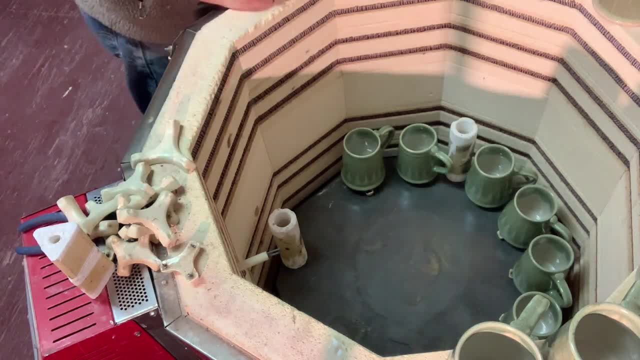 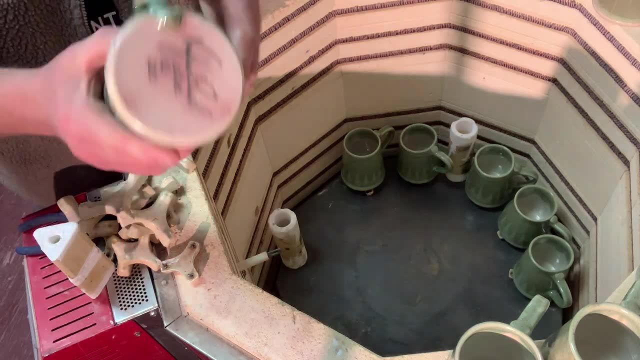 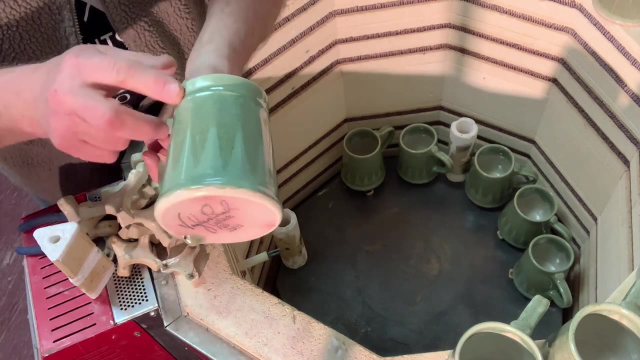 But the rest is fine. So these are saveable just by grinding. The only way around that is for me to dip less time in the bucket. But it's a very pretty apple green And then I think I just do my oatmeal over the top. 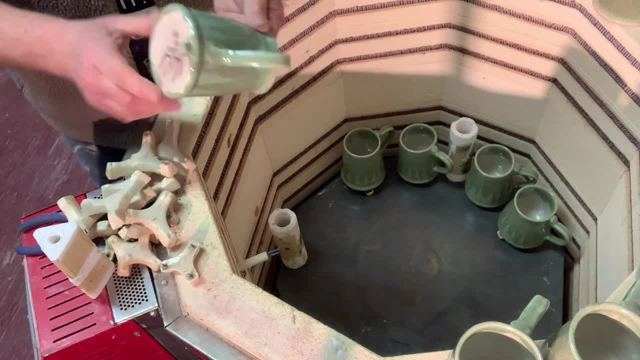 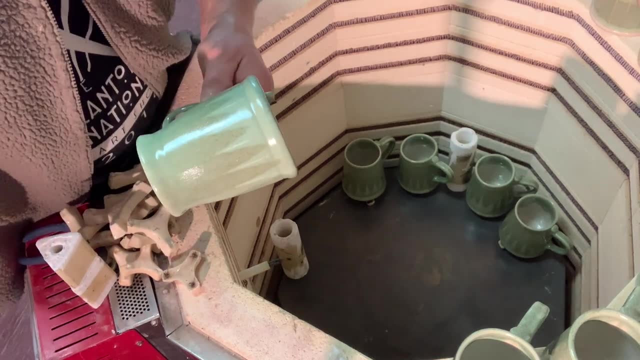 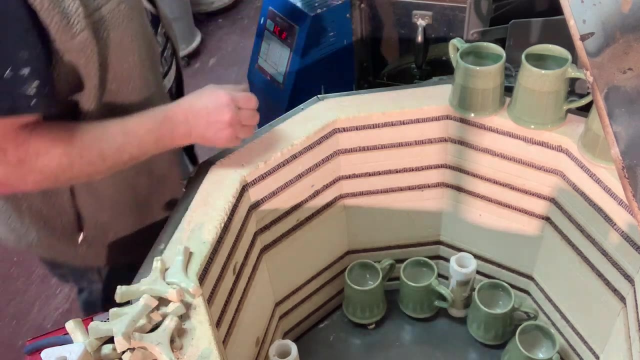 Yep, that one did it too. So all of these need- I'm not going to refire these because I can grind off that one little thing- Let me switch you up a bit because I'm missing you. sometimes I remember what I did. 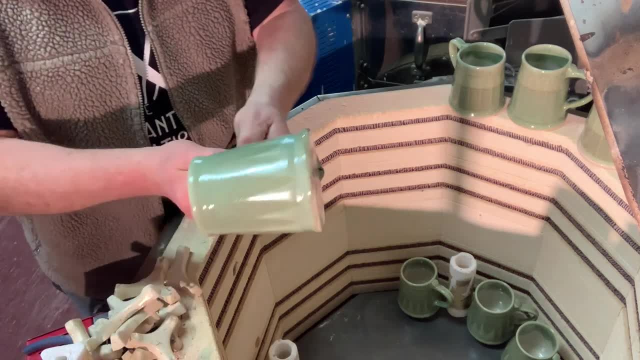 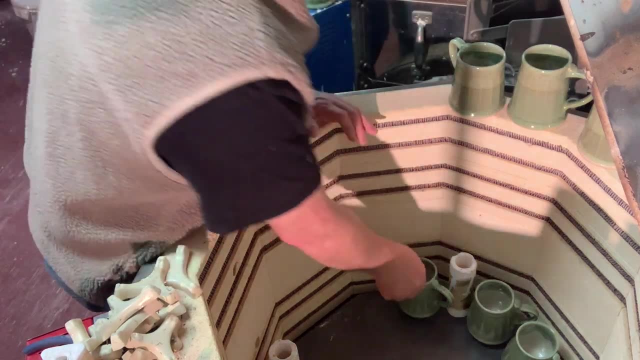 I did 10 Miku Gold on the one underneath here, So another one of those, That's the apple green with the oatmeal. So we've resolved it by refiring upside down, But if it's just one, drip a cone 5.. 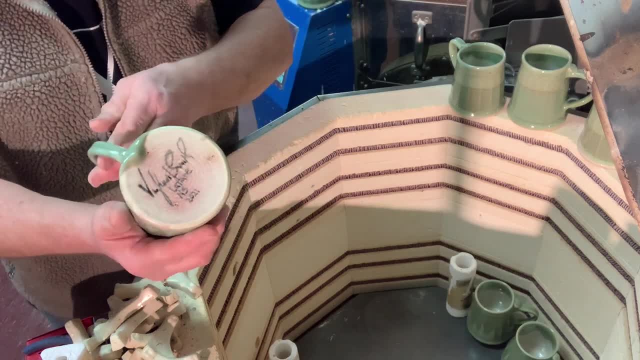 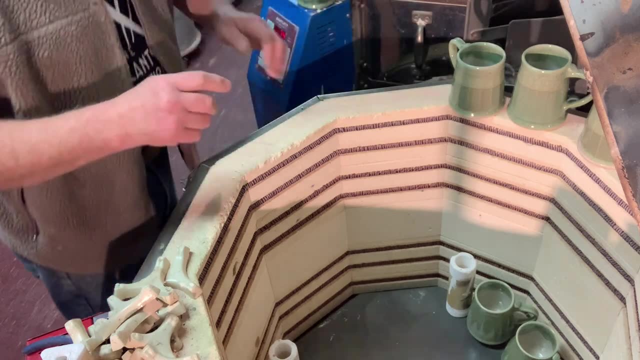 2205 is literally about cone 5.. So basically the apple green still runs a little bit of cone 5. And it is supposed to be a cone 6 glaze. So I'm wondering what happened there. Or that one. 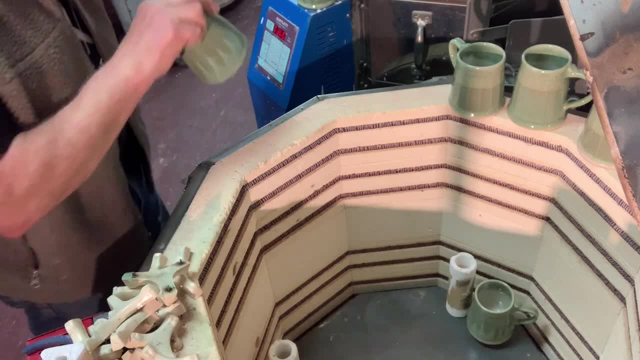 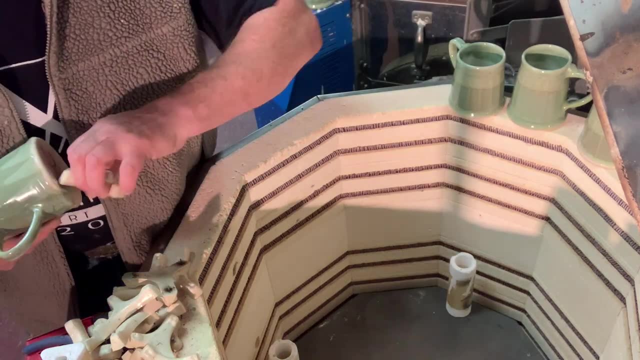 Same again: Always right where the handle is. Get that little run, Grind it off, But you should be able to get this glaze without that. I could add a little silica to this glaze And that will probably get rid of the run. 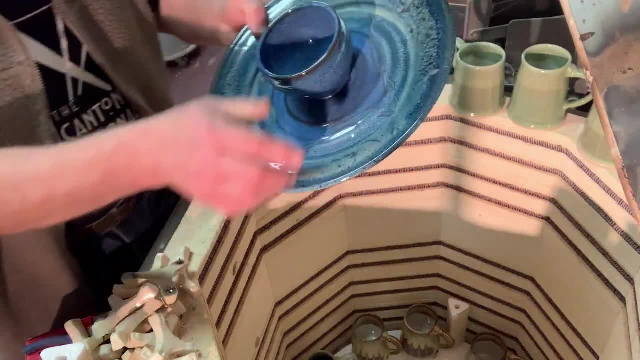 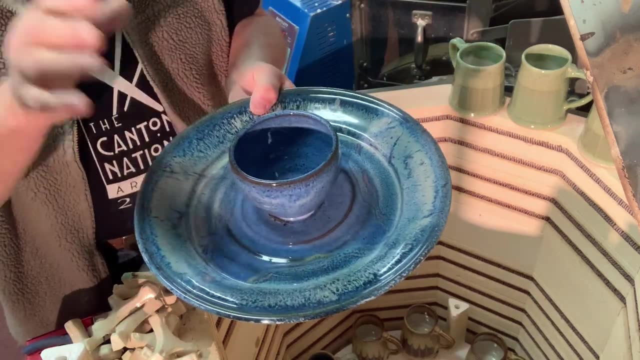 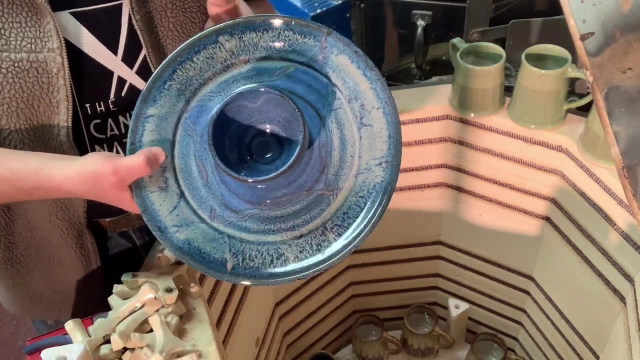 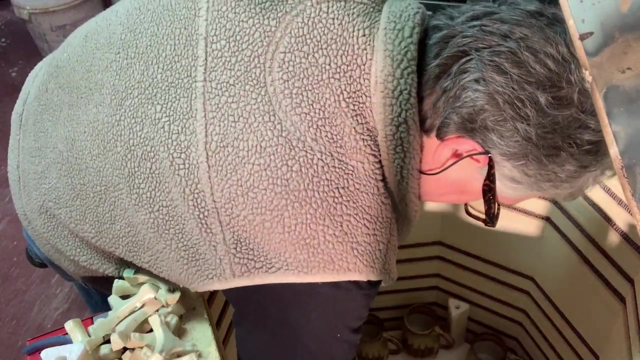 Pretty, My bright blue, Dark blue, No, Very giddy blue. So bright blue first, Then very giddy blue And oatmeal swipes Blue is very popular around here because we're on the ocean. And another fake ash. 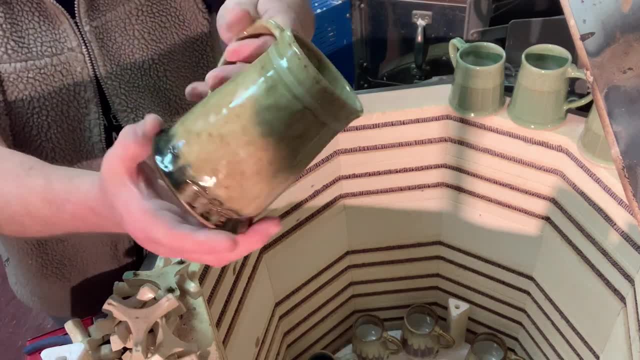 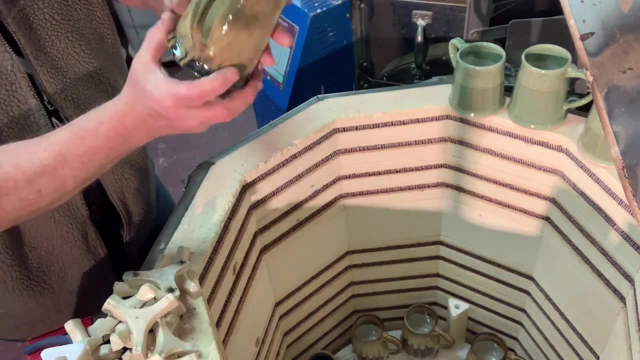 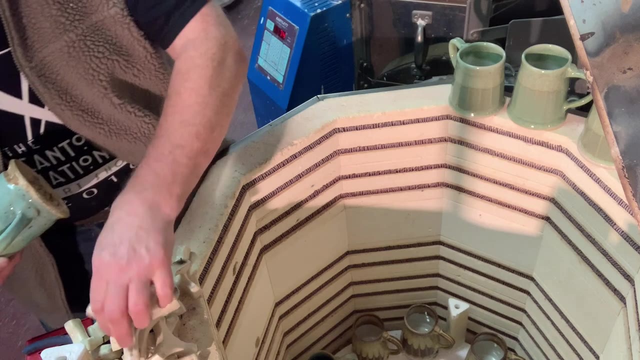 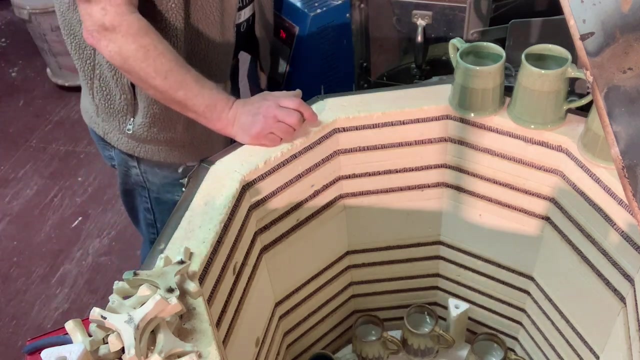 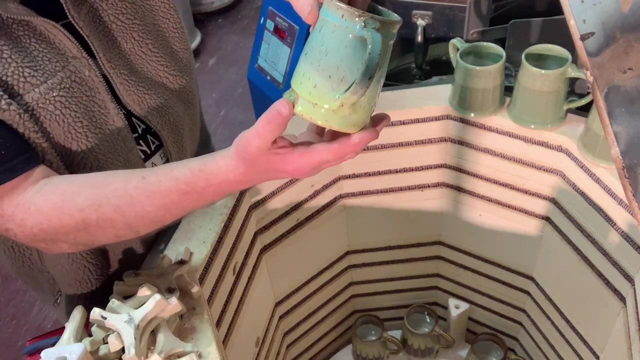 Which is really pretty with the blue on the bottom. So this oatmeal over fake ash works great. I should write that one down in my book. Got a few of the turquoise ones With the oatmeal on the top. Another oatmeal over the turquoise. 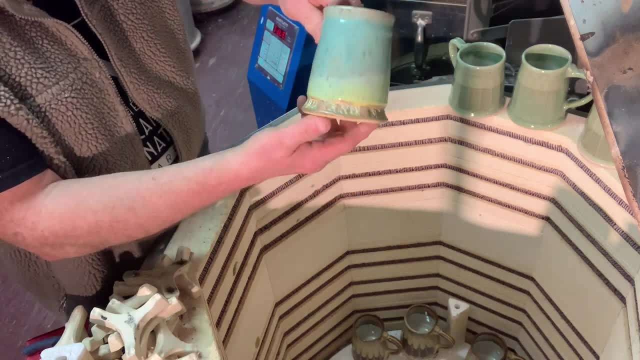 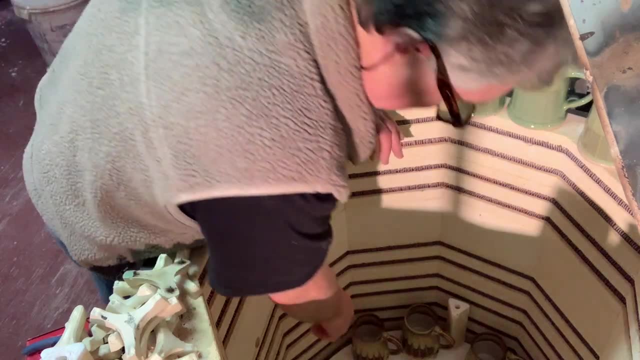 But done the other way around, Because this was an order for somebody who's got their names on it, So I had to dip top from one and bottom from the other for that couple. That way they can tell their mugs more, And this is the best I've seen. 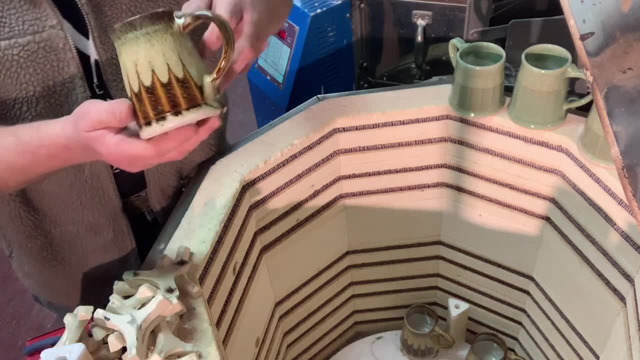 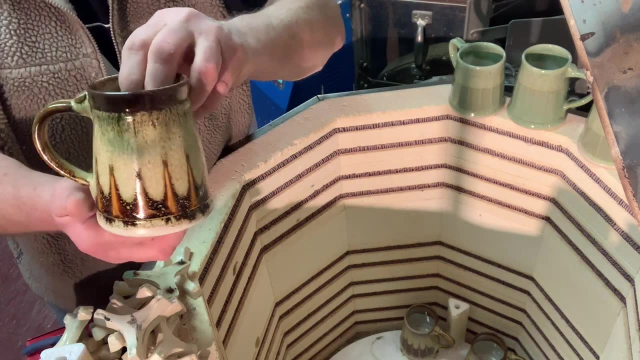 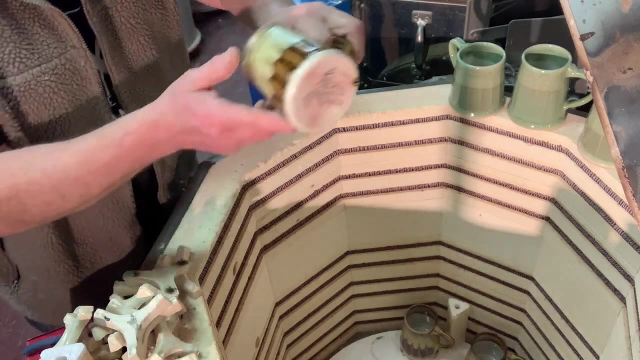 This. Look at that, Look at that. I have a series of these out. Somebody wanted a Tenriku gold mug, So if you see one of these, You should just email me again, because I lost your email And they all did it. 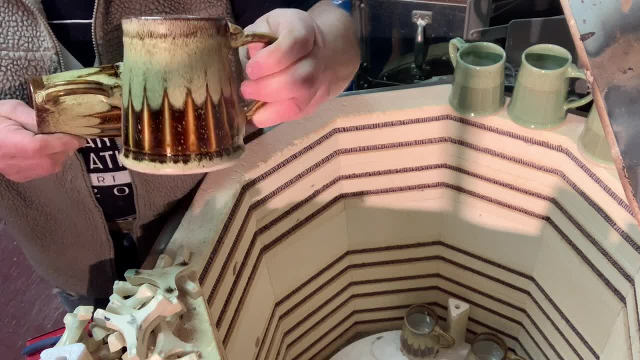 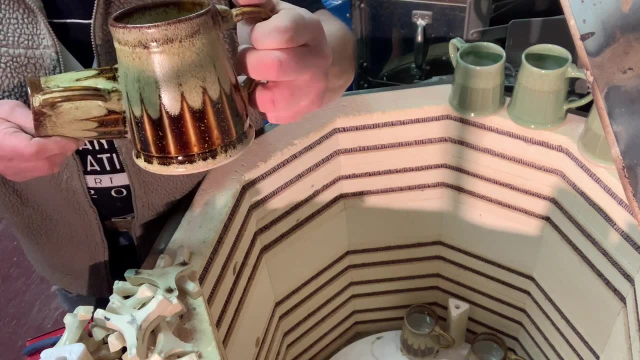 It's perfect. So when I do this, I'm going to write this down, This firing schedule for Tenriku gold here, Because that oatmeal is perfect. If I go to cone six, it melts right into the glaze And turns out: this is done. 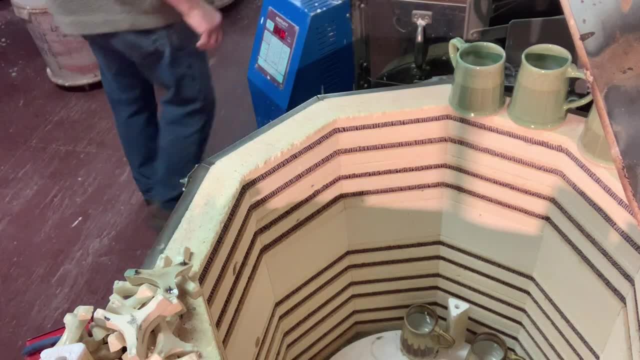 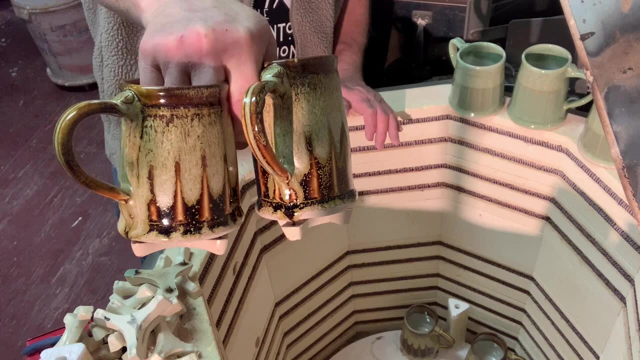 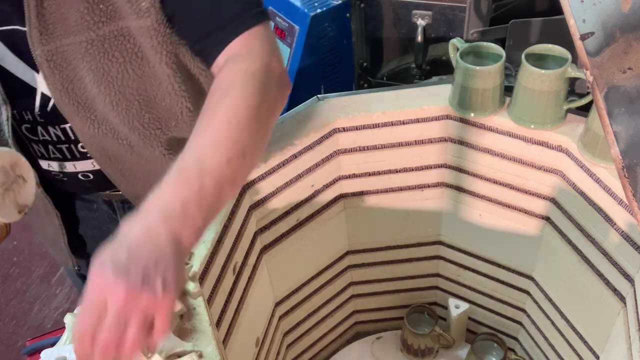 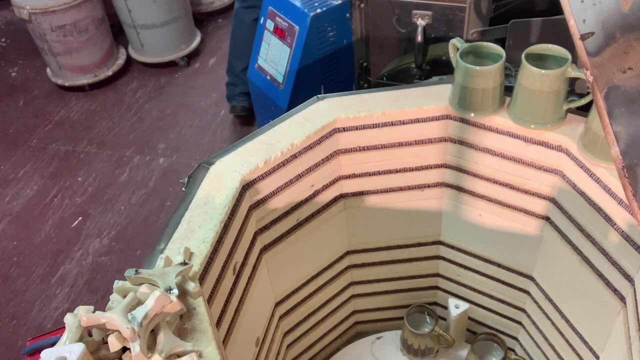 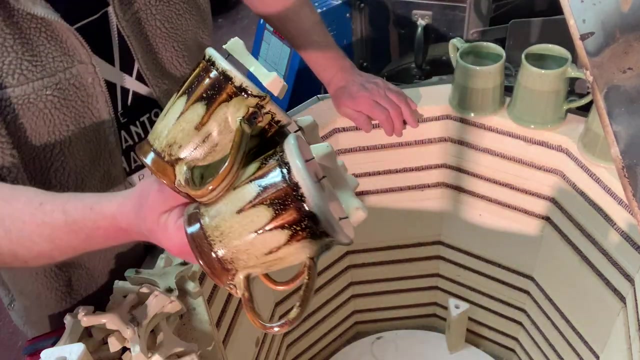 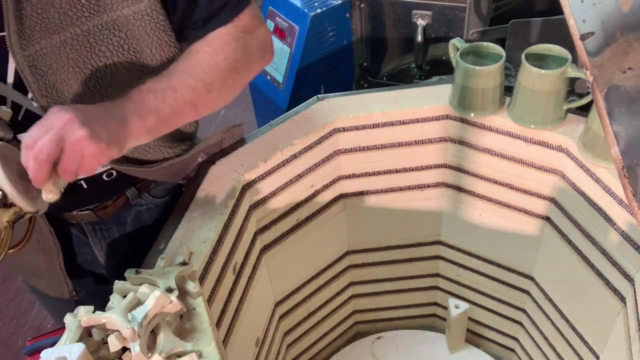 Now time to do this. Look at that. It's the same on every piece. Just perfect. I just have to grind that one a little bit. There's a little bit of glaze there And there's another three, So this behaved perfectly in this firing schedule. 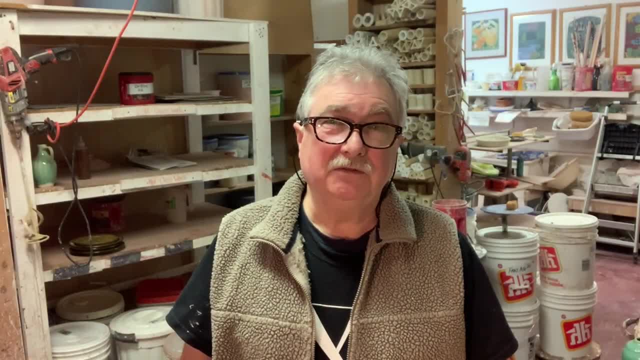 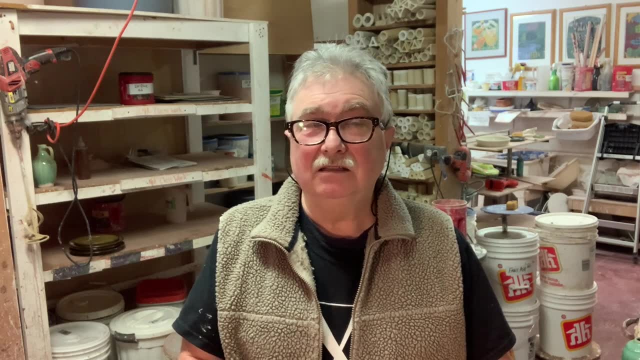 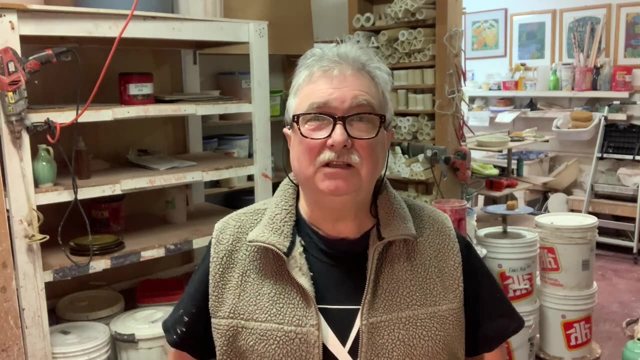 This is a long video, probably an hour, but a lot of information in here. Press subscribe. I have lots of videos now on YouTube and thumbs up whatever. I don't know what that does. I'm not monetizing this channel because I'm fine. I don't need to do that. 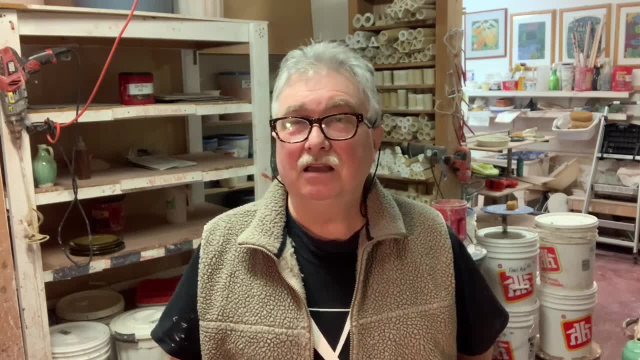 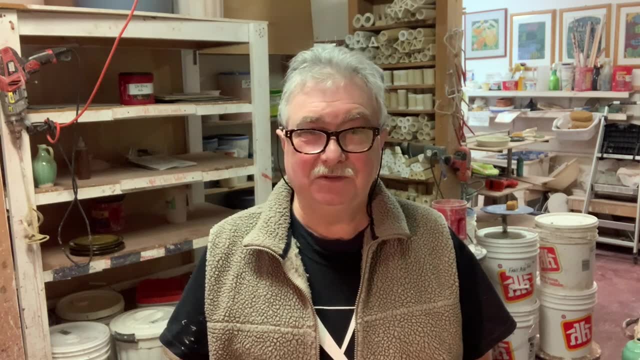 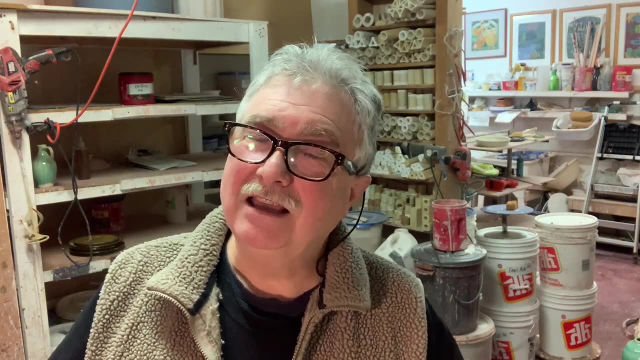 So basically, this is supposed to be for educational purposes and I hope that everybody has lots of fun playing with pottery. I mean, what a time to be doing pottery anyway, we're so lucky we have it. Anyway, this is Vaughan Smith in Westcotebeltpotteryca in Nova Scotia, Canada.